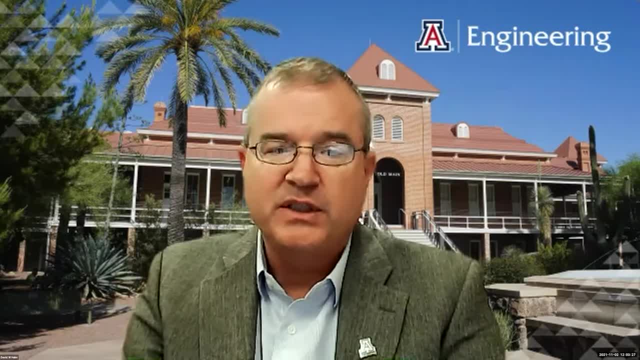 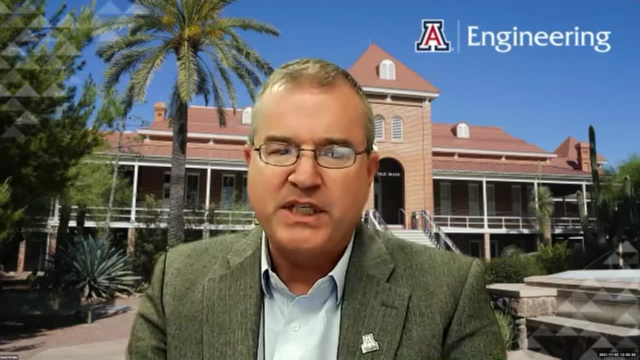 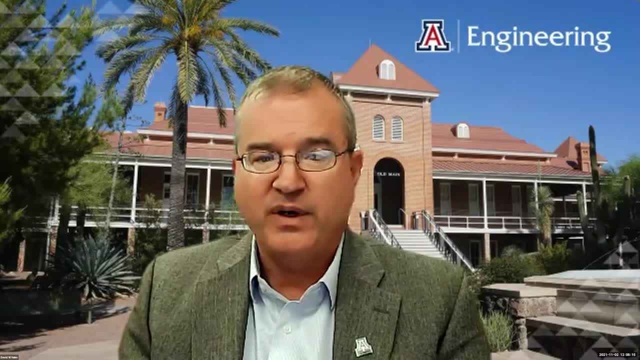 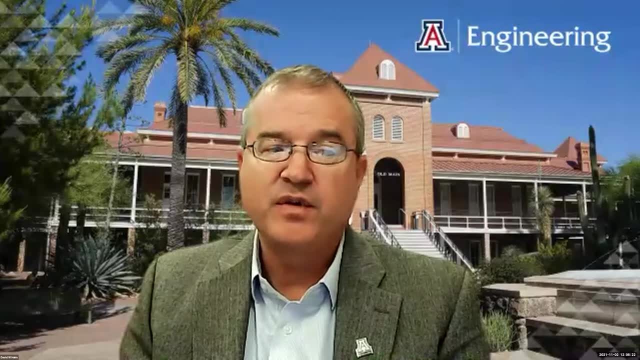 With novel health sensors, the monitoring of pathogens and biological molecules. John Yiel was the president of the institute who created Biochemistry and biochemistry. John Yiel was the president of the Institute of Biological Engineering in 2015.. He currently serves as Editor in Chief for the Journal of Biological Engineering, associate editor for biosensors and bioelectronics. 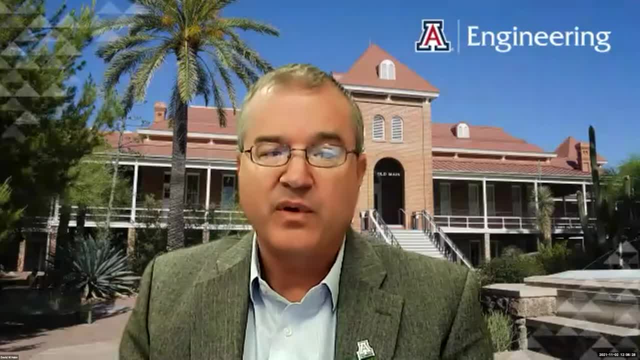 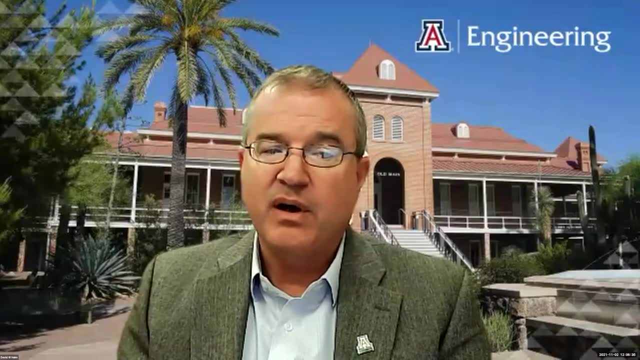 and he is on the editorial board for Scientific Reports and several other journals. He has authored 2 textbooks on biosensors published by Springer and Elsevier, and the third book on tissue engineering is in the works. Dr Yoon's research includes work on biosensing and than. he also published two issues on biological biology and biochemistry in the Chicago Public Library. 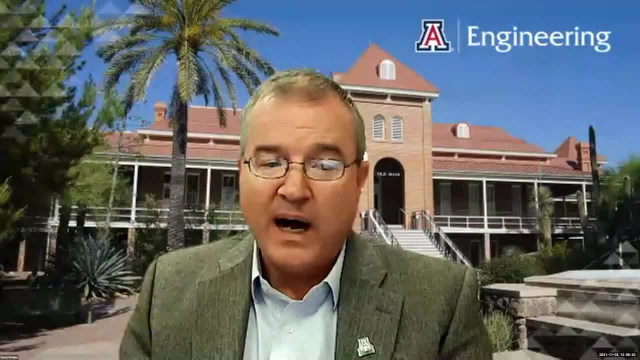 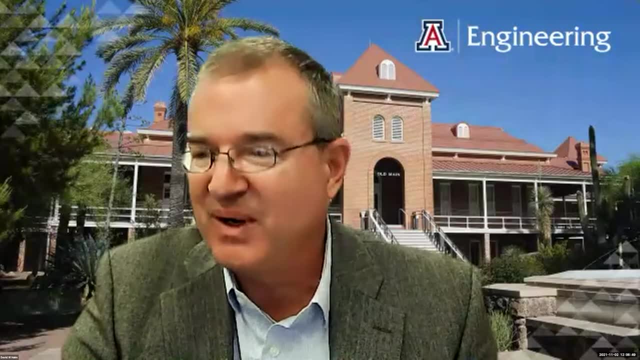 research includes work on biosensors, and he is widely recognized for his contributions to smartphone-based biosensors and medical diagnostics. Welcome Judith, Welcome Jung-Yul, We're glad you're here. Before we get into your presentation, your formal presentation: 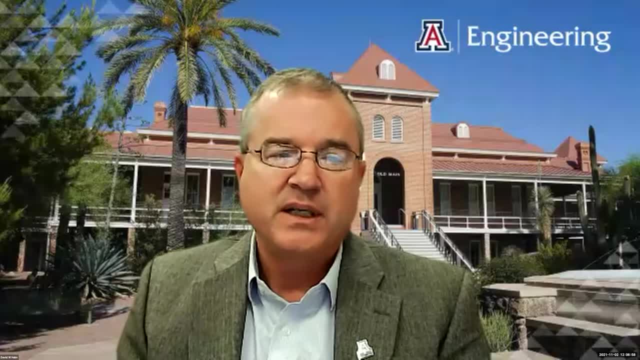 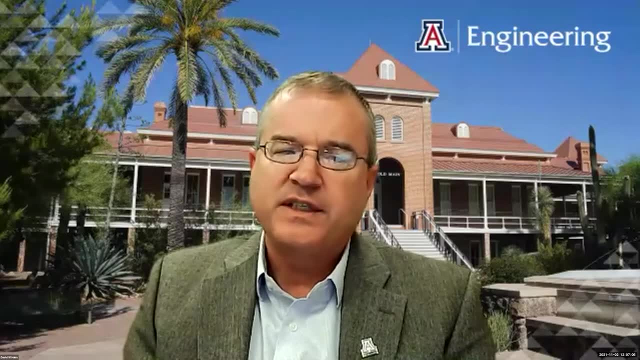 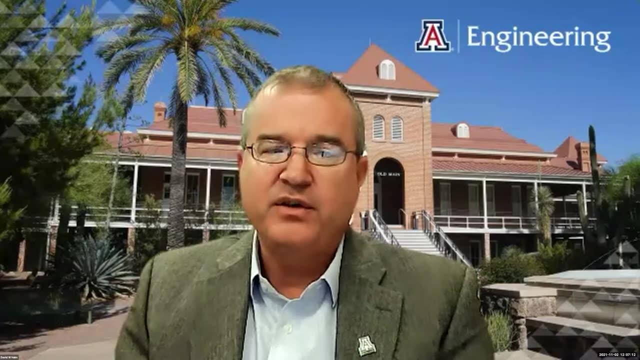 to set the stage. let's start with kind of a big-picture question, You know, looking at our educational mission. how might institutions such as ours keep pace and prepare students for work and advanced health care devices sensing beyond their university days, including supporting local? 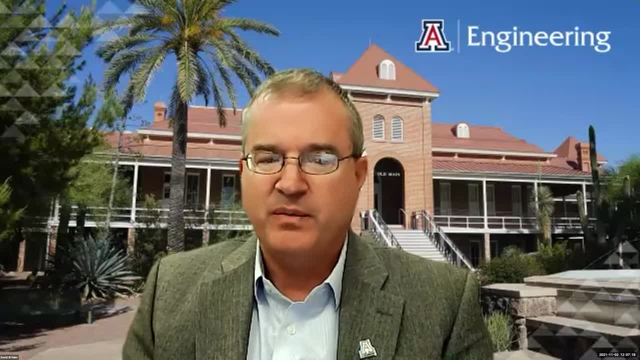 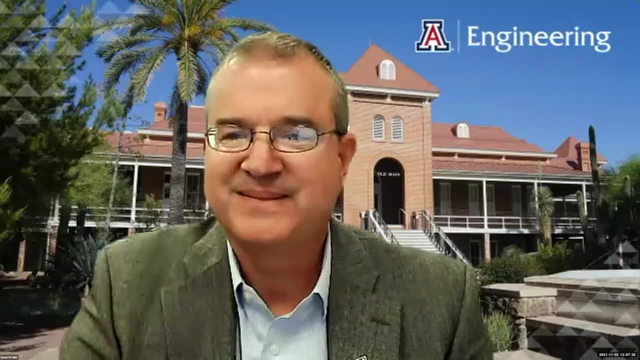 government or commercial ventures, And I do know that Tucson is home to many optics-based startup companies, So I'll go to you, Judith, and then to Jung-Yul. Well, thanks for the introduction, So I think that's a really great question. I think you know when you 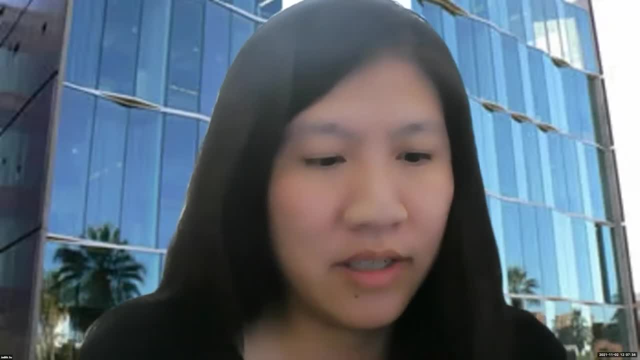 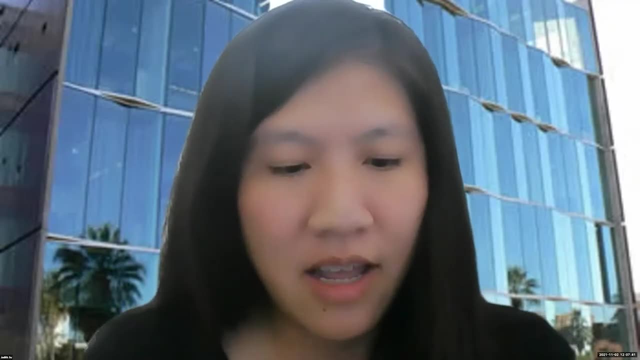 have a world with rapidly changing technology, I think it's important to you know educate students with a solid base of fundamentals such that they can, you know, specialize rapidly without being specialists, And I know that you had mentioned that Tucson was home to a lot of. 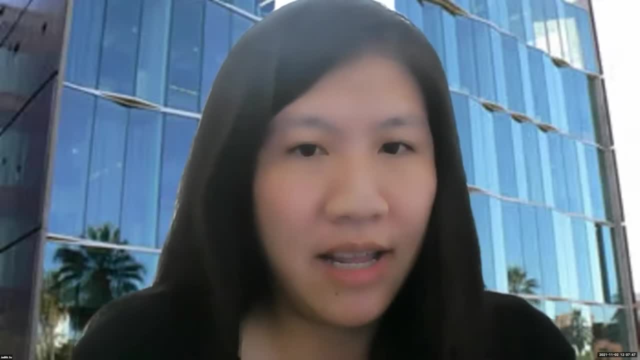 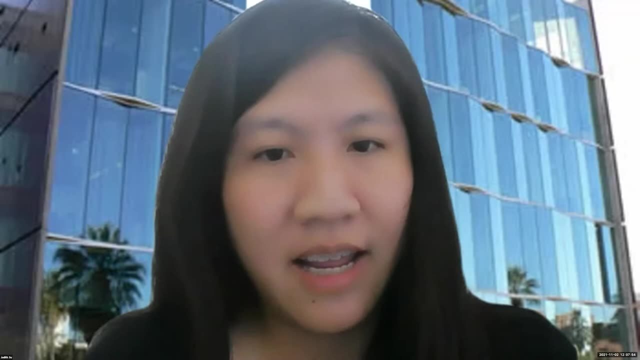 optics companies, many of which were founded by U of A alums themselves. So I think it's also important to connect with alumni such as, you know, the people attending today, you know, for the opportunities and knowledge that you can provide. 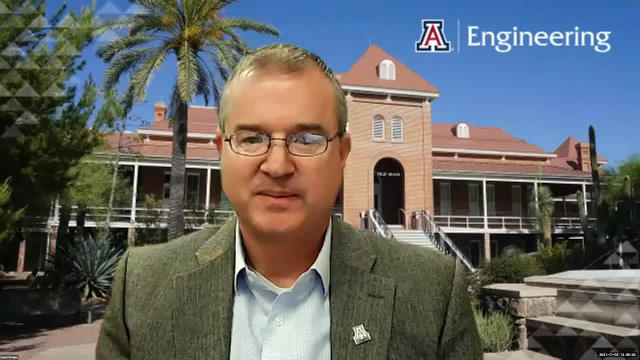 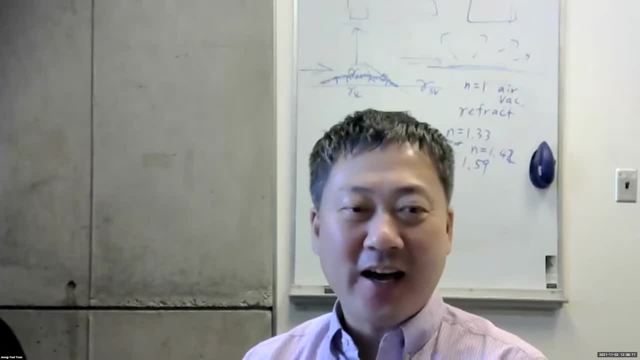 Excellent, Jung-Yul, you're muted. Yep, Sorry about that. So in my personal opinion, I think it's really important to utilize our senior design projects to connect our undergraduate students to work with the industry people out there, So that's going to be a really great opportunity for our students to get better. 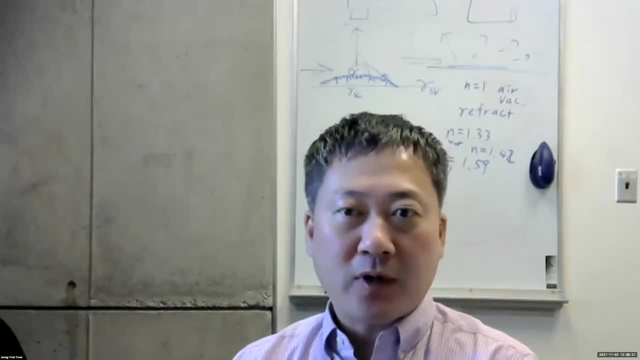 prepared, But at the same time faculty members also work really hard to connect with our senior design out there and industry people out there to establish collaboration and then potential investment in research projects. Or maybe we can jointly ask for federal funding And so we can actually work together as a team and then get our undergraduate and graduate 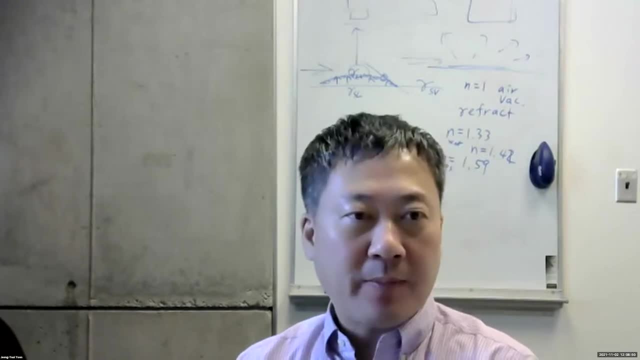 students involved in those projects to get better prepared for their future career, And so that's translation and commercialization, And they also we need to educate them on to stop. That's a great point, And I think it's also important for us to be able to get them to. 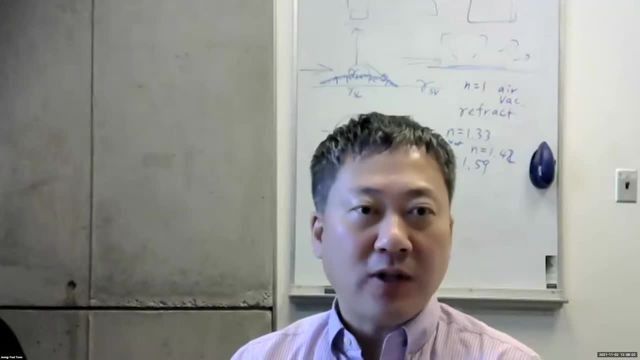 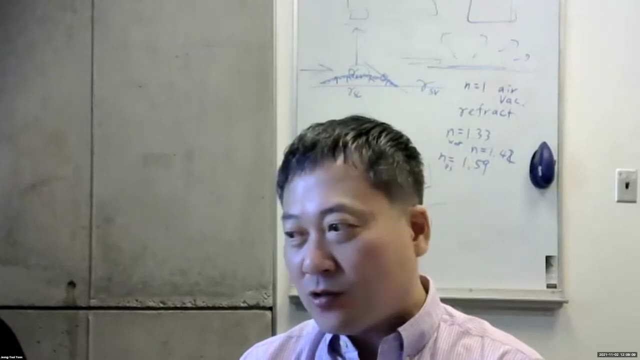 participate and learn from each other at the same time in the future and to connect with them, educate them how they can be, how they can under the students actually have a limited understanding about how industry works, like how we can recruit the um, the people, how we can gain investment. 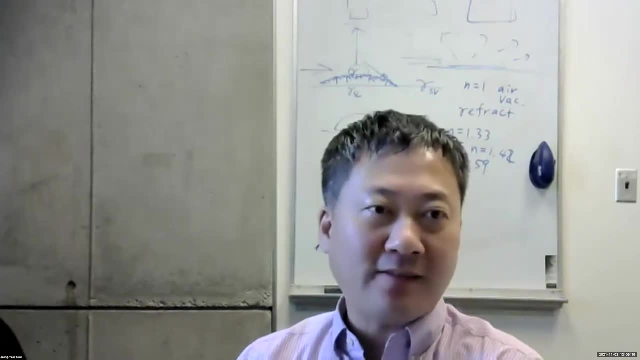 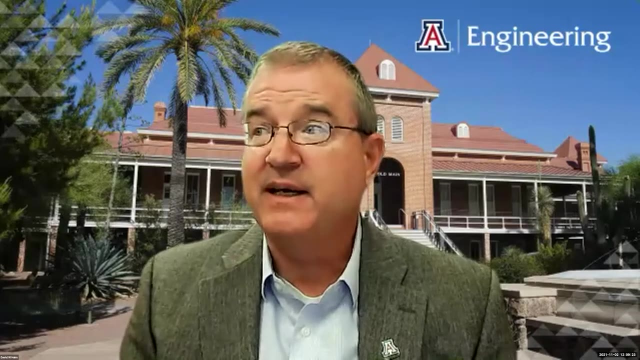 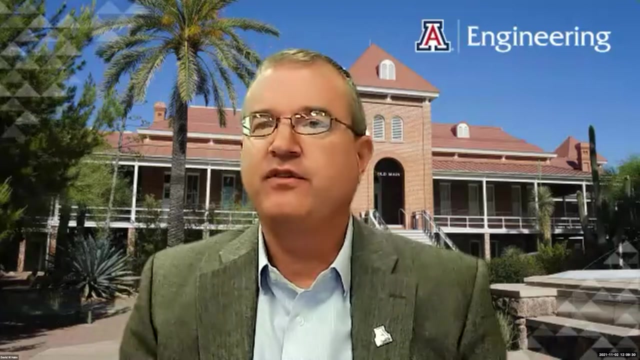 funding and so on. so the entrepreneurship type classes is also important for many engineering students outstanding. we certainly have two outstanding ambassadors to the community in both of you. so i appreciate your answers and your thoughtfulness of of willingness to engage the greater tucson uh community and see that trends technology is transferred nicely so. 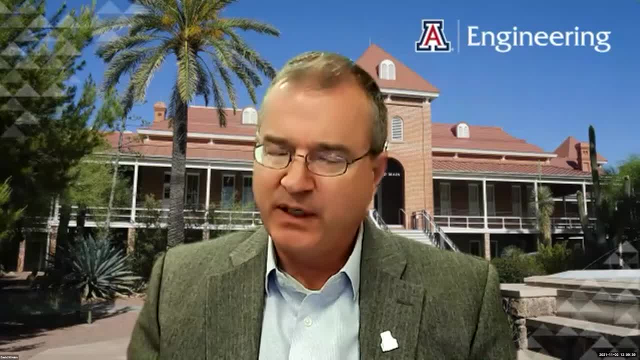 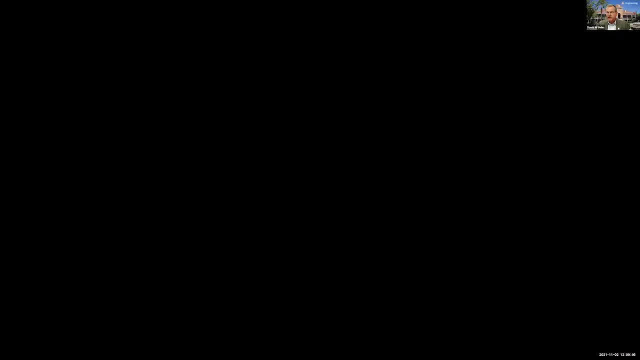 we're going to do now is have you each give a uh, a short presentation to kind of set the stage for our q? a. so we're going to start with you, judith, and then uh, when you're done your lunch here, and go to jung yul. so, judith, take it away. that's a great, great pleasure that i'm here today to share. 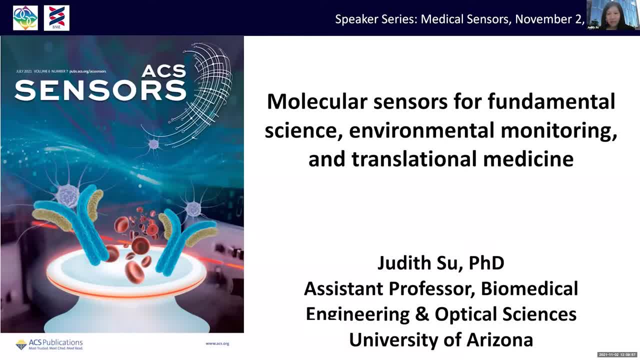 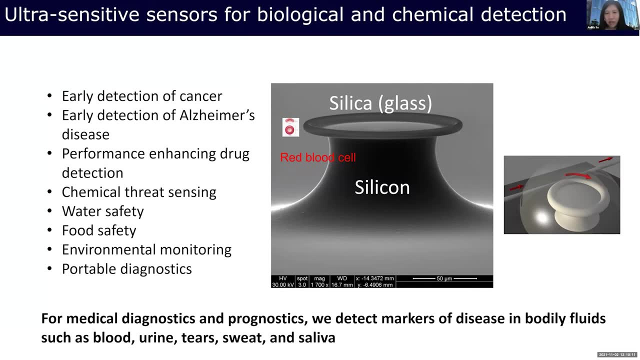 with you guys the world that I'm doing in my lab. So our lab specializes in developing ultra-sensitive sensors for a wide variety of applications, but one of our main application areas is medical diagnostics. So, as I just mentioned, our lab specializes in developing ultra-sensitive sensors, and so the 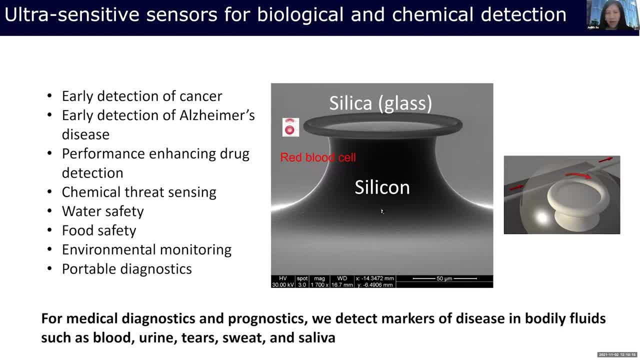 sensor platform that we used is shown in this picture on the right. It's called the microtorid optical resonator. It's essentially a glass donut. It's about the width of a human hair, and I've put this red blood cell next to it so that you can get a size comparison. 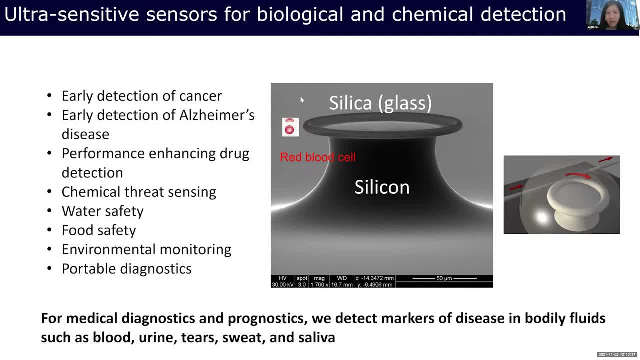 And essentially what we do for our medical diagnostic applications is we detect biomarkers of diseases in any sort of bodily fluids like blood, urine, sweat tears, basically anything that sort of contains a biomarker for disease, And we have a lot of applications in our lab. I'm just 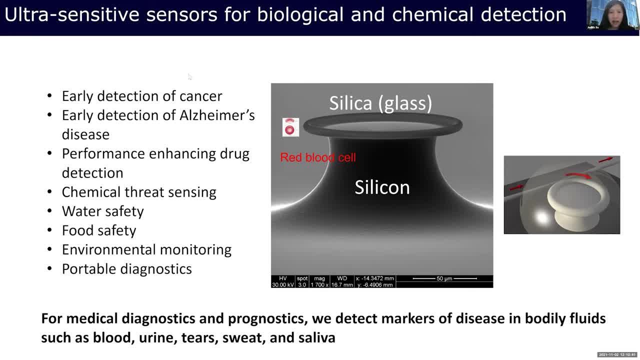 going to go through a couple of them. So one of our main application areas is early detection of cancer. We also work on early detection of Alzheimer's disease. We just finished a project a few years ago on performance enhancing drug detection. We have a large project with the. 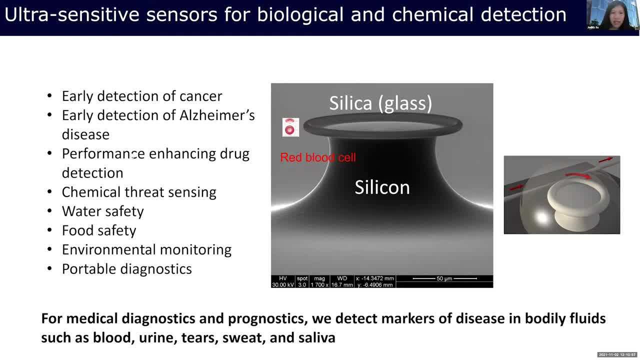 Department of the Pharma and Biomedical Services. We have a large project with the Department of the Pharma and Biomedical Services. We have a large project with the Department of the Pharma and defense on chemical threat sensing. We look at things like water safety, food safety. 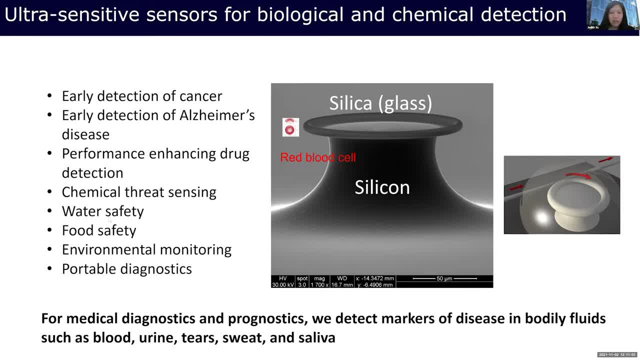 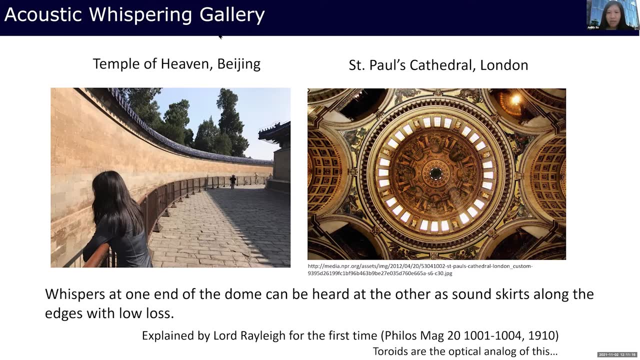 environmental monitoring, and then a large portion of my lab focuses on further improving our sensing platform, for example by making portable sensors more robust sensors. So our sensors are called optical whispering gallery mode resonators. They're named after the acoustic whispering gallery phenomena, and perhaps the most famous example of this is St 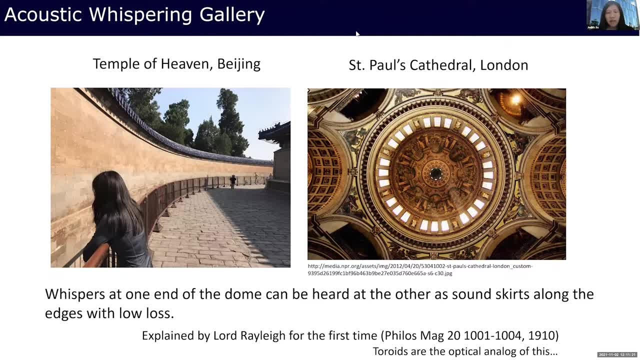 Paul's Cathedral in London. So in St Paul's Cathedral in London, underneath the dome there is a gallery known as the whispering gallery, and if you stand at one end and you whisper in the gallery, your friend can hear you 40 meters away at the other end because sound. 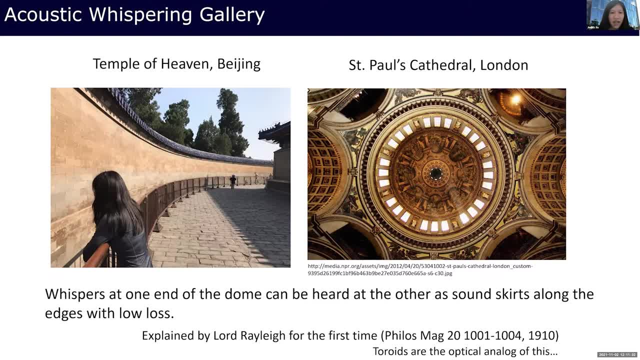 travels along the edges of the wall of the gallery with negligible loss. So here's a on the picture on the left. here's an example I like to use because you can really see this curved wall. So this is called the echo wall. It's in the Temple of Heaven in Beijing. I'm in the front and my 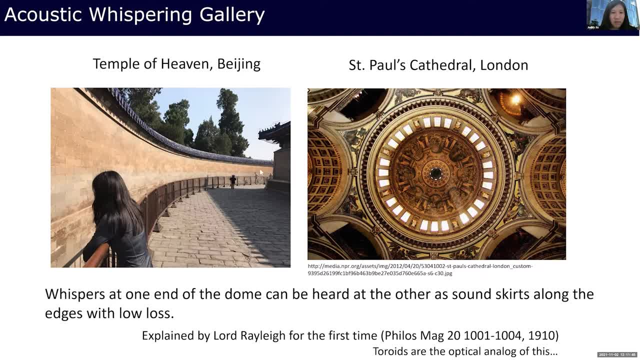 husband's in the back, and he can hear what I'm saying even though we're far apart, because sound is traveling along the edges of this wall, And so our sensors operate on the same principle, which is that we can hear what we're saying even though we're far apart. 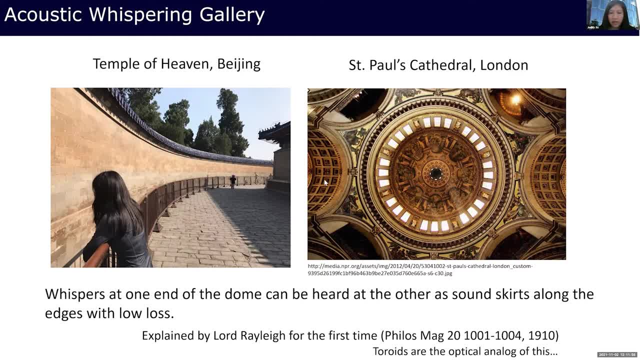 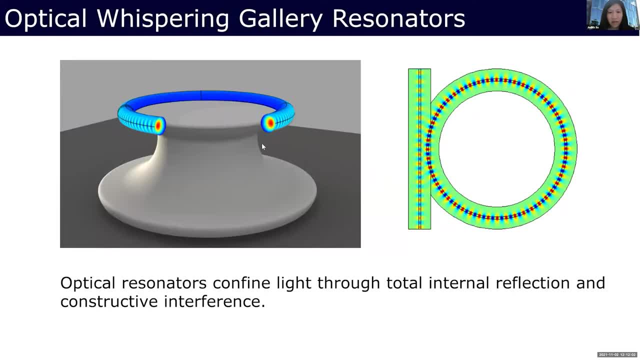 And so our sensors operate on the same principle, except, instead of sound traveling along the edges of a wall or some architectural feature, we use light that's traveling around the edges of this sort of glass donut toward the optical analog of the acoustic whispering gallery. And so here's an. 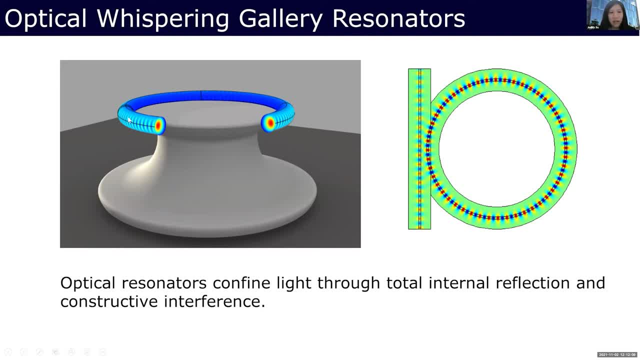 artistic rendering of what our sensor looks like. The bright colors represent the light within the device, And so you can see the light is traveling along the rim of the device and it travels via the principle of total internal reflection. So you can see this is sort of similar to how light 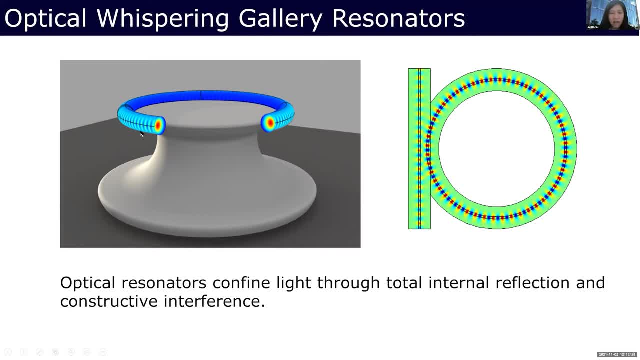 travels along the edge of a wall, And so you can see the light is traveling along the rim of the device, and it travels through an optical fiber. But you can think of this as sort of an optical fiber that's sort of bent back upon itself, And so the light is continuously trapped in this ring. 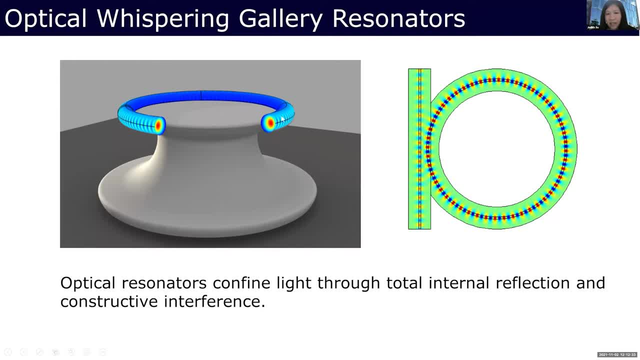 essentially, The light is not perfectly confined in the ring. Some of the light extends a little bit outward, beyond the periphery of the ring, And this is what gives our device such high sensitivity. So what we do is this is made of glass, and so we can functionalize this with capture agents for 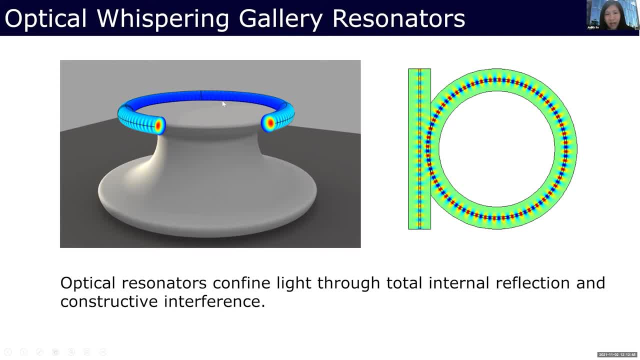 various different biomarkers, for example, like antibodies, And when things bind to the surface, the light continuously goes around, And so we can see that the light is trapped in this ring. So we can visualize the dyeing of the light wherever we cold coloring, we turn the light around it. 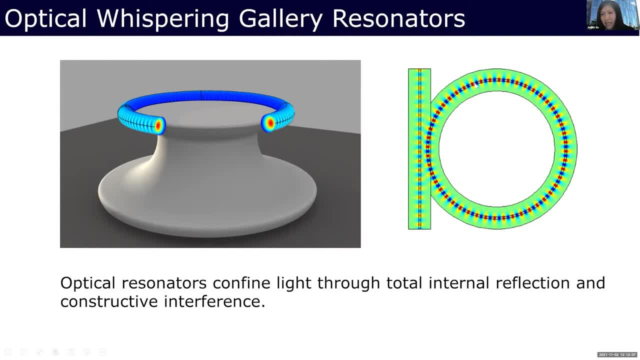 interacts with it, so constantly re interrogates or sample, And this is what generates a very high signal for us, And you can see a little gif of this on the right. So this sort of vertical rectangle represents a waveguide, which is what we use to couple light into our sensors, And then you can 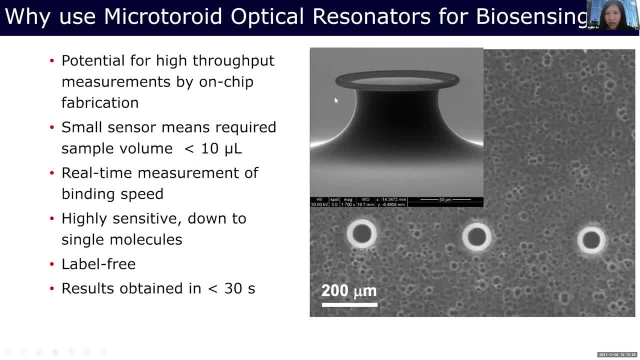 see this constructive amplification of light within this device, And this happens at a particular, you know on the right, in the upper left-hand corner of this image, And then the bottom circles are the sort of the top view, And so you can imagine that we could coat each one of these. 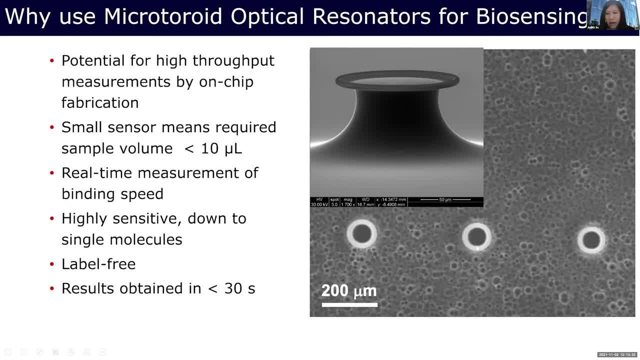 sensors with a different capture agent, so that we could look at different biomarkers, And so we could eventually examine panels of biomarkers. And so our sensors have a number of advantages. One is that you have the potential for very high throughput measurements because you have 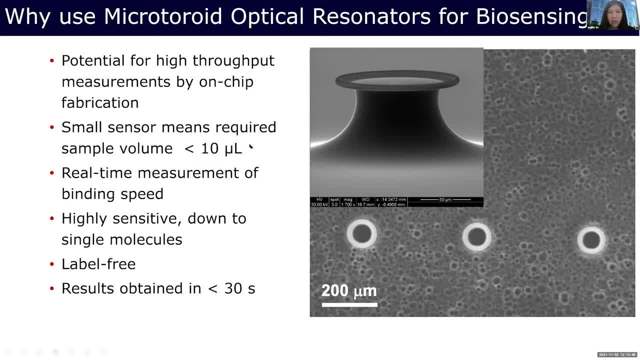 on-chip fabrication, So we can make hundreds of these devices. We have a very, very small sensor, which means that a very, very small sample volume is required, So less than 10 microliters, which is about a drop. So we just completed a study on ovarian cancer which we were able to. 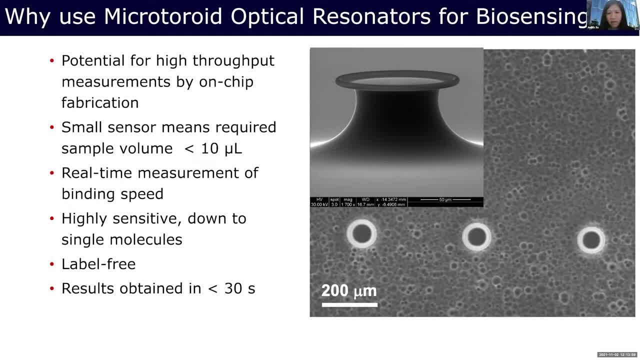 track tumor progression. using just four microliters of a very small vaginal lavage sample from a mouse, We can get real-time measurements of binding speed. We're very sensitive. We're down to single molecules, So we're label-free, which means that we don't have to put any sort of 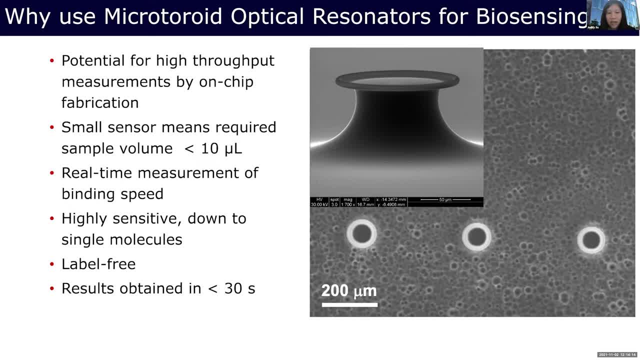 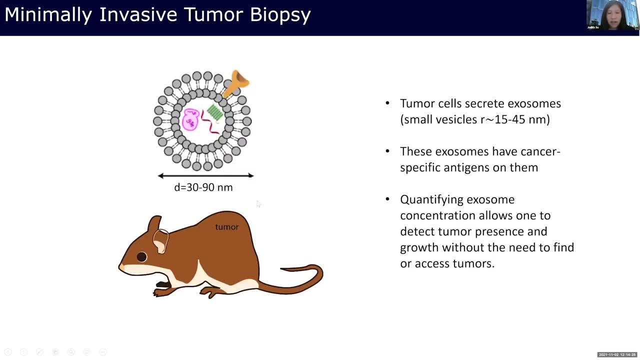 radioactive tags or fluorescent labels on what we're trying to sense, And we could obtain results in under 30 seconds, which is very important. for some of our applications, such as infectious disease detection, It's very, very important to be able to get timely detection, And so this is one of our first applications that we did. 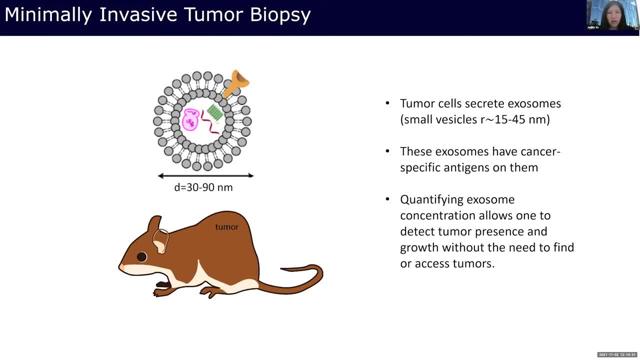 which was on a minimally invasive tumor biopsy, And so what we did is that we implanted mice with human Burkitt's lymphoma tumor cells. So this cell line was picked because it's a very aggressive tumor, And so we were looking at this particular biomarker called exosomes. So exosomes- 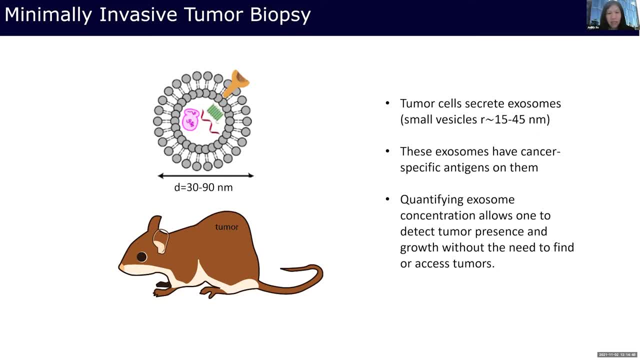 you can think of it as little bits of the earth, the membrane of your cell, And what's exciting about exosomes is that when you have little bits of the membrane of a tumor cell, it carries little bits of your tumor inside your bloodstream, And so the idea. 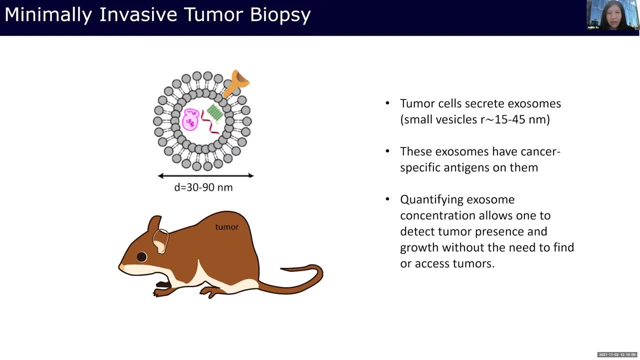 is that you can exploit the circulation of blood to detect if a tumor is present and how far it's progressed, without having to do surgical intervention, without having the need to find or access a tumor and do a biopsy, And so this is really good, because people are very often 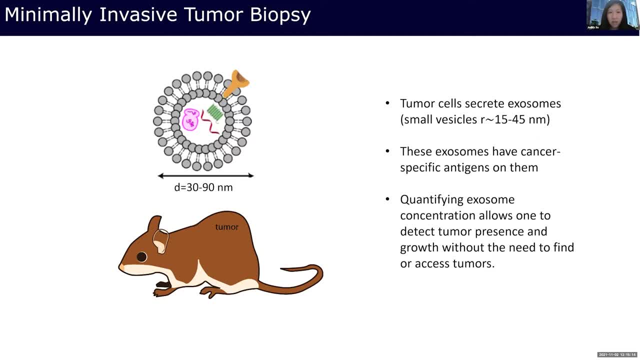 they're interested in. they're willing to, for example, be biopsied once so that they can find out what they have, but they're more reluctant to be biopsied multiple times, And so this is a good way if you can get something. 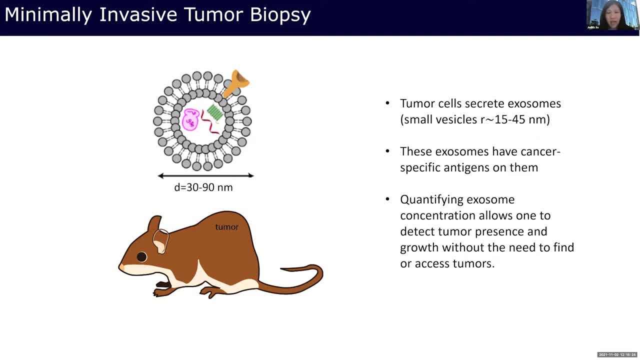 like this to work, where you can track tumor progression. you can also look at- you know- treatment outcomes, for example. So how do different treatments affect different biomarker levels? And so the way to interpret this graph as you can see, so the y-axis or the vertical. 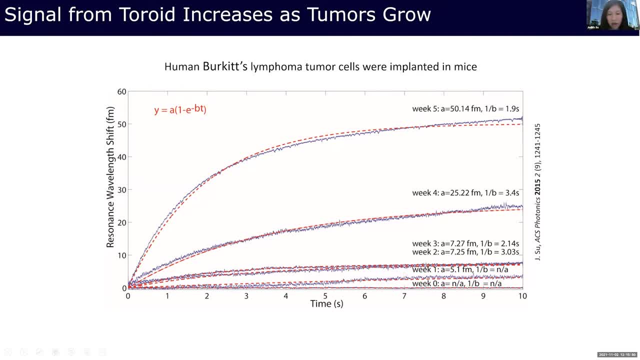 axis. here is the signal from our sensor. So you can see, from week zero we don't see much signal from our sensor, but then as each week progresses you can see larger and larger signal from our sensor as more of these exosome biomarkers are binding to the surface of our 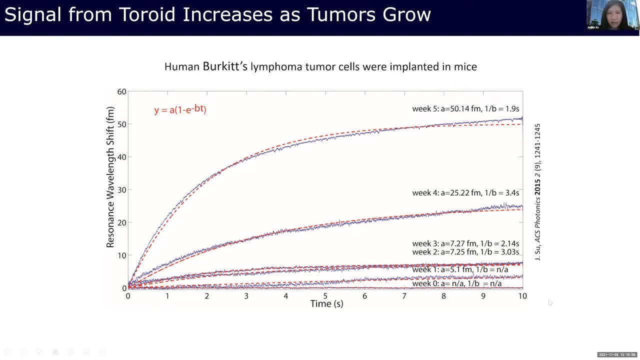 device And then the control experiment, for that, of course, is a mouse with no tumor. So we took a mouse with no tumor and then we looked at the signal from our sensor from week one and week five and we didn't see this similar increase in signal. And so where's the future of this going? 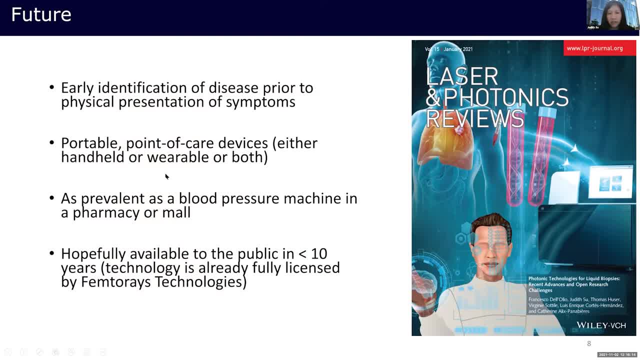 So our goal is early identification of disease prior to physical presentation of symptoms. So we want to avoid a situation where you know you go to the doctor because you're starting to feel like in extreme pain and then you're being told that you know you have stage four cancer and you only have six months to live. 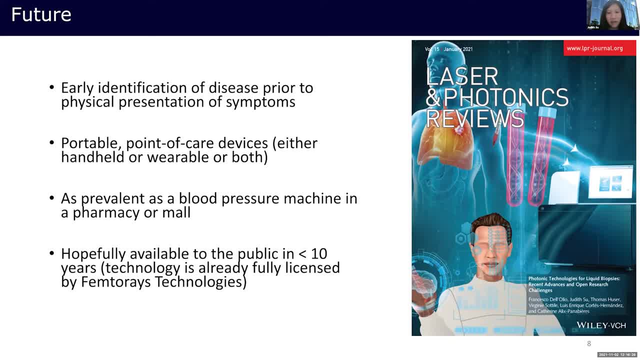 something like that. Because we have a very, very sensitive sensor, we can detect very, very low quantities of these biomarkers. So we're interested in making these devices portable point-of-care devices, either handheld, wearable or both. We're interested in making this as. 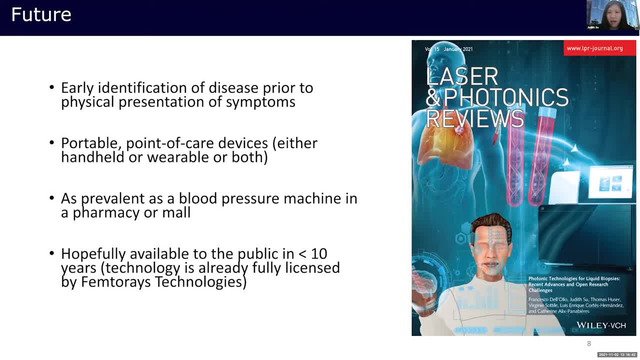 prevalent as a blood pressure machine in a pharmacy or mall. Our, you know, time to getting this into the hands of the public is hopefully in less than 10 years. our technology is already fully licensed by a company called FemtoRace Technologies, which is a startup company. 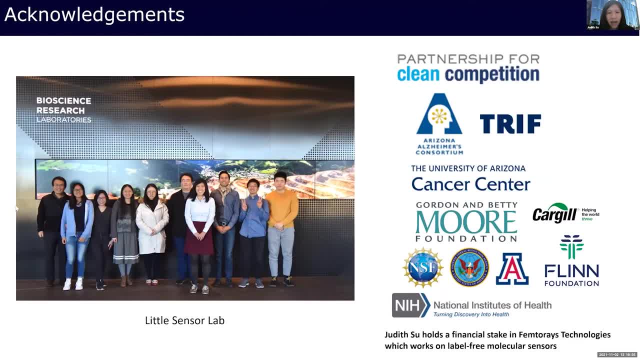 based in Italy, And I would like to thank our lab and all of our sources of funding, And I'm happy to answer any questions that people may have. Thank you very much, Judith. Before we jump to Jonggyu, let me just ask one point of clarification that someone just posted On your mouse model. 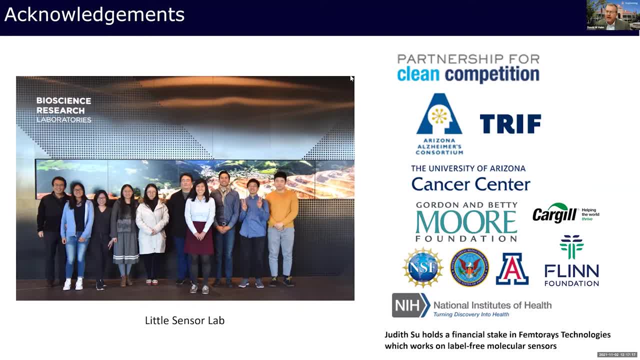 experiment. you're not putting your sensing device in the mouse, you're drawing the blood sample and bringing it to your device. Is that correct? Yes, it's absolutely correct. So we're. currently we are not an in vitro sensor, So we're, you know. 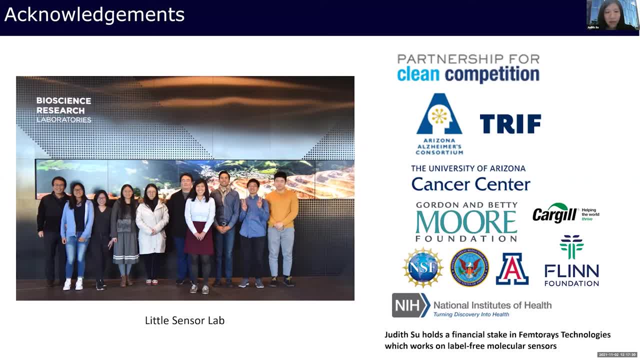 we're, we're outside- sorry, we're not in vivo sensor, we're outside in the laboratory And then we just flow any sort of biomarker containing solution over our devices. Got it. Thank you for that quick clarification, Excellent. If you unshare your screen, we'll turn. 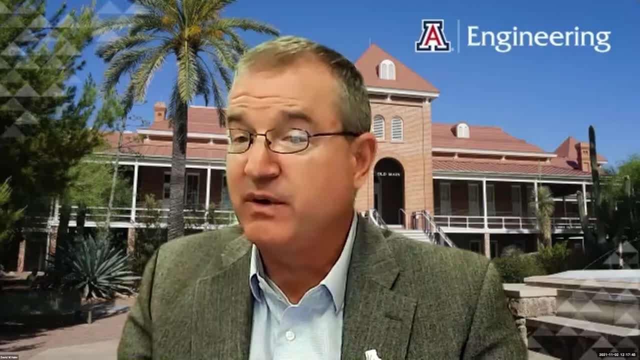 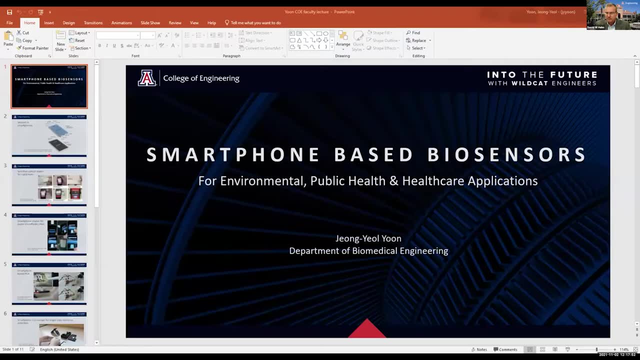 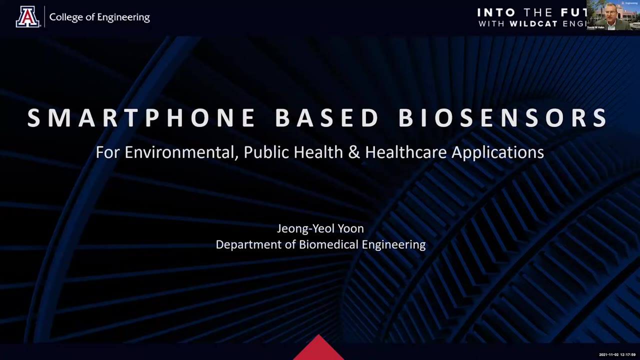 over to Jonggyu to share his screen and give us a presentation on some of his exciting biosensing work. Over to you, Jonggyu. Thank you, Can you see my screen? Okay, Perfect, Sounds good. So, hello, my name is Jonggyu Yoon from Department of Biomedical Engineering, So I 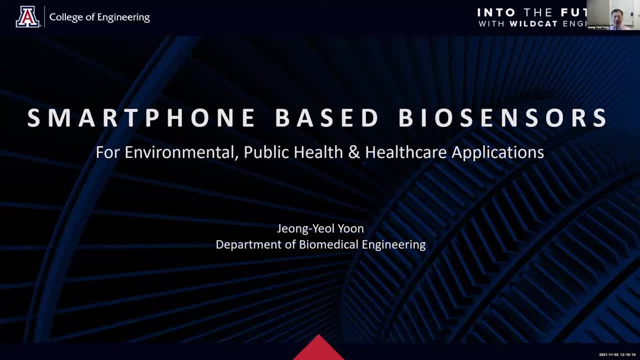 have been known as a smartphone biosensor guy in scientific community. So that's the topic I'm going to talk about today, And actually this can be used for the medical healthcare applications, but equally can be used for environmental and public health applications as well. So my background was microfluidics and 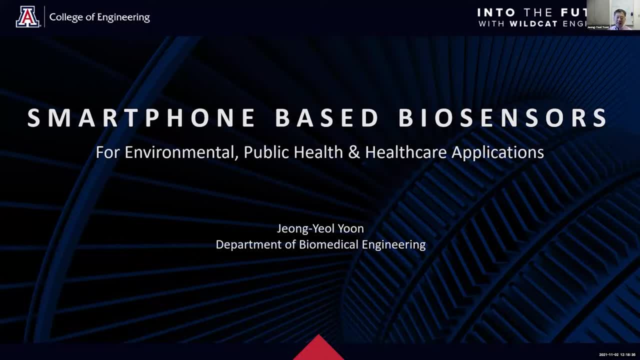 biosensor when I did my PhD study at UCLA And I came to U of A in 2004 and continued working on this, And then it's primarily optics-based microfluidic sensor And again 07i has worked since 2006.. Now the 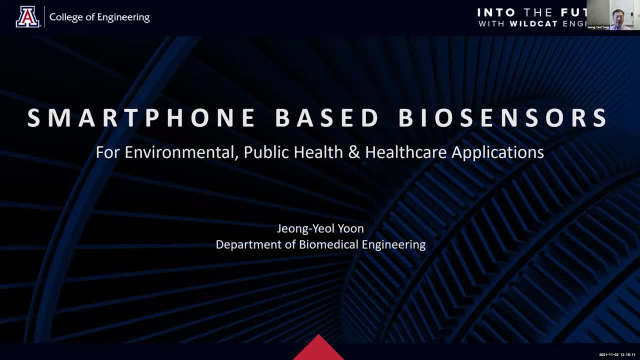 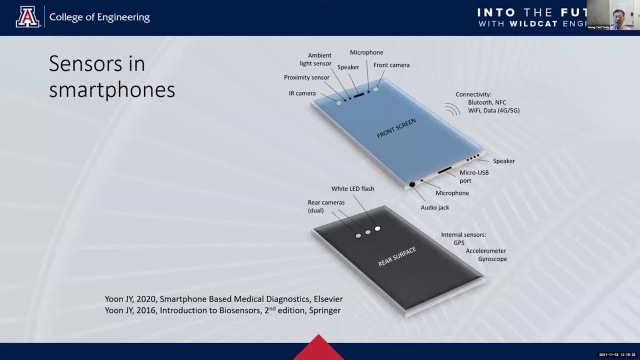 Sar funktion pour mor prend de Réannest함. the sensors: there are many sensors already incorporated in the smartphone. So here's the next slide. We have the front and rear camera, IR camera, proximity sensor and GPS accelerometer, gyroscope. the light source: white LED flash, and then it has a 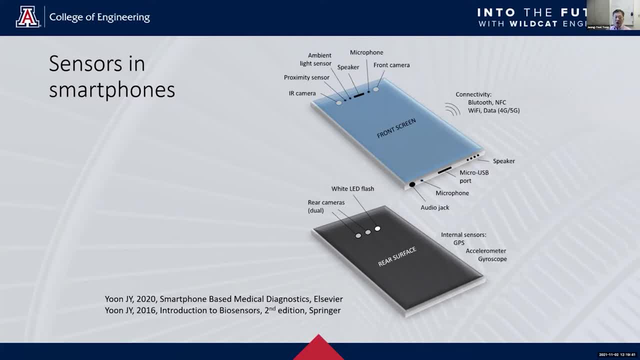 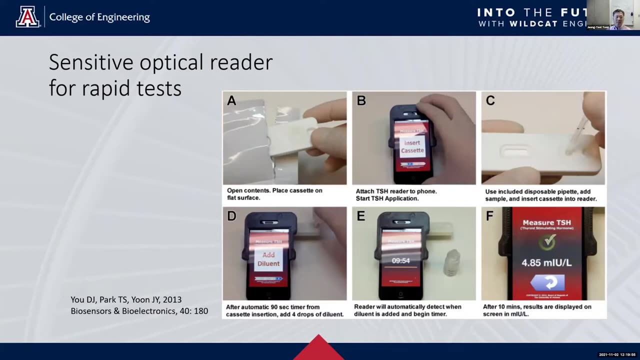 computing power and they send your data through Bluetooth, NFC, Wi-Fi, 4G, 5G network. So can you utilize this? So the first project that I walked in collaboration with industry was create an optical reader device based on your smartphone. So this is the. 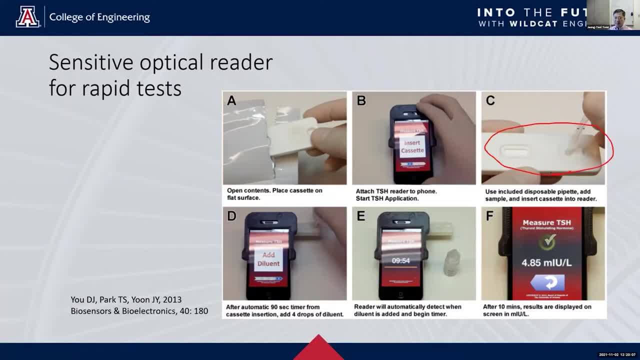 ladder flow assay, also known as the rapid kits, And if you do not know what they are, think about pregnancy test Or, more importantly, the COVID-19 rapid antigen test. If you do not know what they are, think about: pregnancy test Or, more importantly, the COVID-19 rapid antigen test. 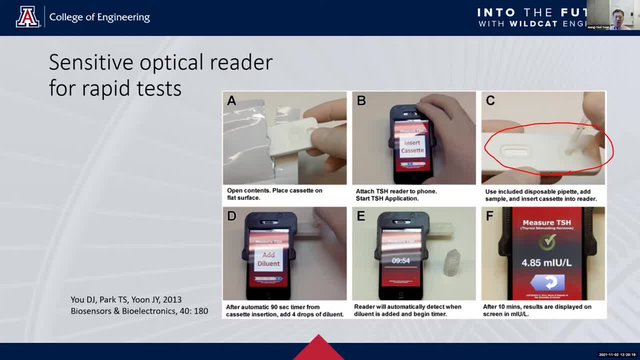 It's all based on antibody. So you're just going to take up your blood or saliva sample, add it, and then the band will develop, And so you can check the positive or negative with your naked eye, but you can actually insert it into the optical reader device to quantify the concentration. 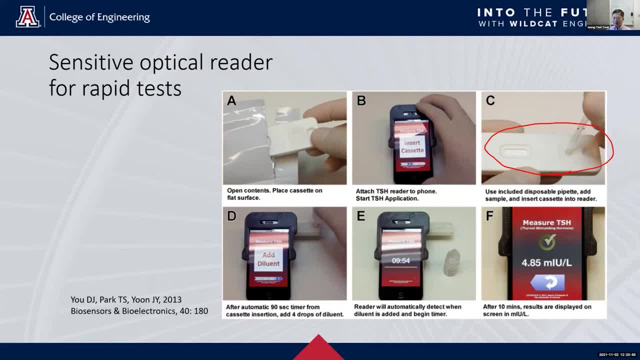 And then that device tends to be rather expensive. So what I did? I replaced that optical reader device. Typically it costs around $20,000 to $50,000 using your smartphone. So in that case I made the optical reader device printed with the 3D printer And then we did a lot of optimization. So this is primarily 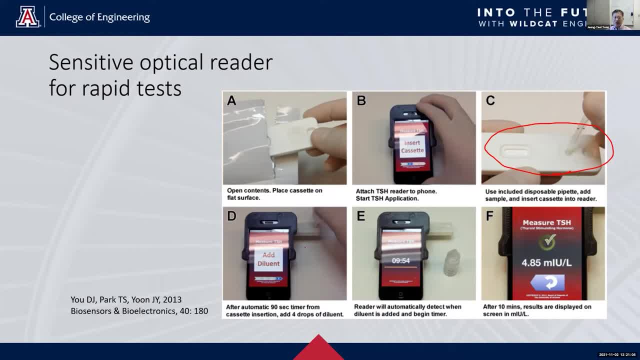 angled detection. We are measuring at a certain distance and angle to maximize the assay. And then we coded our own app. And then we demonstrated one order of magnitude better limit of detection in comparison to the stand-alone laboratory optical reader device. So we got a lot of media. 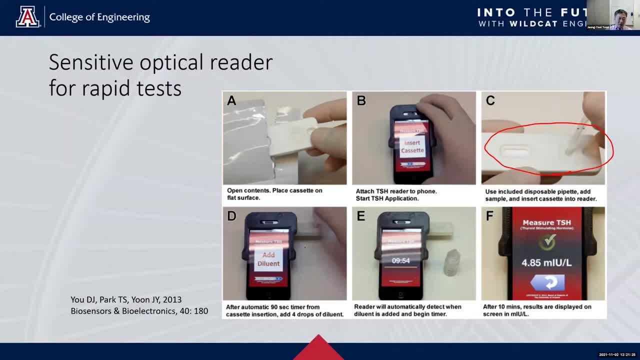 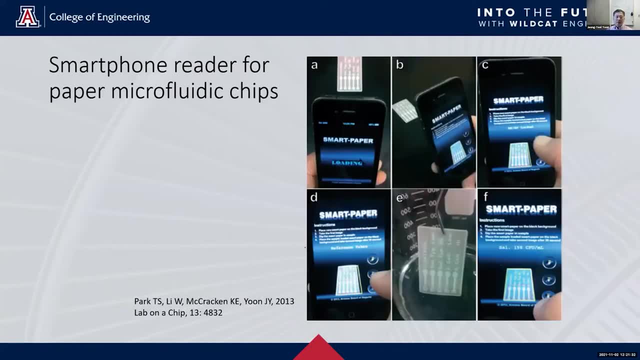 attention in that year And then we actually moved on to a different application. So if you can do that on the commercial rapid kits, can you do that on paper microfluidic chips, Whereas the microfluidic channels are being printed on your paper And we can. 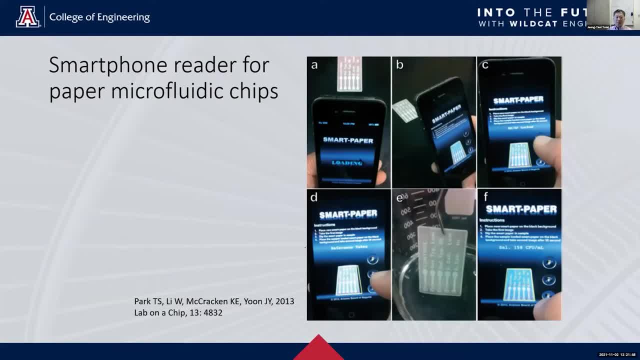 do multiple assays in a more complex manner, but this time we are measuring our signal at an optimized angle and distance using the smartphone's gyroscope and the accelerometer. So it worked quite well and we called it as a smart paper app And we got a publication in 2013 as well. 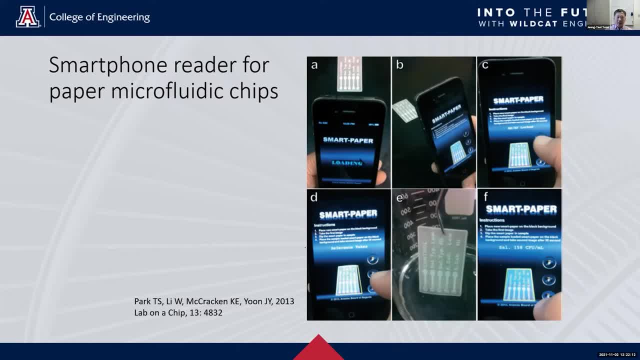 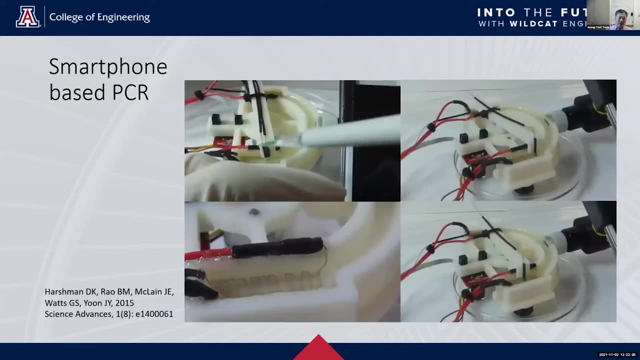 So these are all based on antibody assay And if you got the positive signal with this antibody assay, then you may want to test it for this genetic sequence known as the PCR or polymerase chain reaction. And of course, PCR requires the loss of apparatus, trained personnel, and then it usually takes up four days And we actually 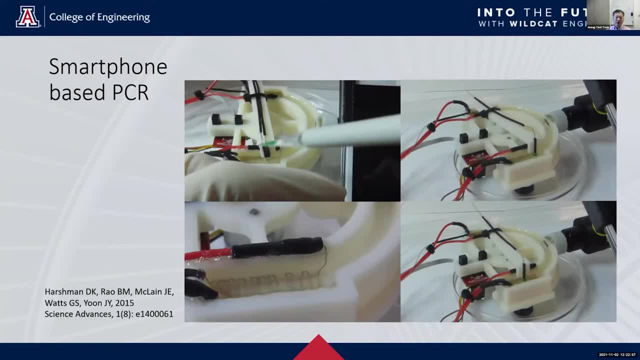 created the PCR device that can be run in a small form factor and then coupled with the smartphone optical reader. We made a lot of innovations on this device so we can finish our assay From sample to answer. it took about 20 minutes, And then thermal cycling itself takes about three. 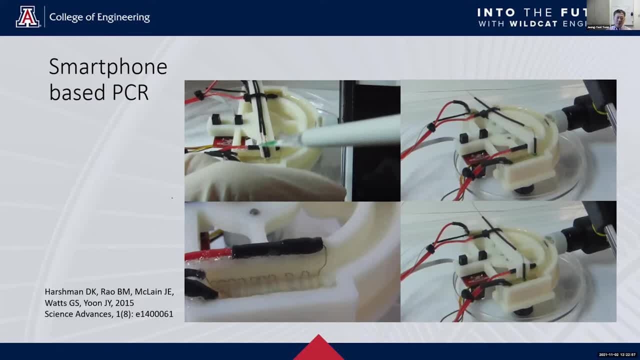 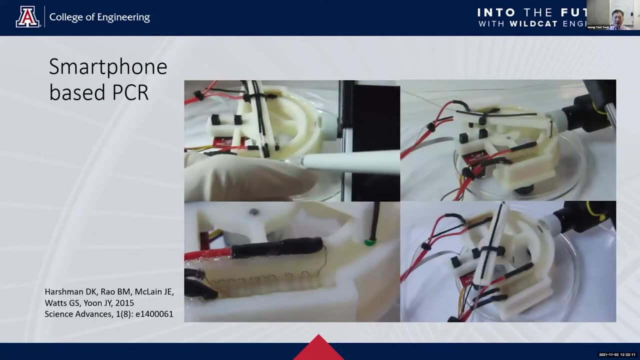 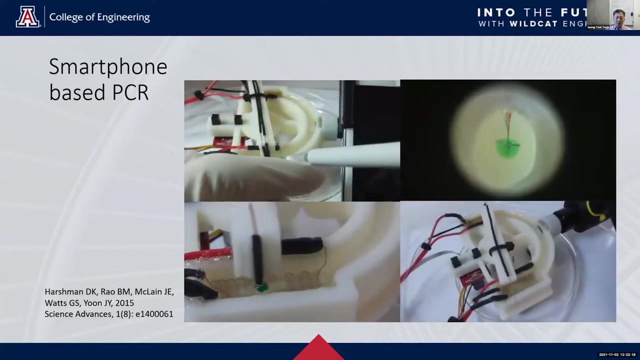 minutes compared to several hours in the laboratory, So I'm going to share the screen. So this is how our device works And you can clearly see that all those detections are being made by this marker. So we made an equal contribution to the PCR assay as well. 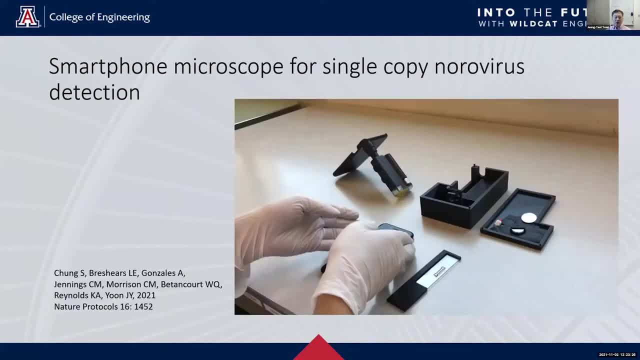 So once we have demonstrated that, then we wanted to push our limit. Maybe can I detect the target molecule, in this case norovirus, down to a single copy level, So this is almost like a molecular level detection, And to make it happen I needed fluorescence. 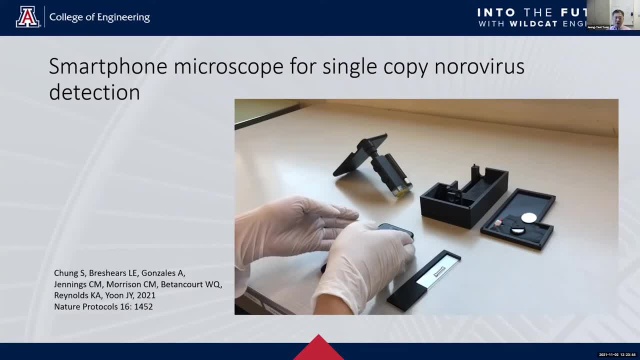 microscope, So Benchtop, really expensive microscope, So we can count those individual virus particles one by one, And then can you do that with the smartphone. And what he did is using the off-the-shelf components and assemble the water together And then we can create the smartphone fluorescence microscope. 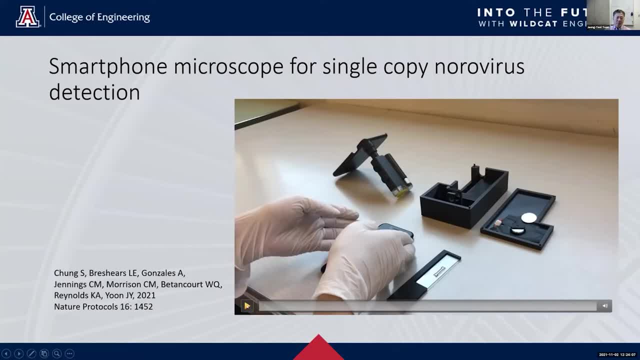 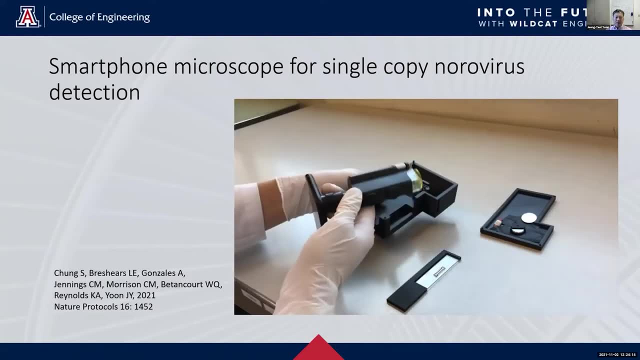 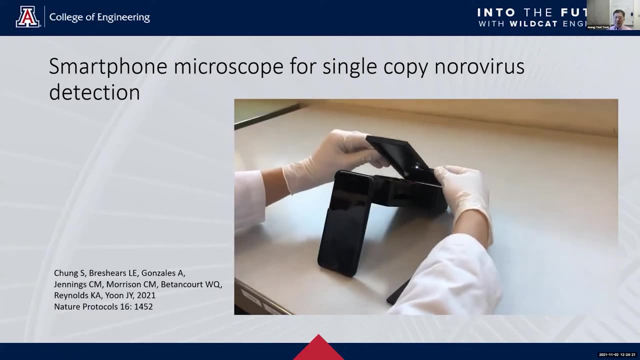 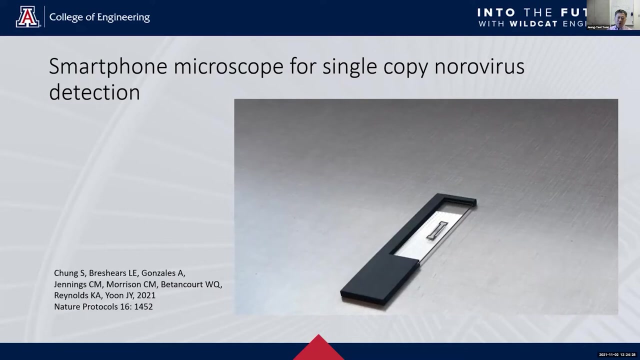 that can count your norovirus sample from environmental water samples. I'm going to play this movie, And this housing contains the white LED light source and many optical filters embedded so we can convert them into a fluorescence microscope. We are doing two pipetting. 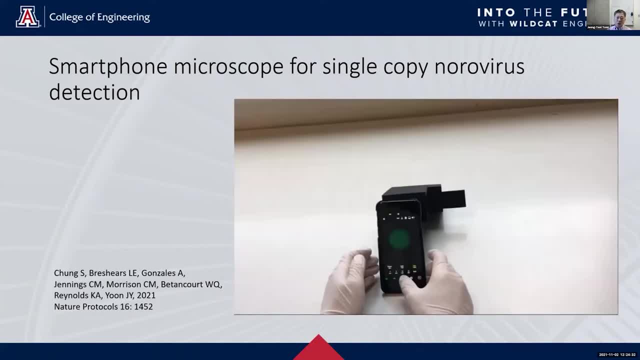 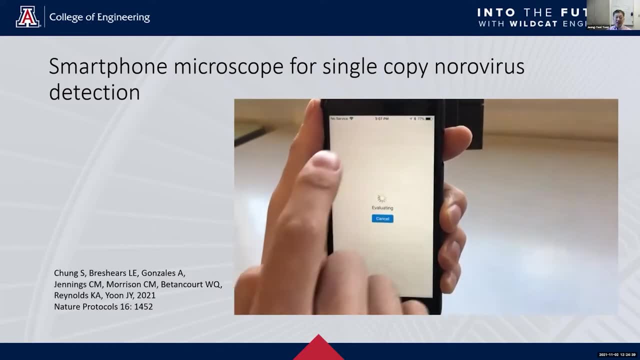 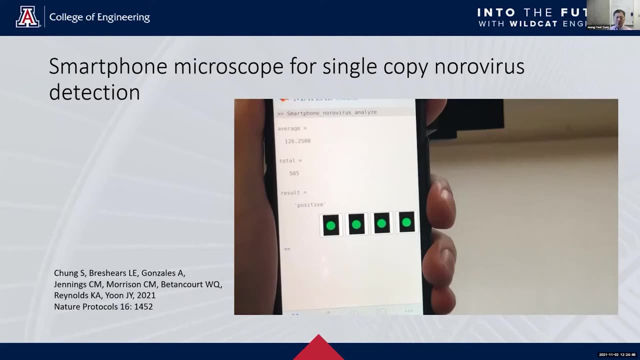 one with the antibody-contaminated particles, the other with the water sample, And then all those image analysis is actually done over cloud, So you actually see our analysis in the smartphone, but the calculation and analysis are all done on the remote server. 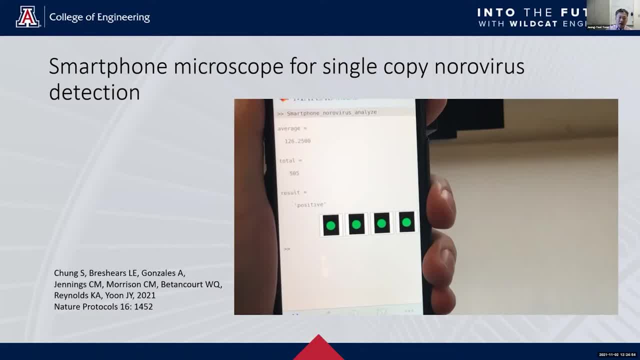 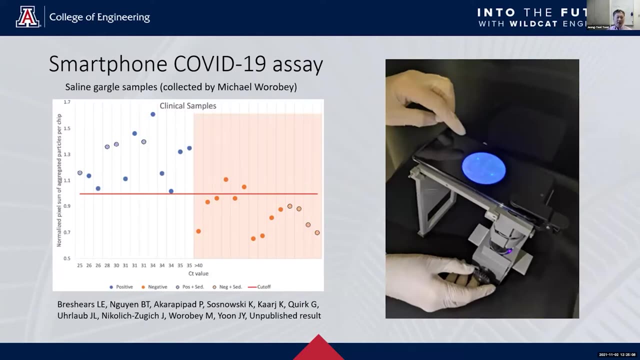 So we got a lot of mediation on this one as well. And obviously when we published this paper we got COVID-19 pandemic. So we wanted to adapt this technology for COVID-19 assay. So the device got even smaller and then simpler And you are using saline goggle samples collected. 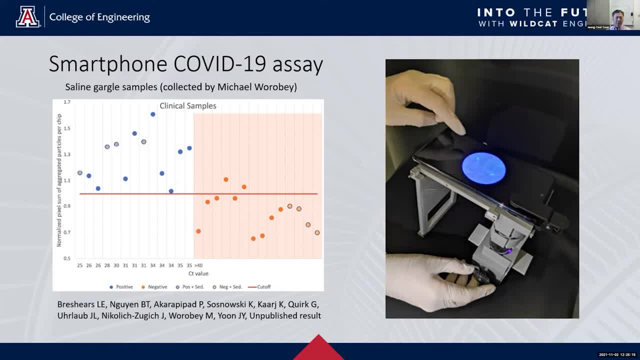 from our students And you can see that the sample size is much smaller than the actual sample size. So you can see that the sample size is much smaller than the actual sample size And this is our clinical data. And then all positive samples are classified as positive. 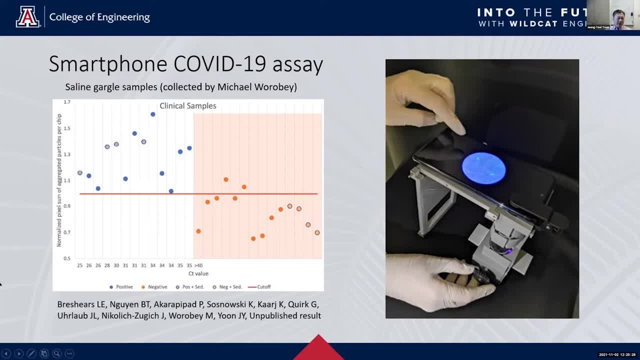 And most of your negative samples are classified negative, with the exception of two samples, And we believe these two are actually positive. Maybe the students got exposed to COVID-19, but the virus load is really low So the PCR cannot really detect them. but we can detect them using our method. 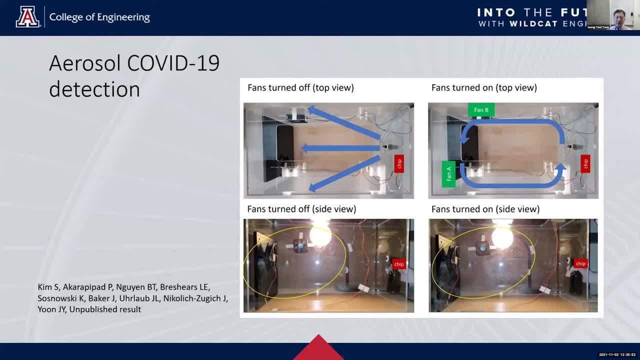 And then we also, since our detection is so sensitive, we can detect directly from aerosols. So we're not collecting samples from the humans, but we are collecting samples from the aerosol passively collected on your paper microfluidic chip. And we can still do that. 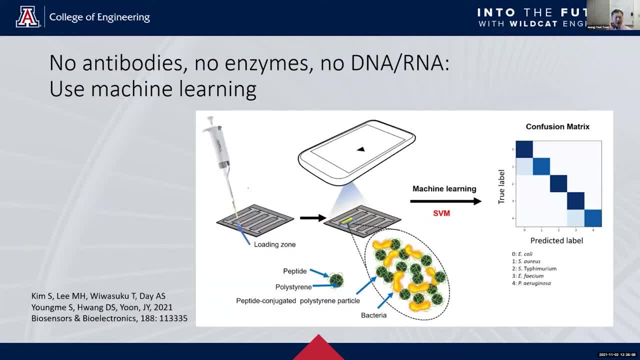 detection And finally, the one we are working on, is that the. I wish you had a microphone, but you don't. Let's try that out. Think about this for a minute. Do you have an idea of what you can do to detect this? 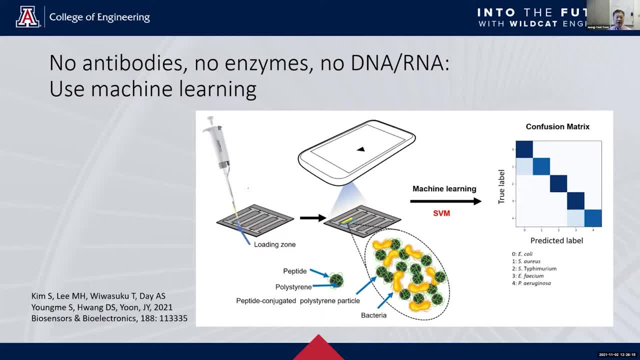 to develop a biosensor that requires no antibody, no enzymes, no DNA or RNA, but use machine learning to sense anything, Because for many biosensors you need to know what you're looking at So you can prepare antibodies or enzymes or DNA, But can you have a universal biosensor? 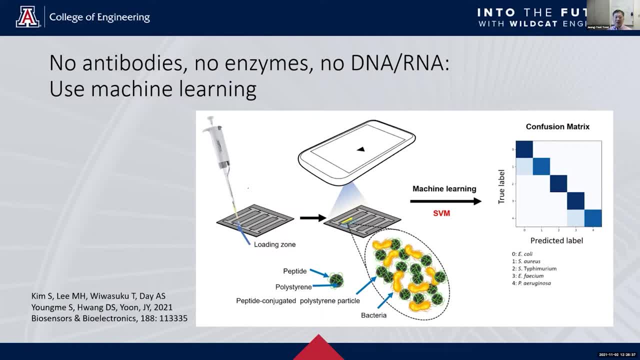 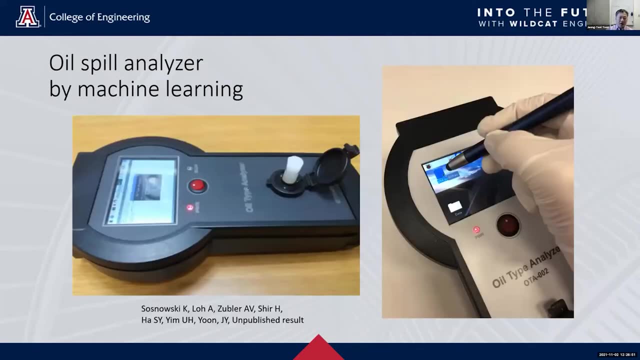 that will tell you. based on your pattern, then figure out what do you have in our sample. Right now we are using it for identifying bacterial species, But eventually we want to expand it towards the many different virus detection. I'm going to skip the last slide, And so this is the lab photo that has been taken last year. 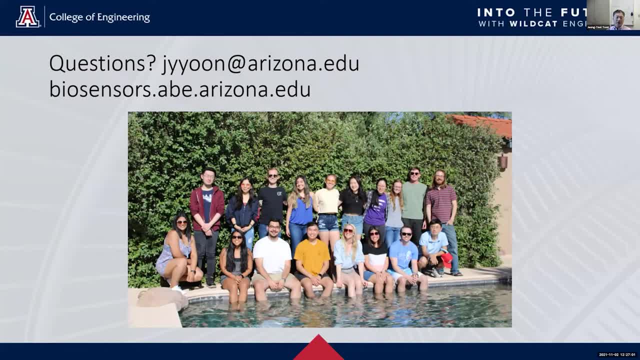 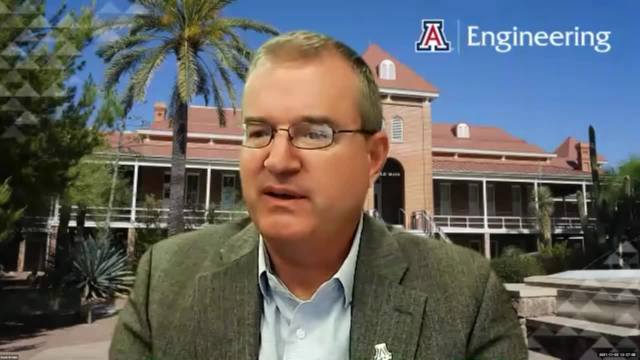 So I'd be happy to answer any questions you may have, And thanks for your attention. Excellent, You can unshare that. Thank you, both, Judith and Jeong-Yul, For some really nice presentation. So we're going to move into the Q&A portion. 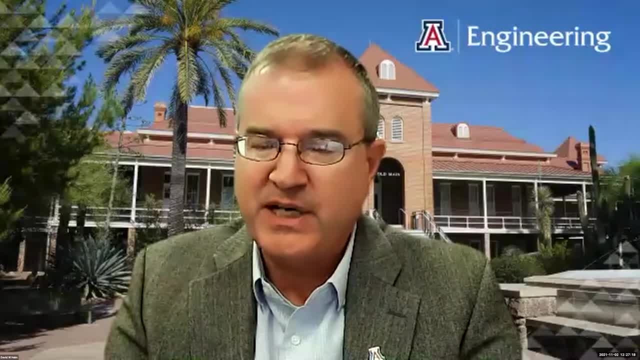 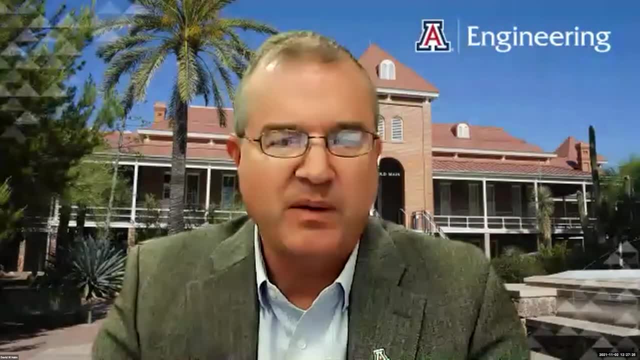 I encourage those in the audience to use the Q&A chat. Judith's already answered a couple. I've pulled questions that were pre-submitted by the people registering, So I'm going to start with those and work our way through and pick up, as we can in real time, some additional questions. 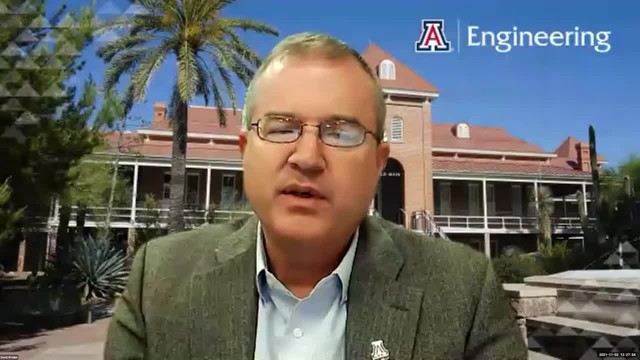 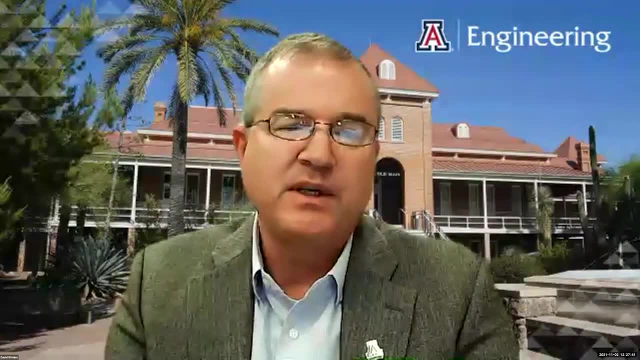 So one question is asked is: what are the most challenging factors preventing these technologies that you both are working on From transferring this technology to actual clinical uses? And we'll start with you, Judith, And then we'll go to Jeong-Yul. 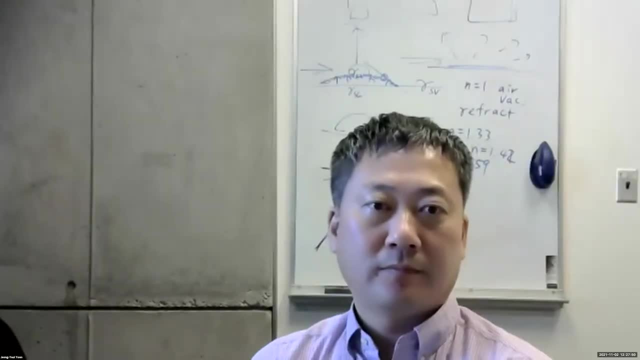 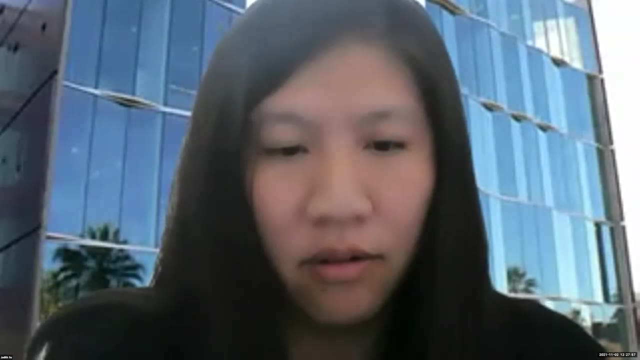 So, for our specific case, it's this use of this optical fiber that we use to couple light into our devices. So this optical fiber is really, really fragile. It's around 500 nanometers in diameter, And so it's easily broken, And it has to be precisely positioned next to our sensor using 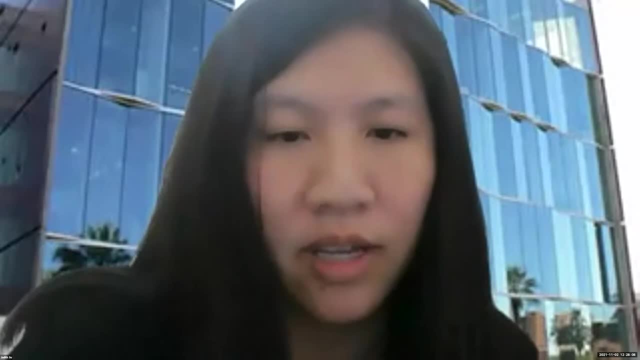 a nanopositioning stage, And so what we've been doing is we've been working on working on what's the best ways to do: alternate light coupling into our device to eliminate the need for this optical fiber, And so once we can eliminate that, I think that's our main impediment to translation out of. 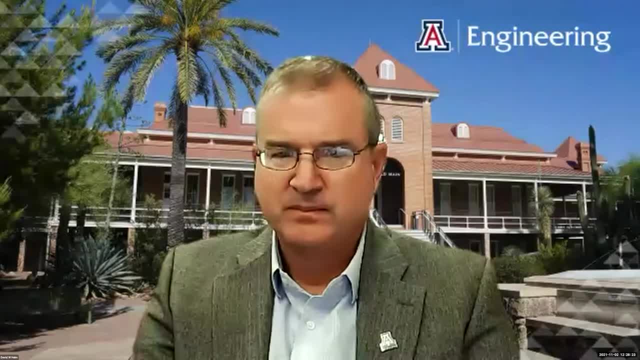 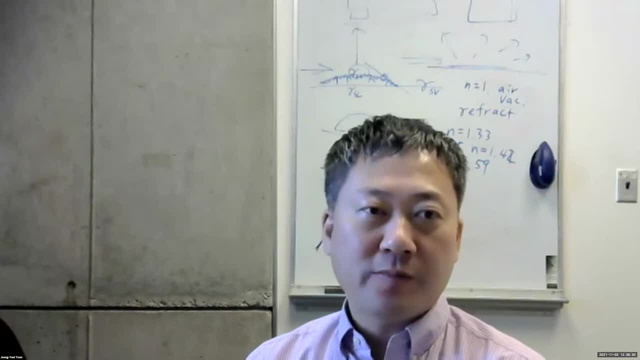 the laboratory. Okay, very good, Jeong-Yul. So my immediate most important concern would be: you know, we are using the commercial smartphones And they have their own, you know the IP rights, And so we developed a lot of different. 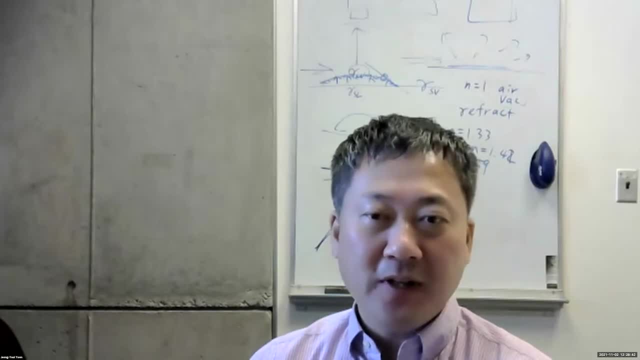 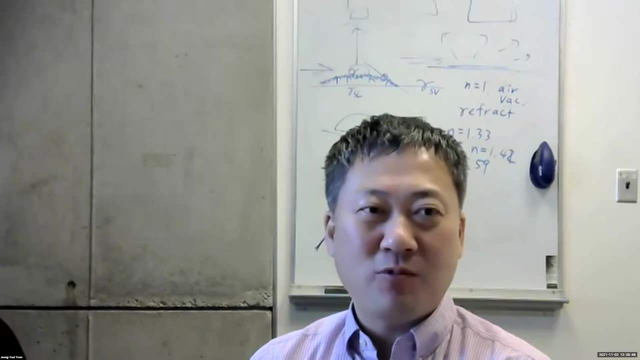 smartphones, And then we're not really asking their help. we developed on our own, But sometime later they just step in: oh, this is ours, you can practice this, And that's the biggest part I'm really concerned about. So I think some people are a little, I think the Android phones are a little. 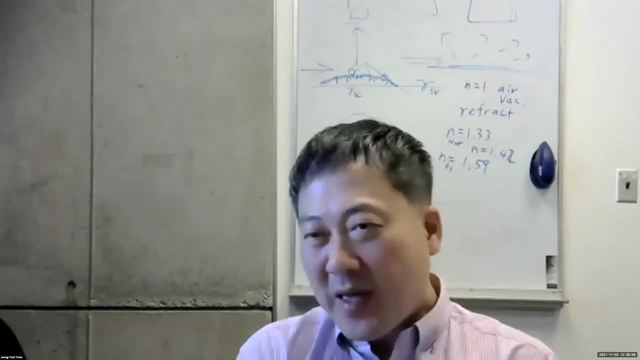 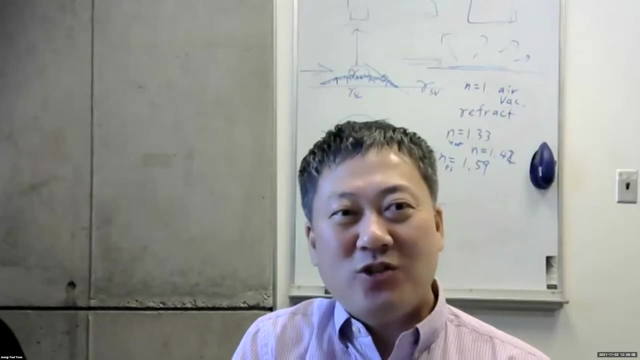 bit more open architecture. So so in the past I'm a big fan of the iPhone, So I have been using iPhone all the time, But maybe I need to switch to a more open source, some smartphone architecture. So that's the one direction we may want to pursue, But the other direction would be: 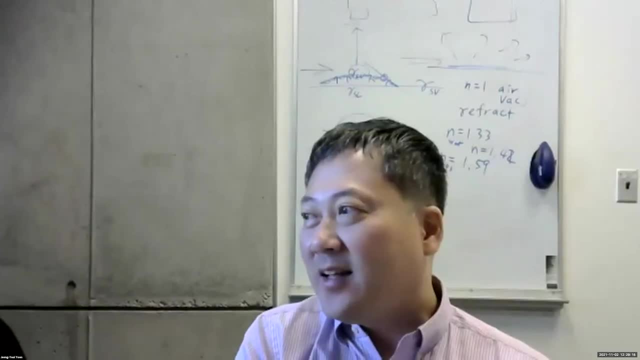 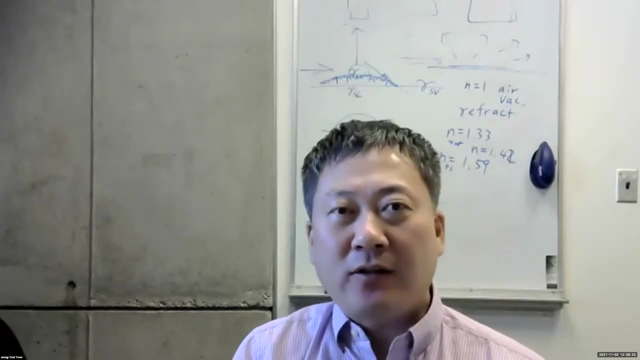 forget about the smartphone. create the small, the Raspberry Pi based camera and the Raspberry Pi detection device. Then we don't really have to worry anything about the commercial things. So I think that is the biggest bottleneck, And the second bottleneck is that we may need to get 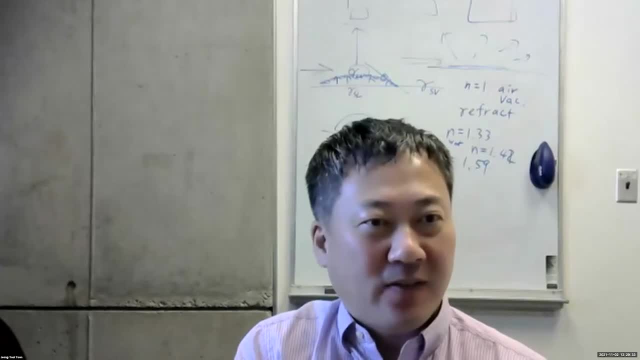 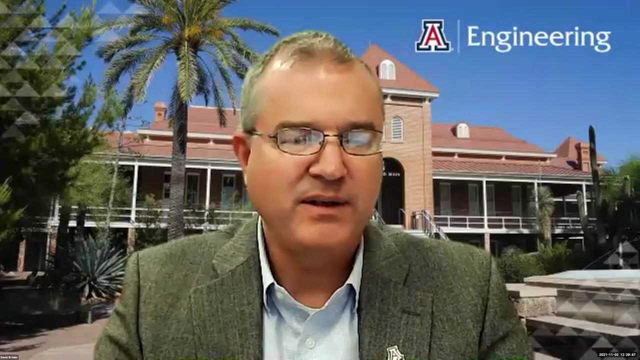 an approval on the smartphone itself, Because if you're using a smartphone, your medical diagnostics it may be considered as a medical device. then they must go through all those, the FDA clinical trials and approvals. So yeah, Thank you. Thank you, I'm going to stay with you on a somewhat related topic, which is 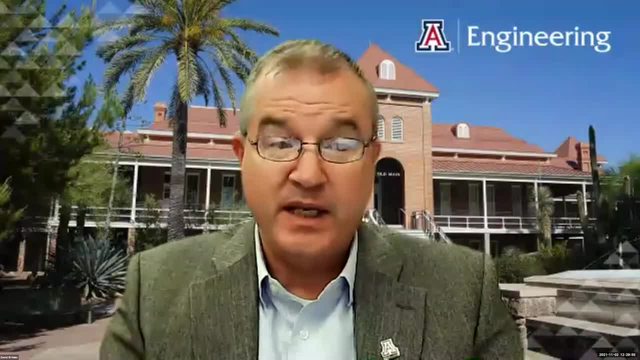 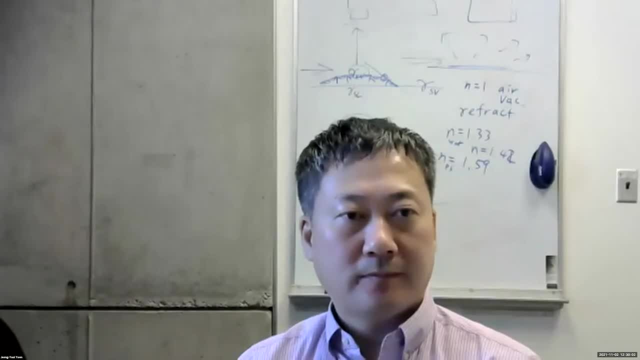 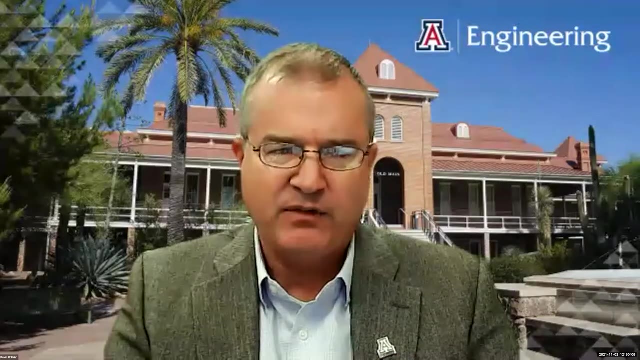 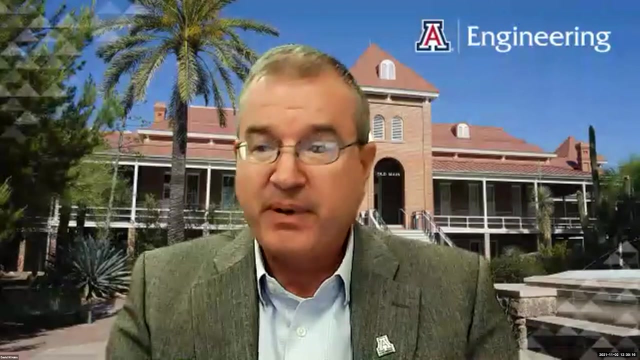 we know, when we can talk about medical devices, that HIPAA imposes strict regulations with patient health care data. So again, as you move forward transitioning these, your your really novel technologies, do you have additional HIPAA compliance? We have all the support devices to continue shooting CC kind of. 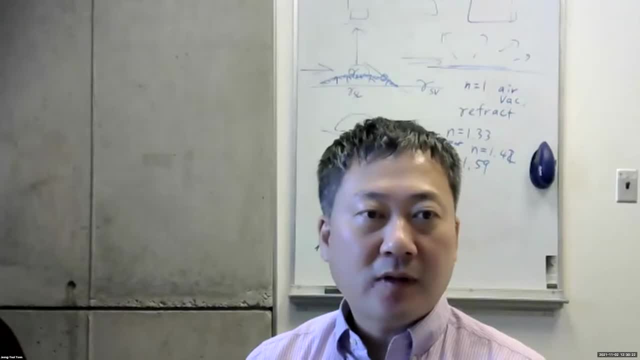 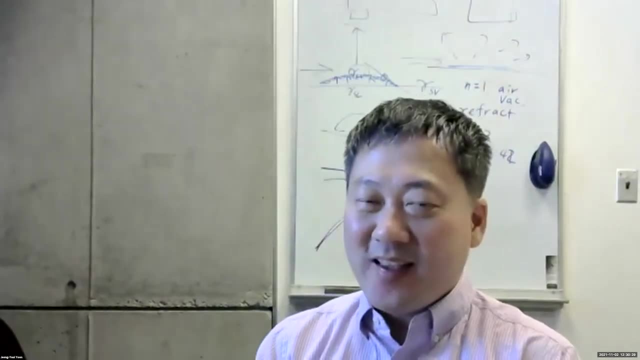 client concerns cyber security, those types of things when you're talking about using a patient's cell phone to record, you know, patient health data. So, Kidis, do you want to go first? Just speak with you on that one, since you're the cell phone person. 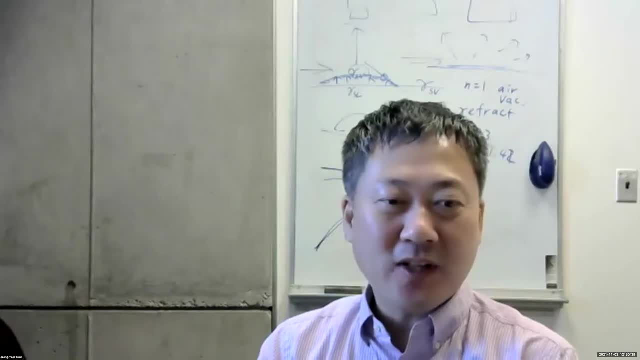 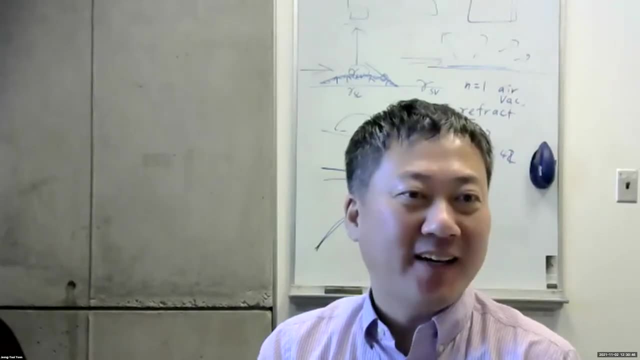 OK, sounds good. So in my personal point of view, probably put the I really want this price tag something like less than the co-pay you make. So if your co-pay is $30, I'm going to make all of my devices cost less than 30 bucks. 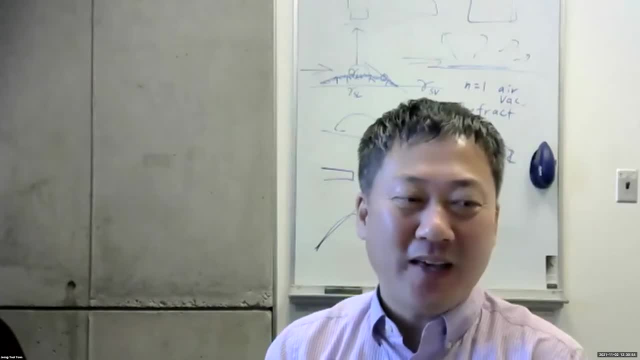 Then you don't have to worry about insurance, And the problem is we're going to face some resistance from the existing medical industry, or maybe there's some regulatory guidance. But you know what, Back in the old days, when the pulse of similar first came out on the market, 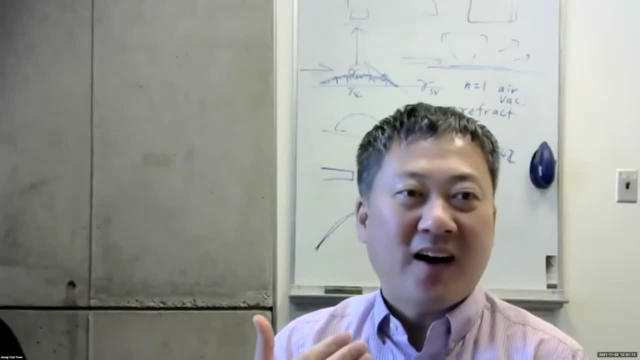 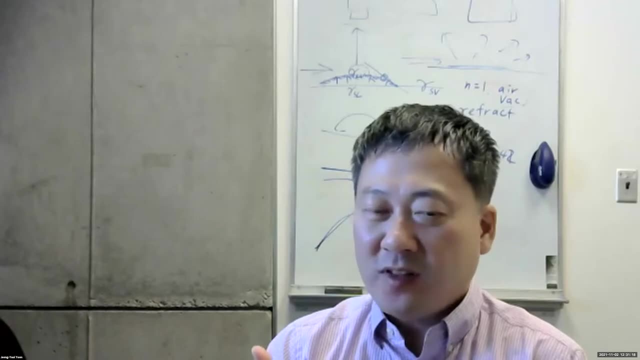 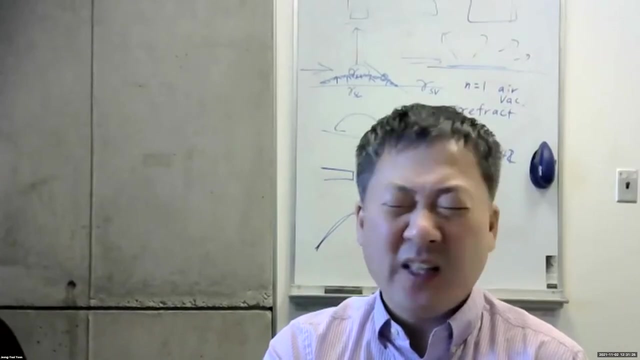 when the first glucose meter came out on the market, the regulation regulatory. many people actually raised a concern about how can a person purchase this device and you know, they read, you know this data and interpret in his or her own and that's basically infringing. 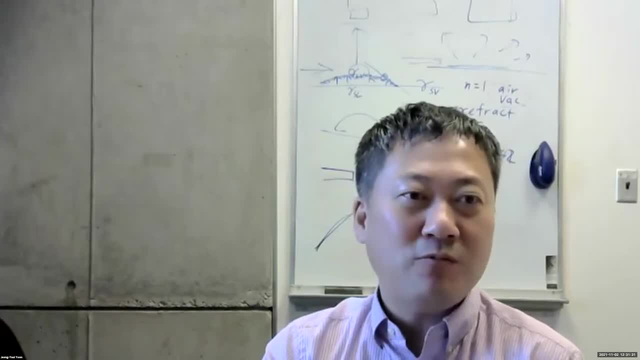 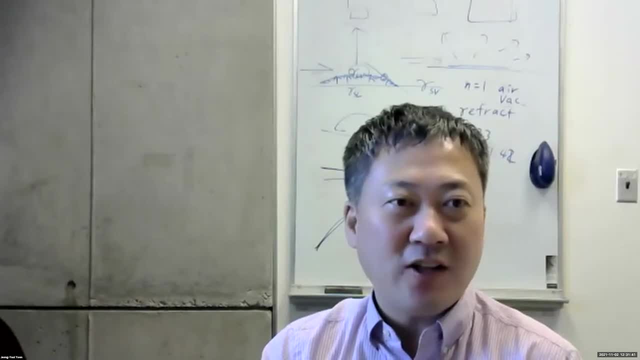 and glucose meter and you can purchase the pulse of similar and glucose meter without doctors prescription and they're really cheap and then they can just read and interpret all the data. So eventually that's going to happen, but I wouldn't want to make it happen much earlier than. 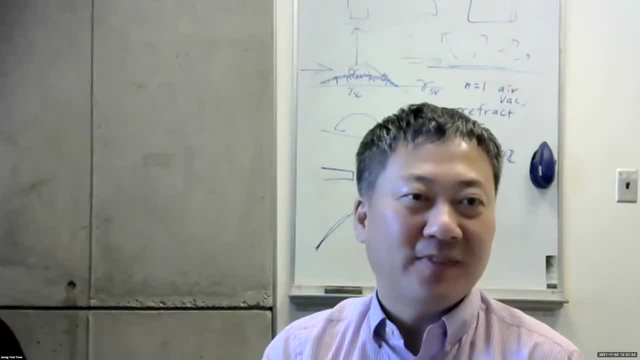 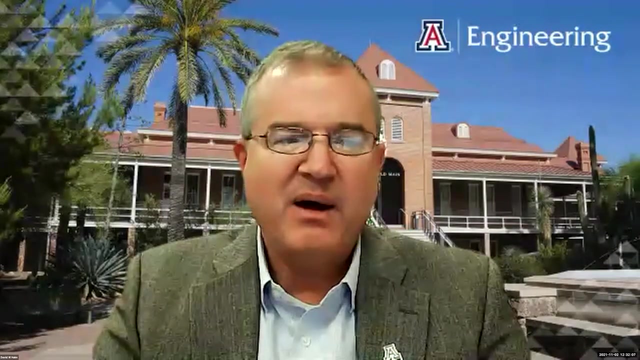 you know, the, maybe in the next five or 10 years, So so that we don't have to worry about the, the insurance regulations and the doctor's prescription and doctor's order and so on. Excellent, Thank you for that, Judith. I'm going to go to you now with the. 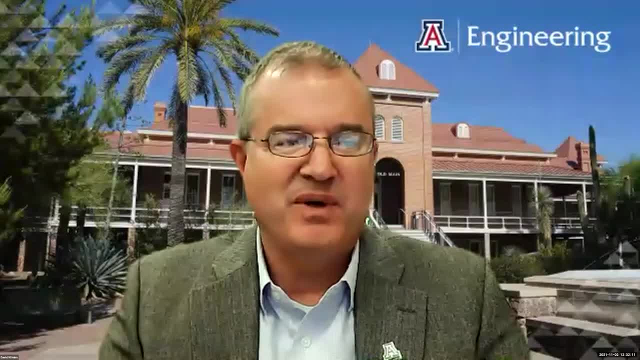 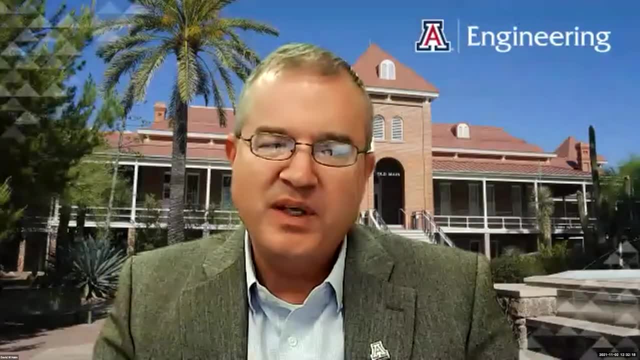 with the question. So this is an interesting question. You're you're very much versed in photonics and biophotonics, So this is kind of a future looking question. You know someone asks: will we be able to at some point in the future? 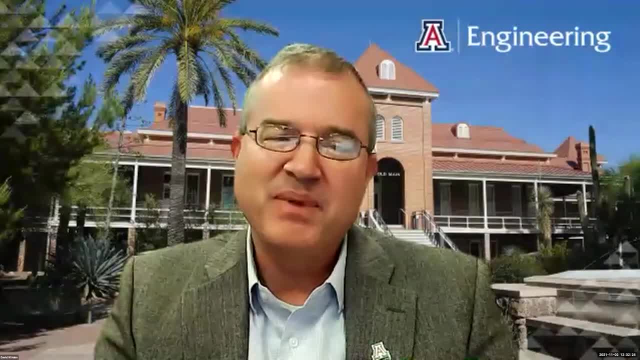 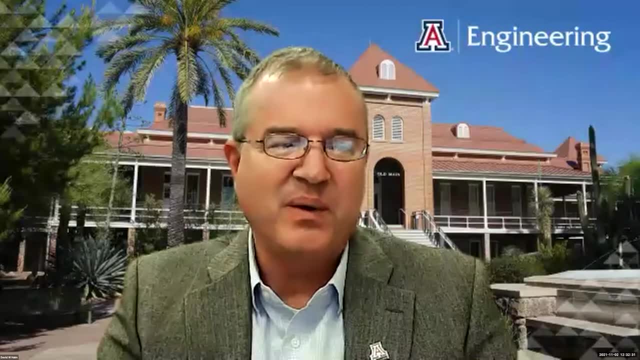 you know, look into your mirror and have it tell us something about our conditions, sort of a you know mirror, mirror on the wall, who's the healthiest of all? kind of question. So I think it's an intriguing question. And where do you see that going, Judith? 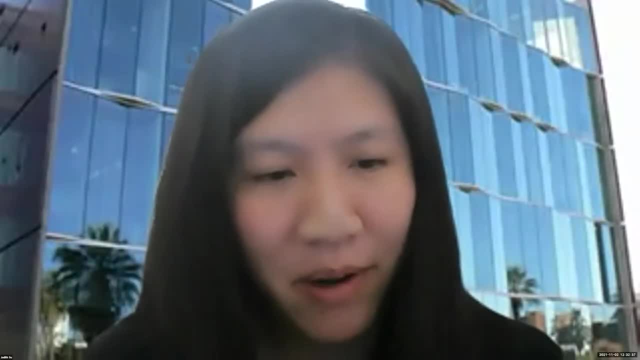 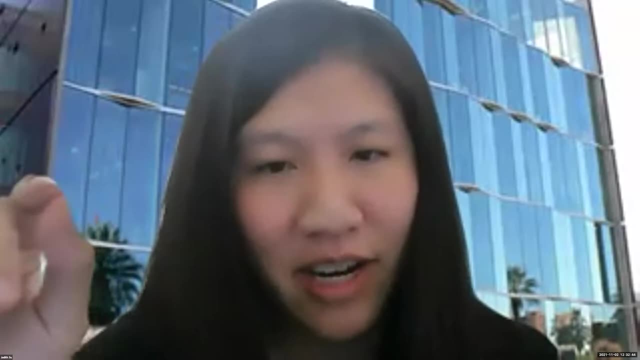 I think that's a really interesting question. In fact, just the other day I was reading a book, a paper that had just come out, where it said that you know, people could zoom into your eye, like a picture of your eye, and detect whether or not you had COVID with like 97% accuracy. 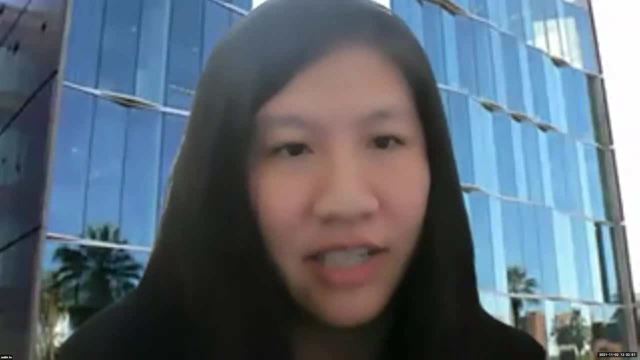 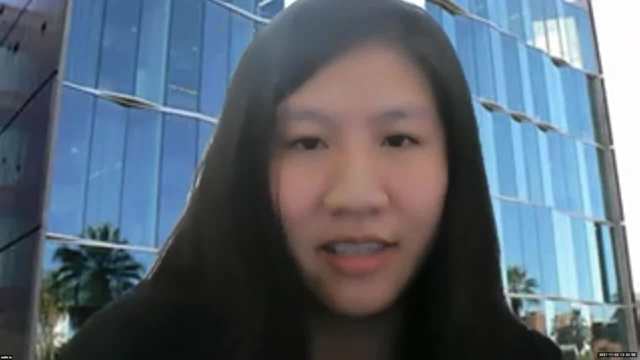 So I think these sort of technologies- it was was incorporated a lot of artificial intelligence, of course. So I think these sort of things are definitely on the horizon And I think people are working on these technologies right now. So it might seem very futuristic but you know, as with the COVID example, people, people have started to 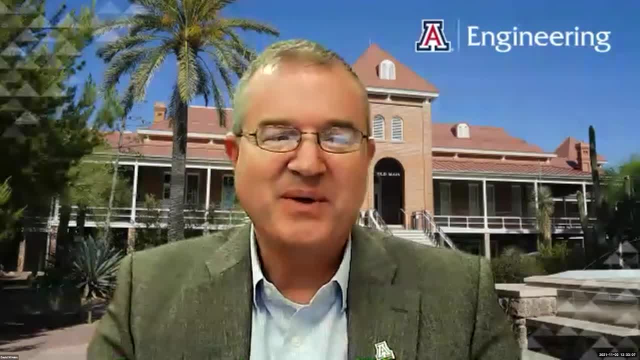 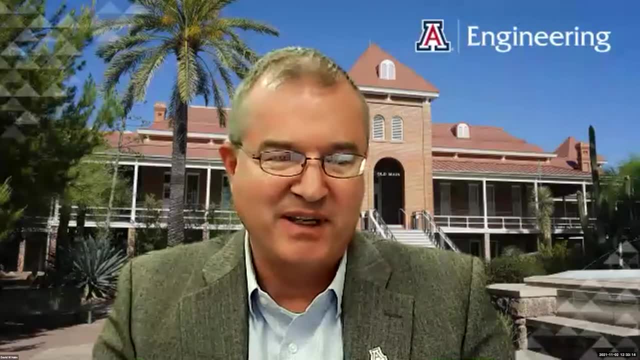 do these things. That's fascinating. Good, I agree with you. You know the idea that. that you know, I know there's a lot to be done with the eyes around even diabetes and things like that of of getting diagnosis. So I agree, It's a very intriguing. 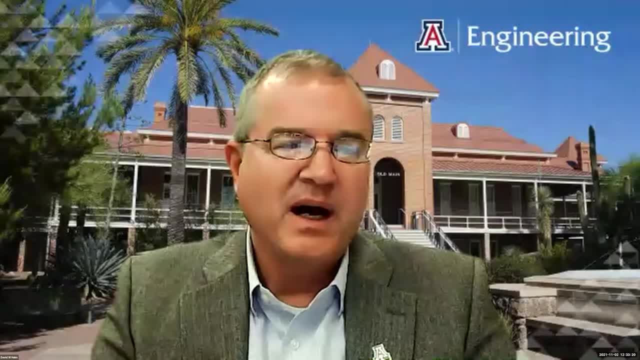 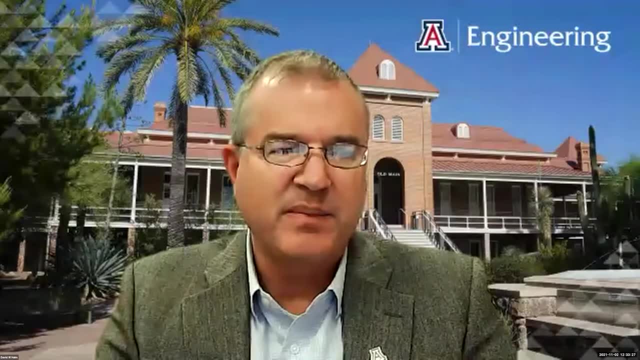 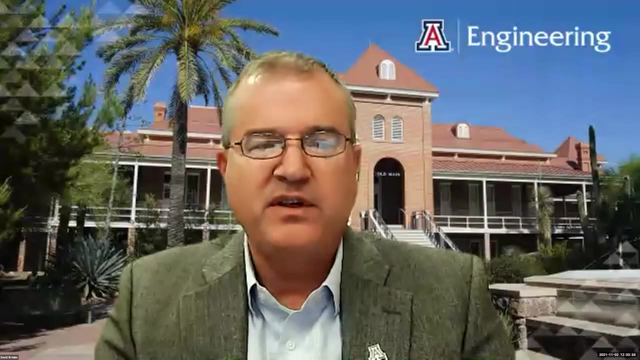 question and probably we'll get there at some point in time. So someone asks to discuss the issues of accuracy and drift in your devices. Is this a major issue for you know as, as John you'll just describe sort of over the counter technologies versus you know devices. 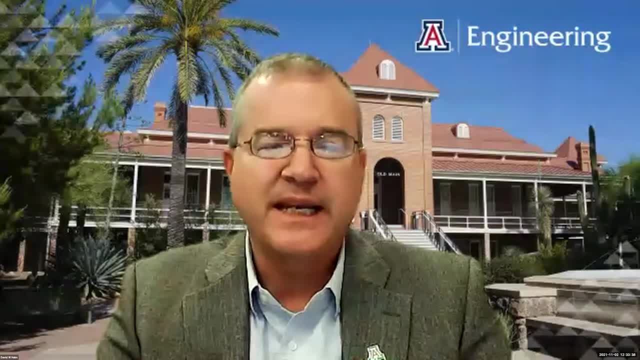 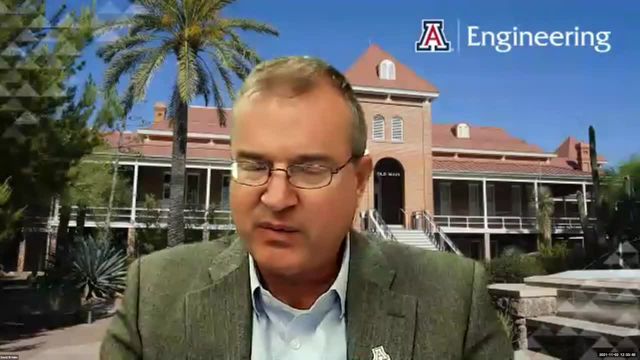 that are prescribed by a physician and possibly use in the future. So I think it's a very intriguing clinical setting. So, as we bring this out to the masses, does that present problems with calibration, accuracy and drift? So I'll start with you, John, you'll, then I'll go to Judith for her. 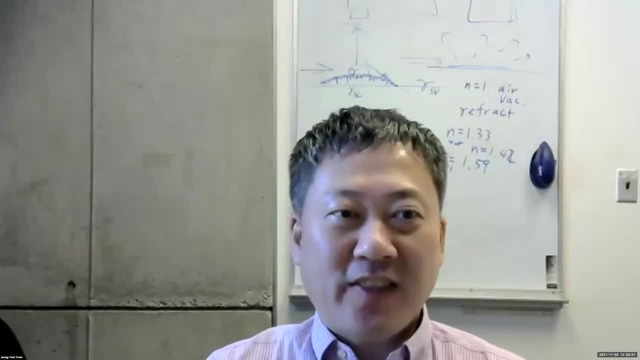 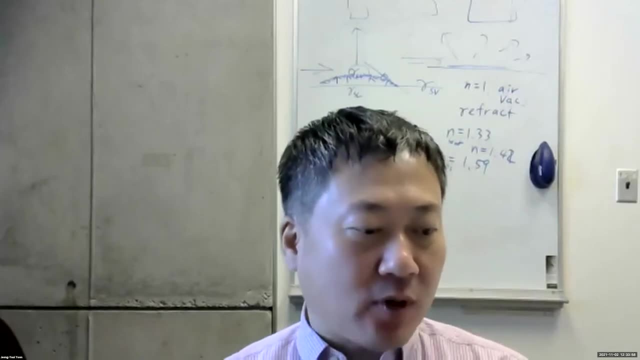 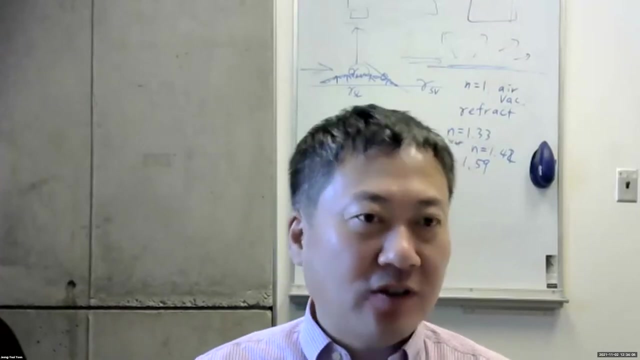 own interpretation. Well, the calibration is a major thing because, frankly speaking, before you do the assay, all the time you need to manually calibrate them. So, for example, how I'm going to position your phone and how gonna, if it is based on the, the light intensity detection, and if it 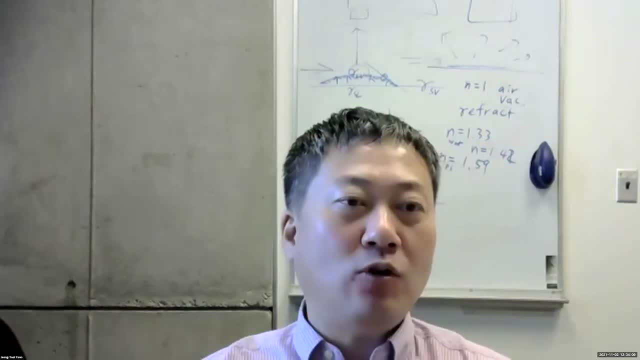 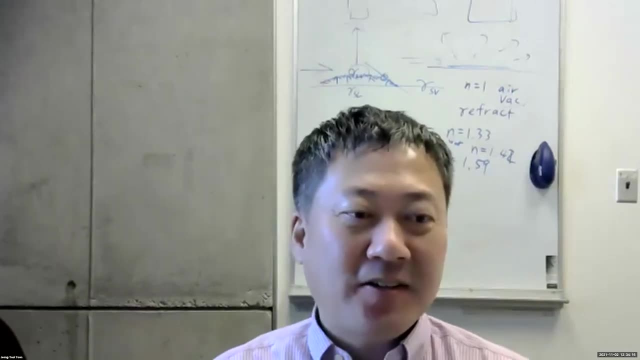 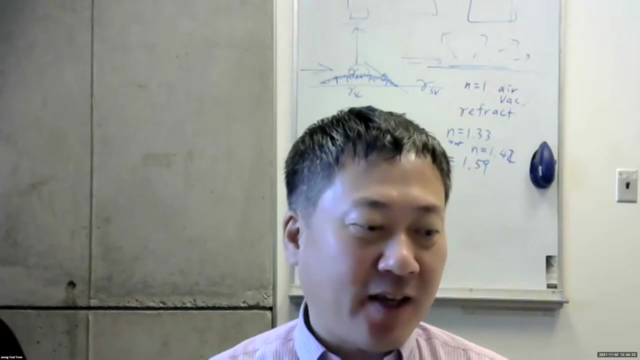 is based on the microscope Imaging, then how you need to manually focus them. So eventually we need to create a system that are set to calibrate automatically. So that's a lot of work And then a lot of the the industry, or you know the developments. you're supposed to be the they're supposed. 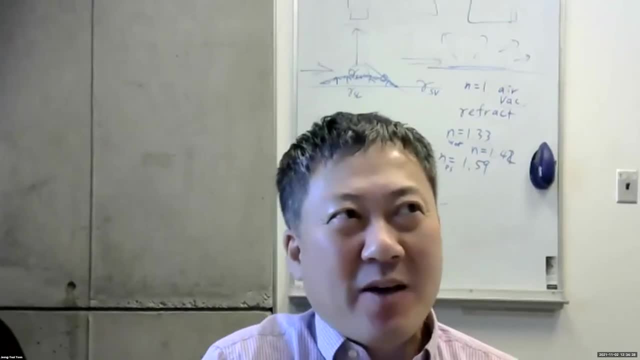 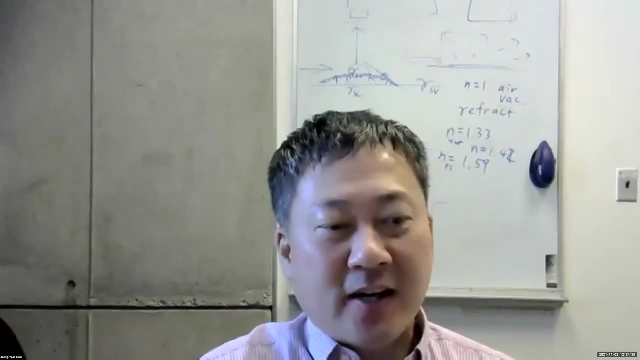 to be done on this, down on this. but it's less academic but more commercial development at that point. But certainly, yes, it is needed, because if you're asking each individual to calibrate your Machine all the time, then people are not going to use it. 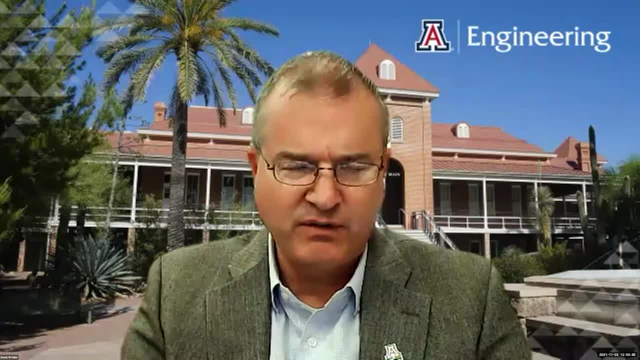 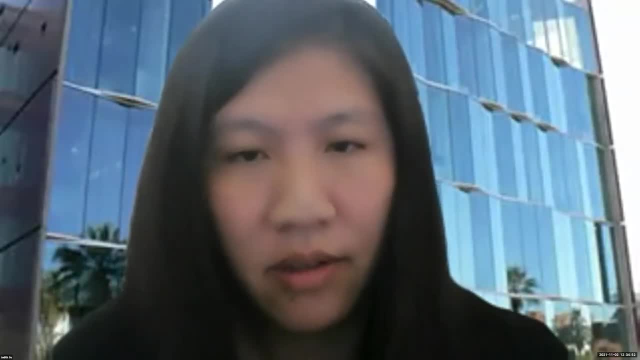 Good, Very interesting. And, Judith, when you look at some of your technologies, how do you view these kinds of issues? Yes, I think accuracy and drift it's really important And you know we do a lot of studies to. 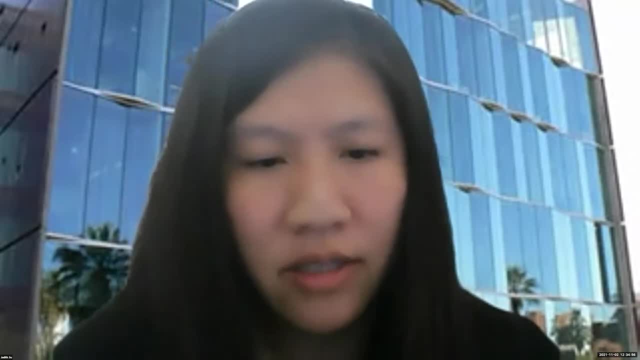 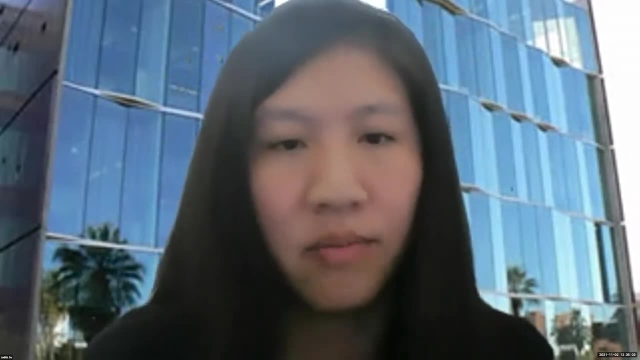 try to characterize it and minimize it, And I think there's always going to be, you know, a difference in the quality of results you get from you know, a large instrument that you find in a clinic versus something that's portable and and wearable at this point. So you know you might. 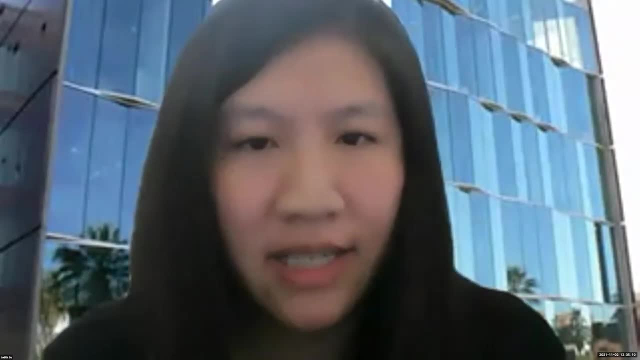 have you know. for example, if you, you know, take a pregnancy test at home, you can get these very cheap over-the-counter tests, but then people always want confirmation from a physician where they have, you know, more accurate tests. That's considered like the gold standard, And then I've seen that they started to sell these. 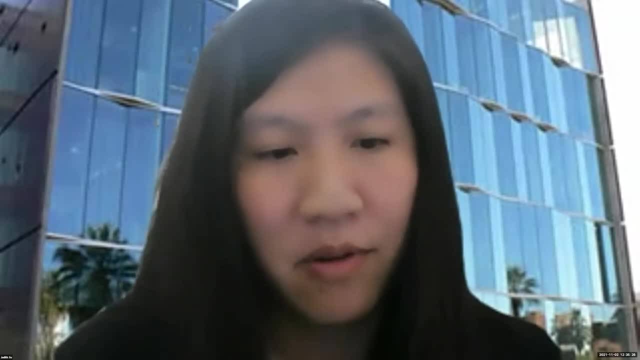 sort of portable handheld ultrasound devices, But of course you know the accuracy of that compared to, you know, a big instrument that you see in the, in the clinic. So I mean, when you have smaller point-of-care devices, you know they might be cheaper, they might, you know, be hand-held, but they're not as expensive. So I mean, when you have smaller point-of-care devices, you know they might be cheaper, they might, you know, be hand-held. So I mean, when you have smaller point-of-care devices, you know they might be cheaper, they might, you know, be hand-held. 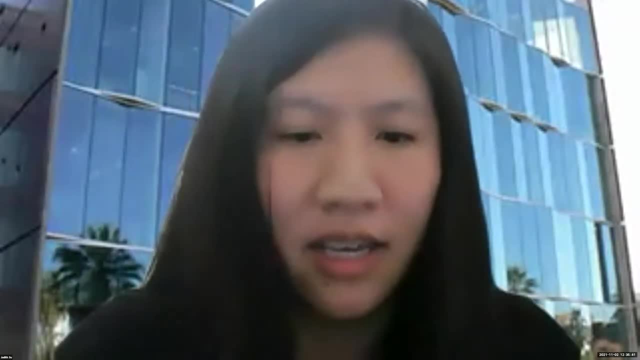 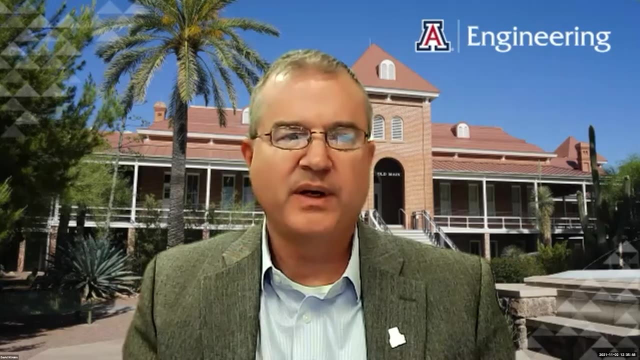 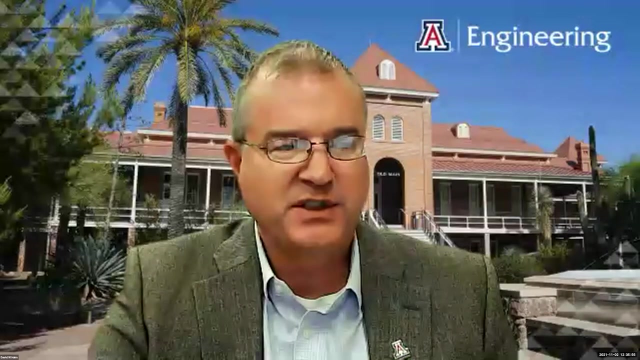 But I think you're going to sacrifice things like accuracy. you know when you, when you start doing things like decreasing cost and size- Yep, I totally agree. So the balance of widespread, low-cost preliminary answers maybe, and then maybe some confirmation on more serious issues, So that's good. 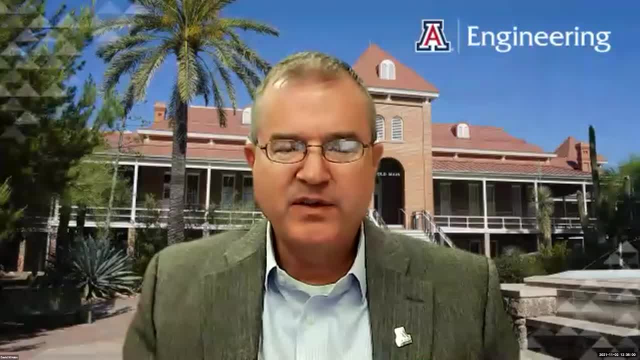 Yangyou, I'm going to go back to you and pick back up on the topic of COVID. You know we're still in the midst of this pandemic. I know you talked about COVID, but I'm going to go back to you and pick back up on the topic of COVID. 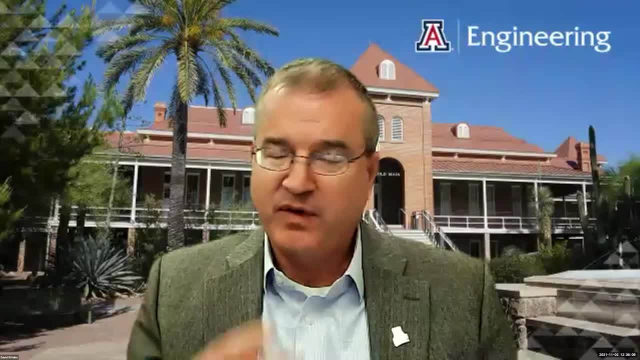 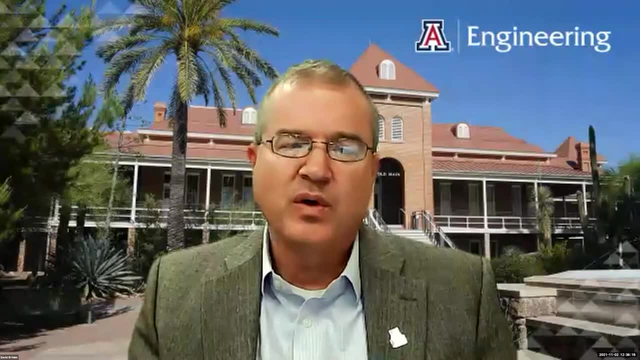 You know we're still in the midst of this pandemic. I know you talked a little bit about COVID in your presentation, both from the saliva tests and the potential to even do aerosolized detection. So you want to elaborate a little bit more on what are the 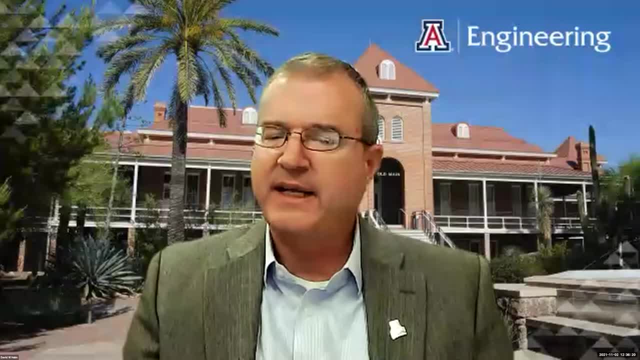 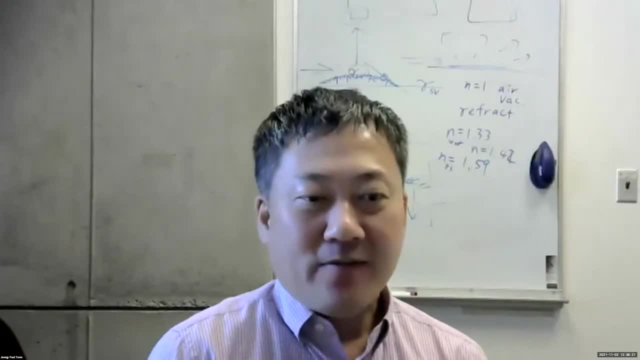 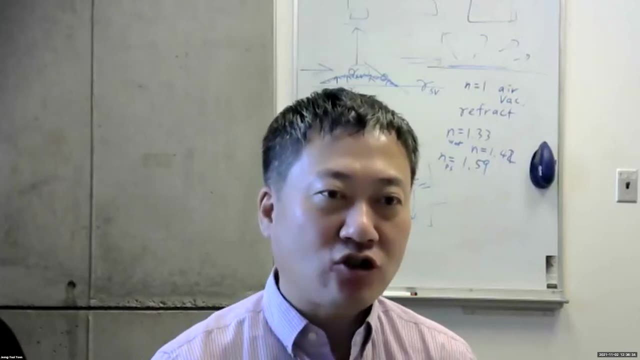 potentials for your technology moving forward and do you have plans to continue along those lines? So, frankly speaking, the we have spent a lot of time on developing COVID-19 assay, but our emphasis has been really really extreme low-level detection. 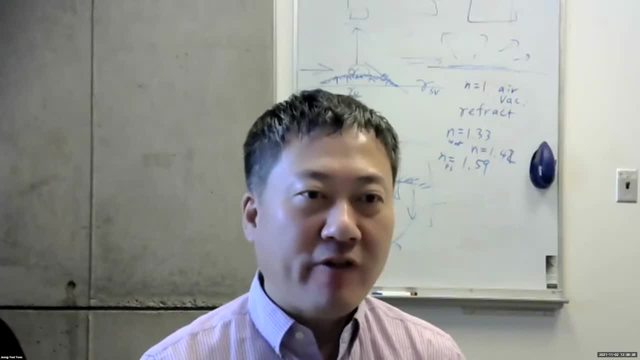 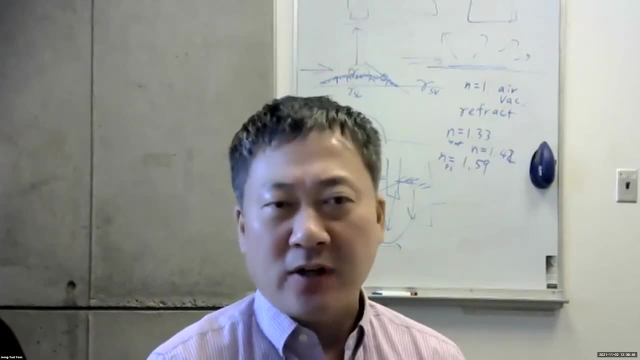 And right now we got the commercial rapid test. They are not very accurate but we can detect the- you know, the presence of your COVID-19 from your nasal and saliva sample. So I think my technology has a potential use for. 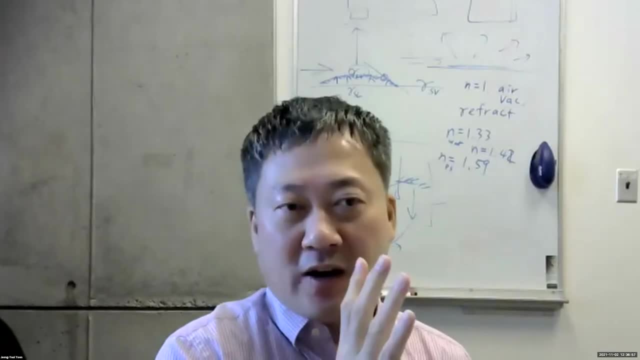 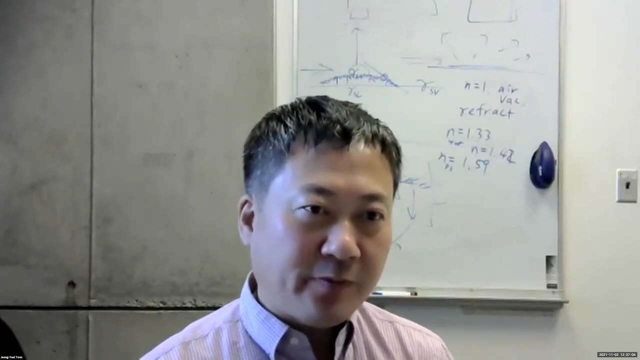 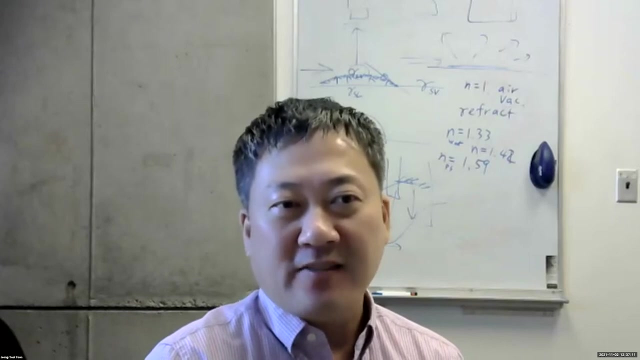 aerosol detection, not from the human samples. That's the one area that I'm very interested. Another area that I'm very interested in is that the antibody qualification, Especially neutralizing antibody. People are talking about how long you can have your protection. Of course, once you get vaccinated, you have a lifelong protection through your memory B-cells and memory T-cells. But if your neutralizing antibody wanes over time, then you're going to get a short infection. You're not going to die, of course, once you get vaccinated, but you're going to develop some symptoms. 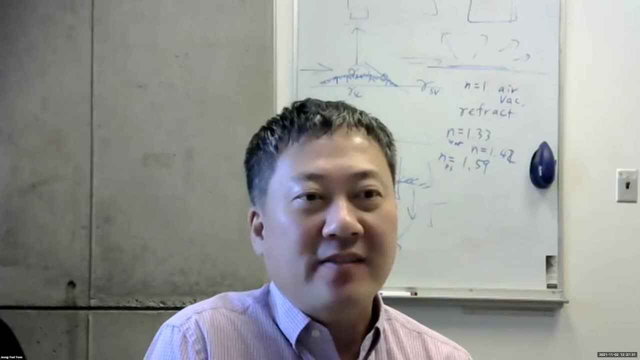 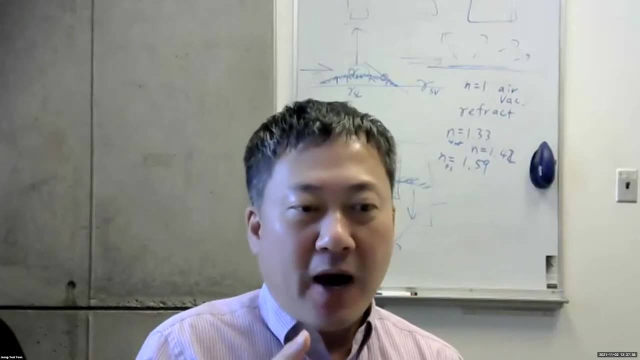 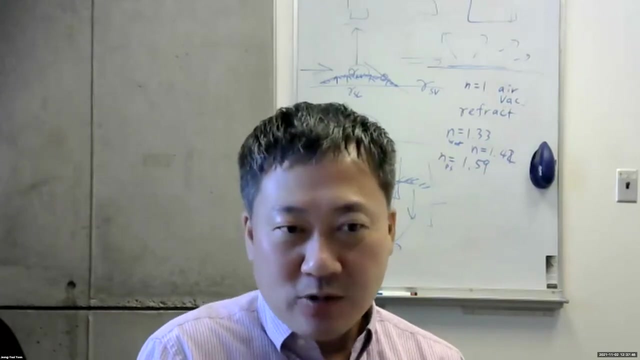 And people may want booster shots, And then when exactly that should be, Or do I really have to have a neutralizing antibody? So right now, the only possible method you need to withdraw your blood and then they get it tested in a lab Because the antibody amount neutralizing antibody- 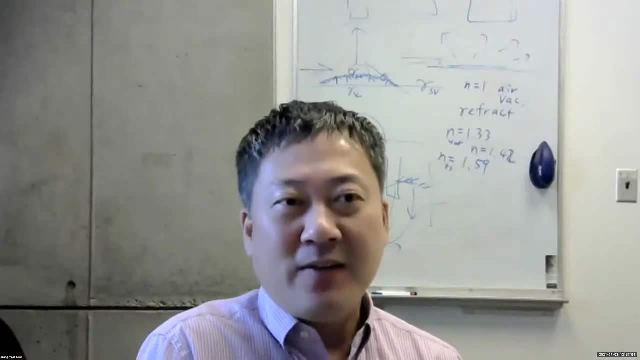 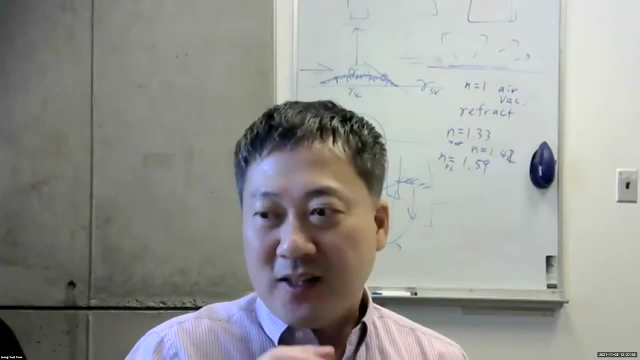 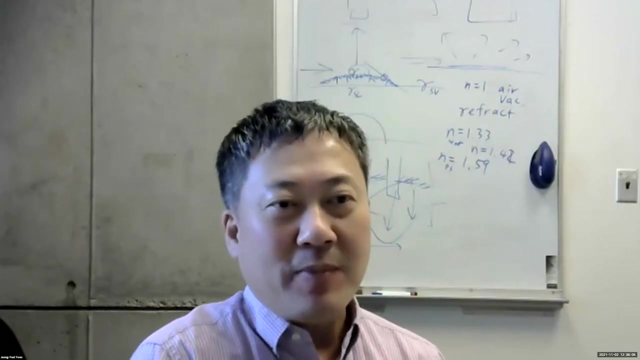 amount from your saliva is extremely low, But I believe my technology can detect them because mine is so sensitive. So right now we have just started a project detecting the antibody from saliva And then we don't have conclusive data yet, But we believe it is promising Outstanding Good And that's great. 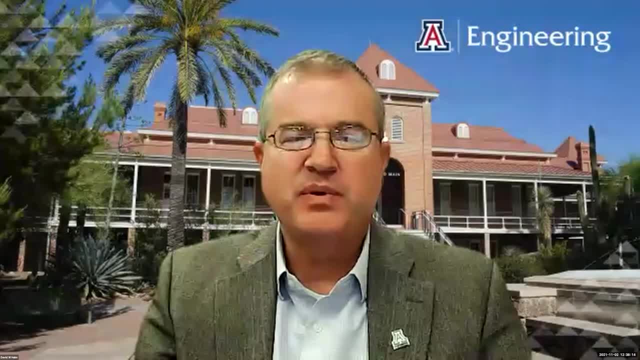 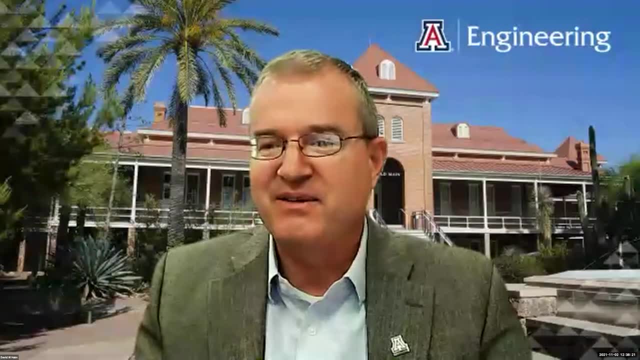 That's good to know, You know. that's an example, looking at your data that you presented in your talk, where drift is an issue. right, You have this fine line that segregated the positives from the negatives And if that line's moving up or down, suddenly that detection is starting to come. 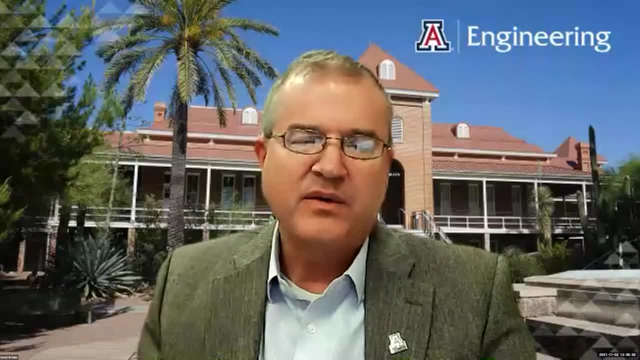 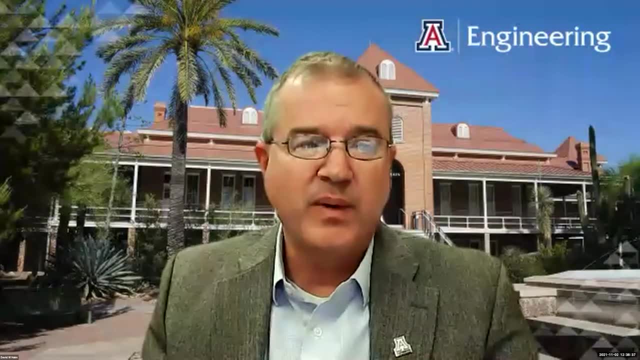 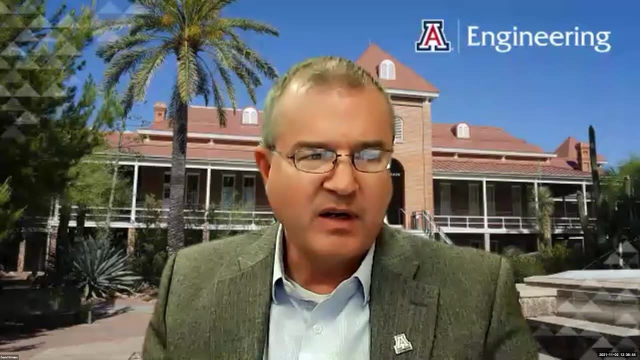 into play, right? So calibration is very important. Now, cancer remains a devastating disease, And so I'm going to start with you, Judith, And then I'll come to you, John, and you'll see if you're doing anything in this area. But when we talk about cancer detection, Judith, what sensors? 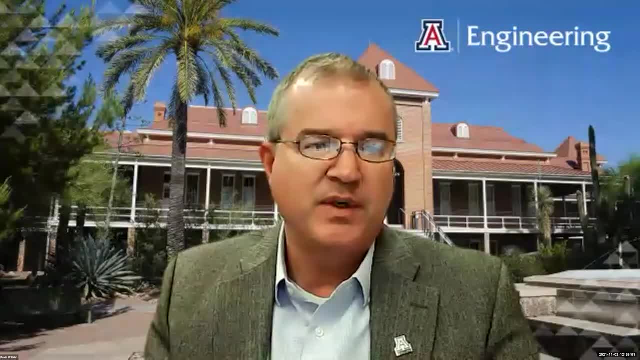 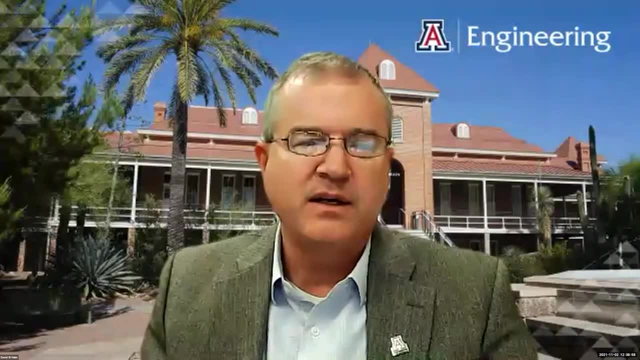 are being developed, maybe using your technologies, to, you know, detect cancer, And you kind of made it addressed this partially in the chat, but I'll ask you to elaborate. You know, when you find a circulating tumor cell, for example in your ex-situ device, how do you? 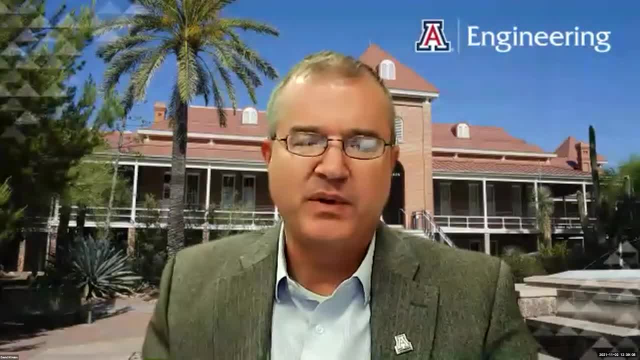 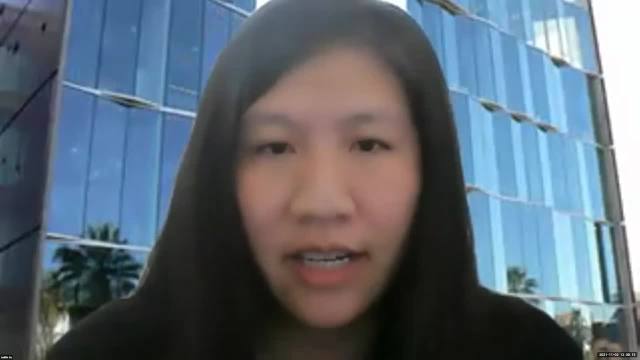 then what do you do with that knowledge, right, And how do you source that back, maybe to within the body? So talk to us a little bit about cancer detection, Judith. I think probably most of you guys are familiar with standard techniques like a mammogram, ultrasound, MRI And now, of course, 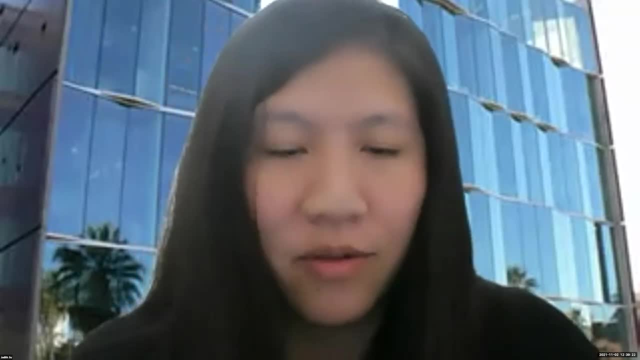 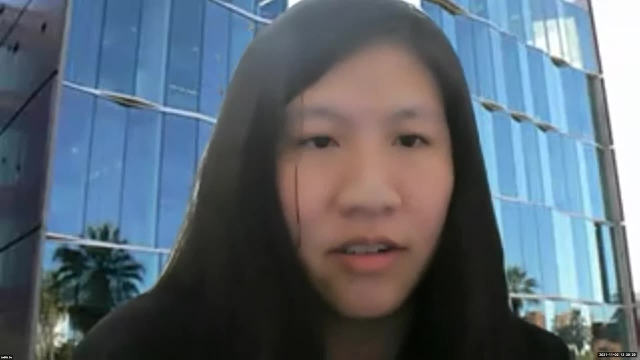 this is, you know, a huge field. Like anyone who's doing these sort of sensors, probably they'll try to target cancer at some point. So you have all sort of different detection modalities, like electrical sensors, optical sensors- everyone you know trying to detect cancer- biomarkers, And so 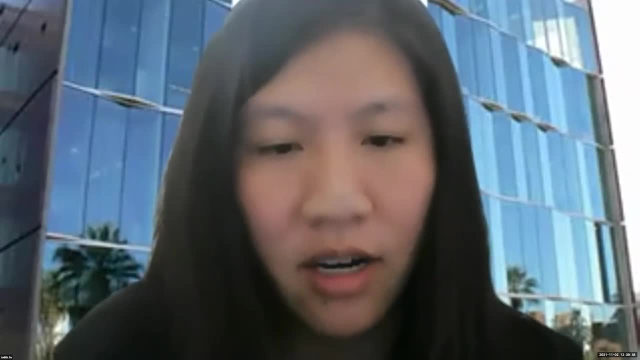 personally, what we've been doing are things like what I mentioned in my talk about the liquid biopsy. So this is, I guess, what people would call hot topic now. So there are, you know, large companies that are doing this, where you're looking for biomarkers that are shed by tumor. 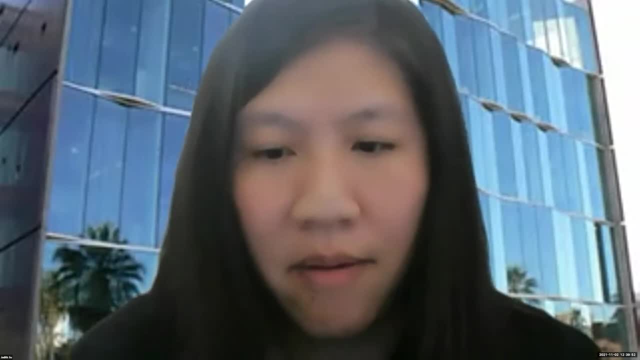 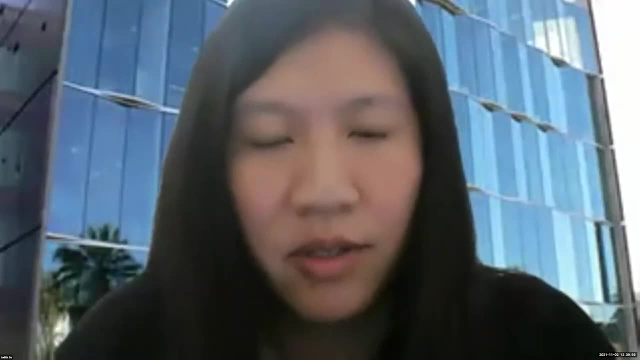 cells, whether it's, you know, DNA or protein biomarkers, And you know people have been able to distinguish. you know between, you know well. so there are different biomarkers for different cancer types. So you have to find a specific biomarker for that particular cancer type. 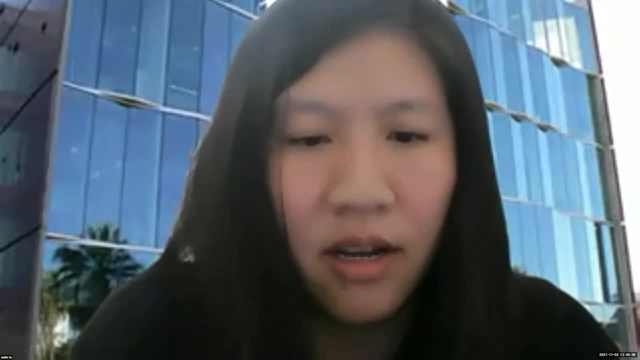 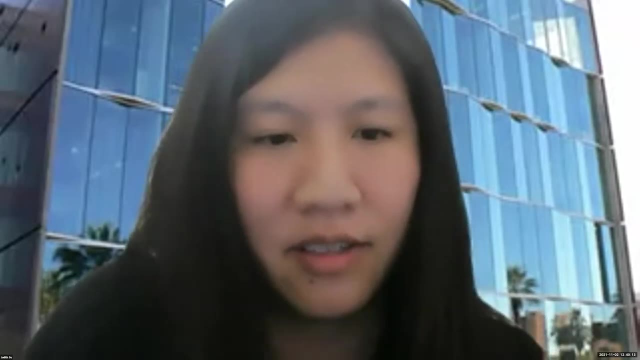 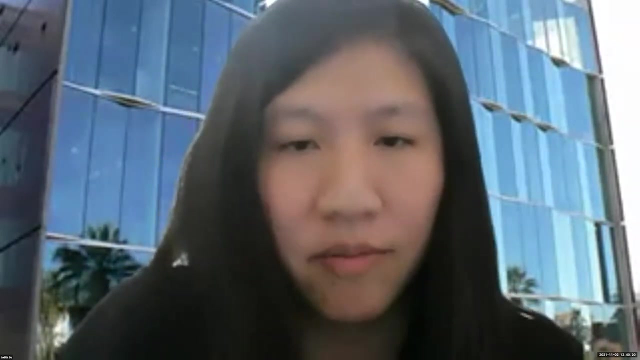 And then, for certain kinds of cancer, people have been able to get, you know, reasonable discrimination. And then it's, of course, there's all these different things, like you know, ethnicity, that comes into play for some of these biomarkers. So, in our case, what we do with when we detect these cancer biomarkers? 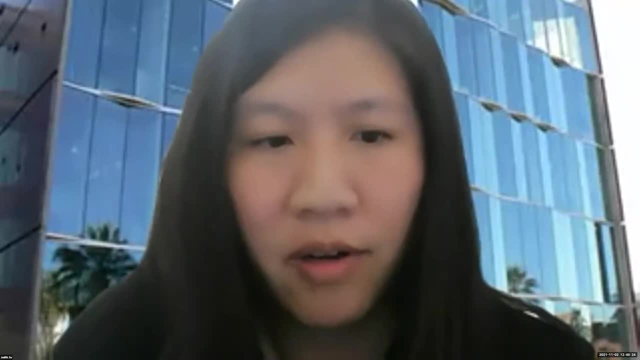 like, for example, these exosomes, is we do things like we track tumor progression, So can we see how far a tumor has progressed, And then we also might be interested, for example, in evaluating things like treatment outcomes. Like you know, if you applied a particular 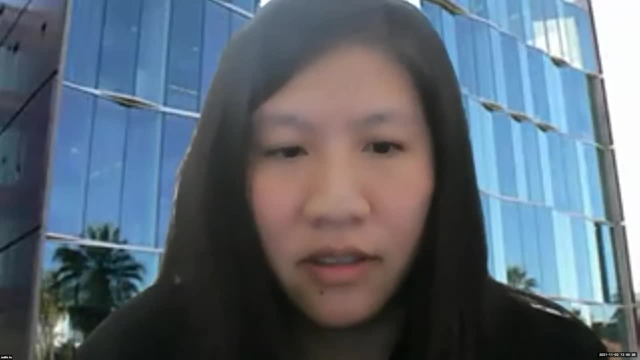 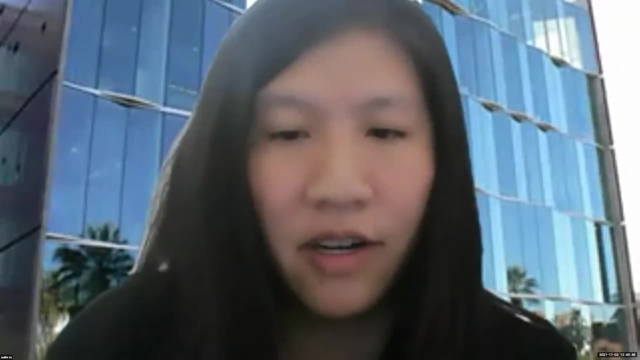 kind of treatment? how do these biomarker levels change? So we haven't yet gotten that far with our cancer work. but, for example, for Alzheimer's work, some things that people are interested in are, you know, exercise. So if you have Alzheimer's people tell you to keep your. 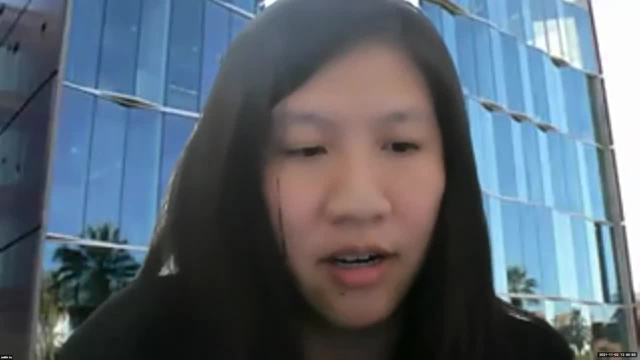 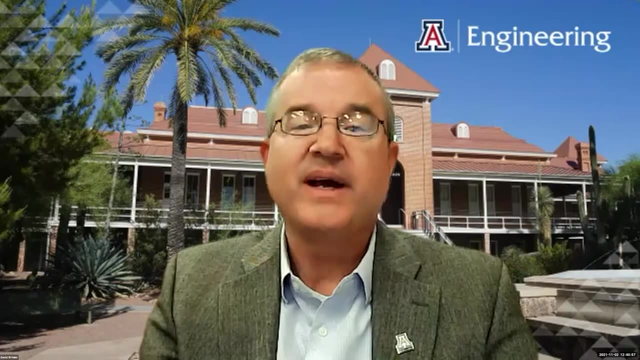 cardio up, stuff like that. And so you know, things people are interested in are like: you know, after you exercise, how do these biomarker levels change, and stuff like that. Go ahead. Oh no, no, go on. I was going to say you know. 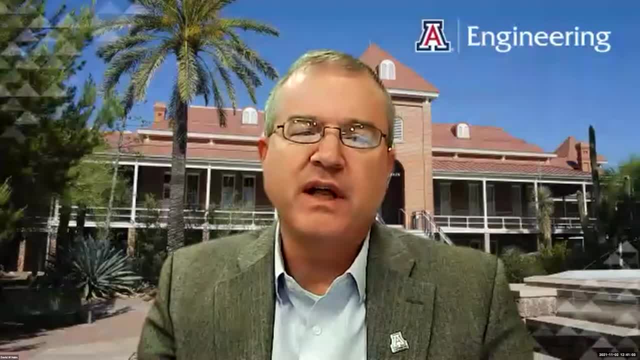 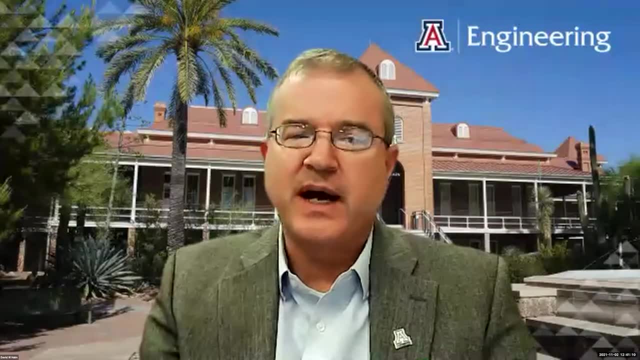 pull out your crystal ball and, let's say, 10 years from now, do you feel like you know you go to your physician, you have a blood draw? do you feel like, say, a decade from now, they'll be able to extract some pretty useful diagnostics around cancer? early detection Is. 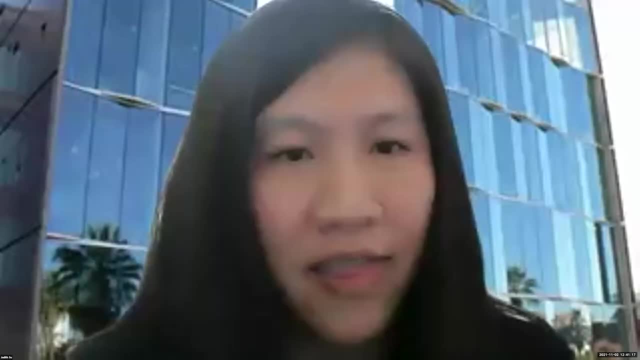 that the right timeframe to make a lot of progress? I think so. I think companies are even doing this now, where you know you can take blood and you can send it out to be, you know, sequenced and stuff. Yeah, That's great. Jong-il, are you working at all in the? 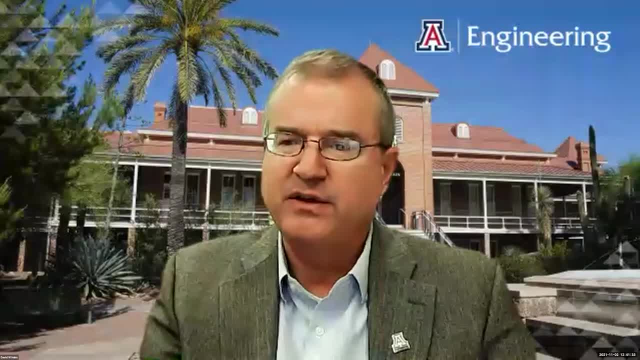 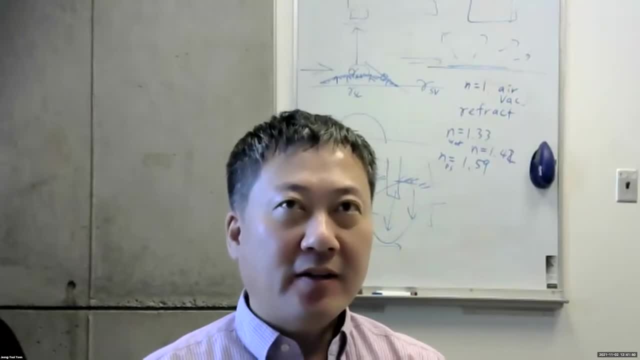 cancer space And is that something that your technologies could have some applications? Yes, Also I work on cancer, but I'm primarily interested in the circulating tumor cells from blood and then also the- you know, the blood cancer. So I'm very interested in detecting 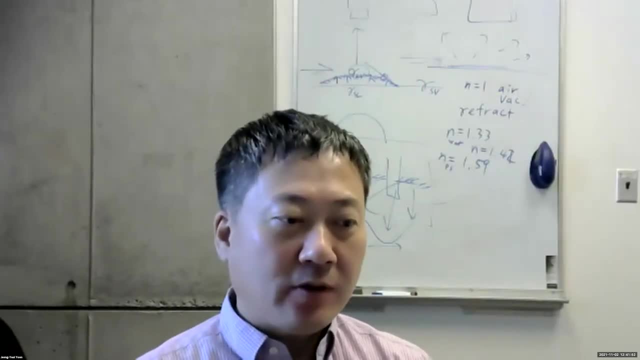 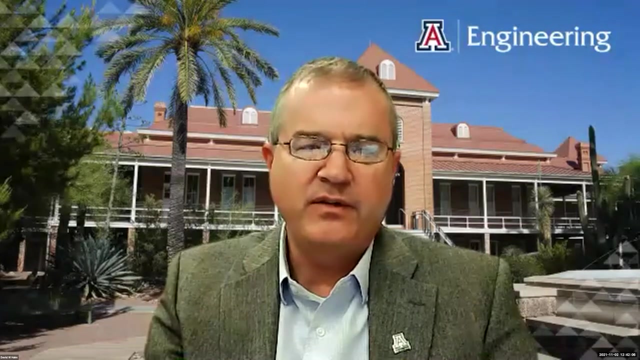 the cancer markers from blood, And it's all based on either the antibody-based assay or, you know, I can also do the PCR-based gene amplification. So I work on both Excellent. Thank you both. I'll stick with you. Jong-il, It's increasingly common for people to use Fitbits. 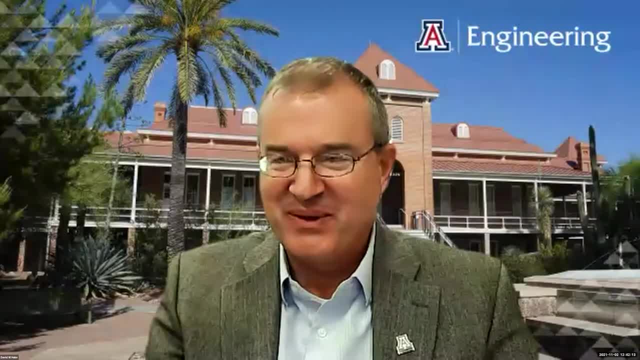 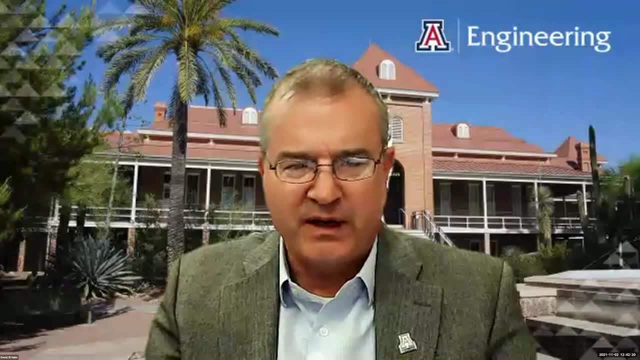 Apple Watches. You know it seems like the commercials are nonstop with the new Apple Watch about monitoring your health. Are these kind of wearable technology opportunities? can you leverage that into some of your own research interests with? you know small sensors and those types of things? 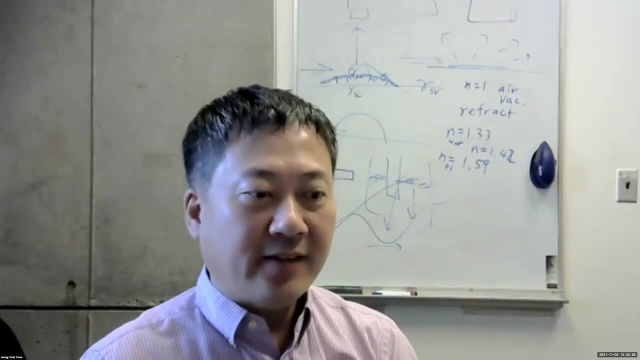 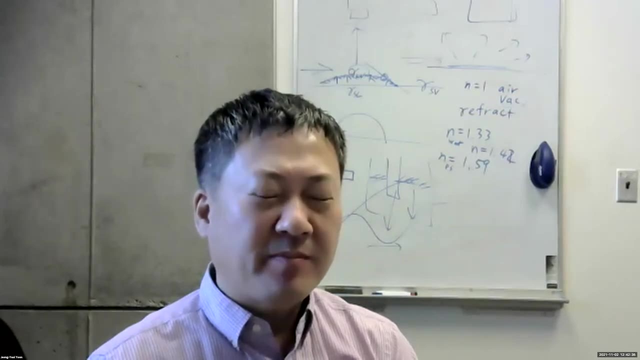 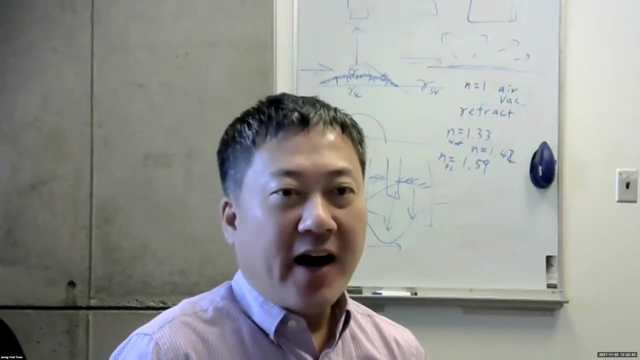 There are a lot of other people out there utilizing the accelerometer, GPS and gyroscope And, in the first, monitoring the system towards activity trackers. many commercial apps and commercial devices are already wearable. What I am interested in is that they do have the image. 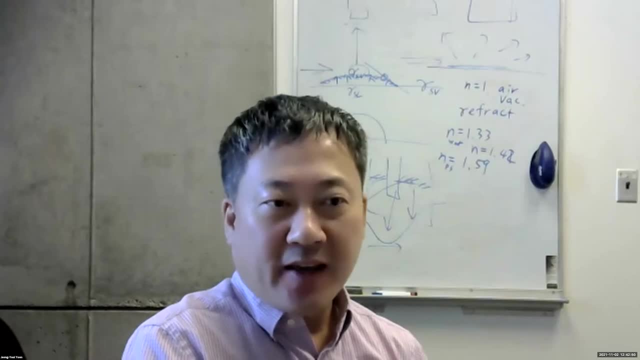 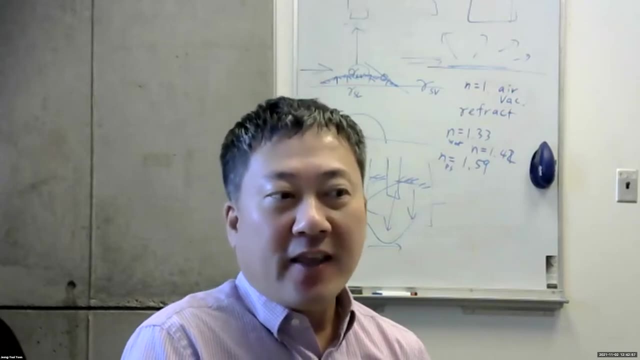 sensor. So basically they take the image of something and then show its coloration in three different colors: red, green and blue RGB. But what if you can construct the entire spectrum, So not just like three colors, but 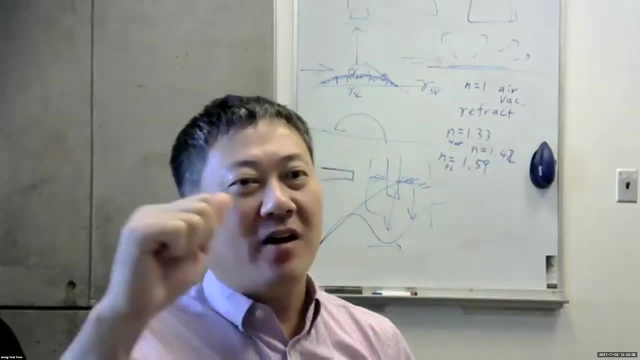 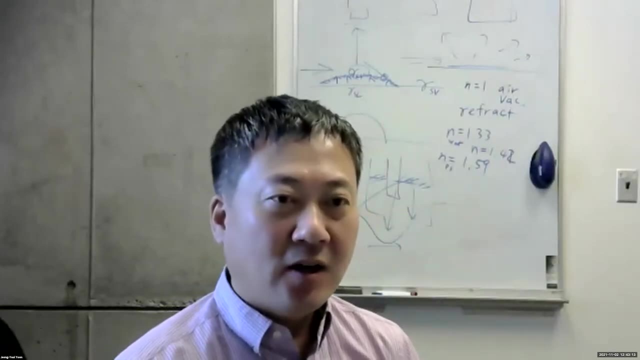 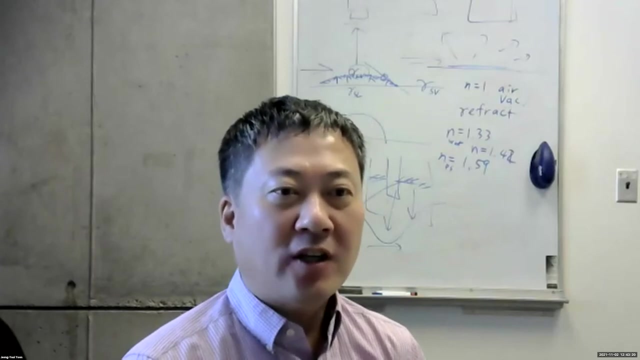 100 nanometer, four one nanometer, four, two nanometer, keep going on and then calculate, establish a spectrum across the entire wavelengths of your visible light, or maybe well into the UV or near infrared as well. So if you do that, spectroscopy for the entire imaging. 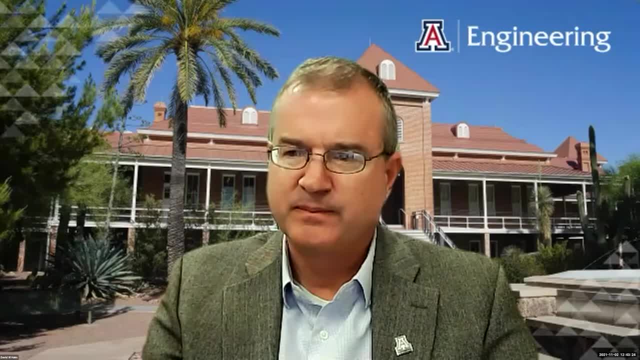 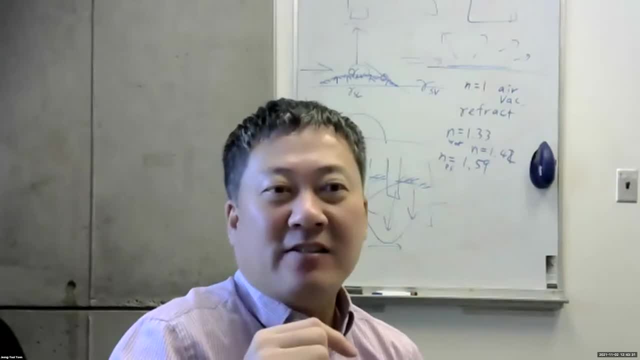 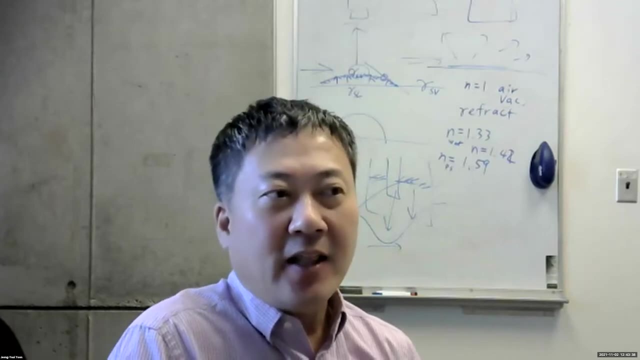 that becomes a hyperspectral imaging. Sure, And I really want the smartphone companies, to you know, enable that spectroscopic analysis or maybe either hyperspectral or multispectral imaging capability, and if we can make that happen, then everything will change. We can detect the presence of bacteria from your table. 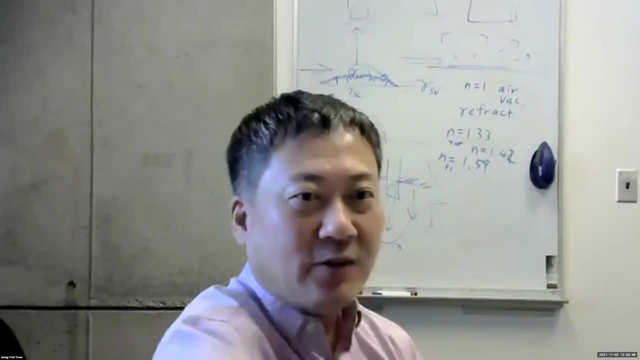 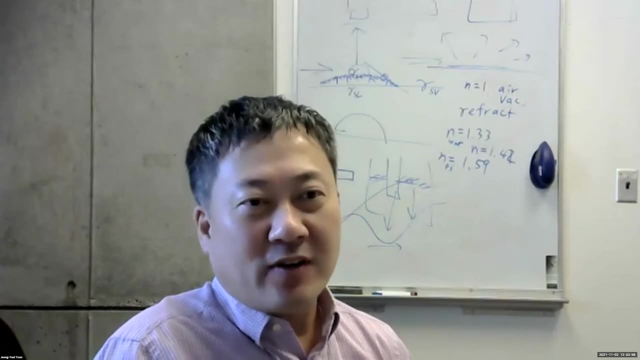 from your toilet, from your kitchen. just scan it with your multispectral imaging device And then scan it through, and then it may tell you you have some pathogens out there And most likely it's some dangerous pathogens or it's less dangerous pathogens. Dr. So is it safe to use spectroscopy with cameras and AR reporting? Dr? So the technology, and now I'm going to talk about you at a little bit, but I'm going to go to the next slide and then I'll get back to Dr Marciano. So the technology and what they're doing is: 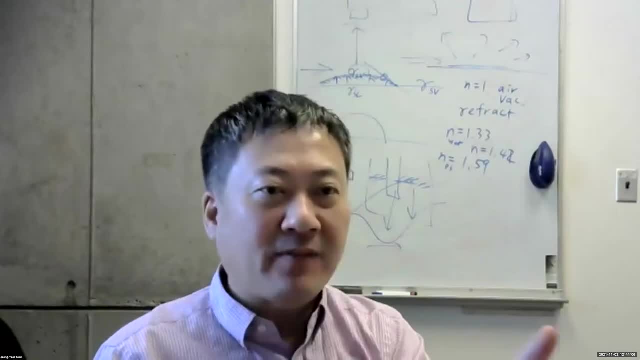 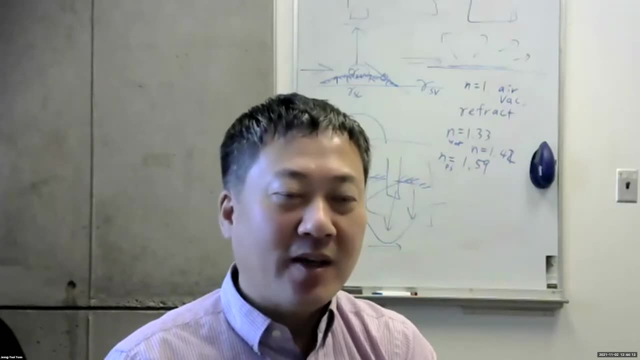 Technology is already out there. It's just a matter of incorporating them into your smartphone And then right now the obstacle is the high price. But if you can mass produce them, it may happen. That's great. That's some really promising new avenues right that could open up. 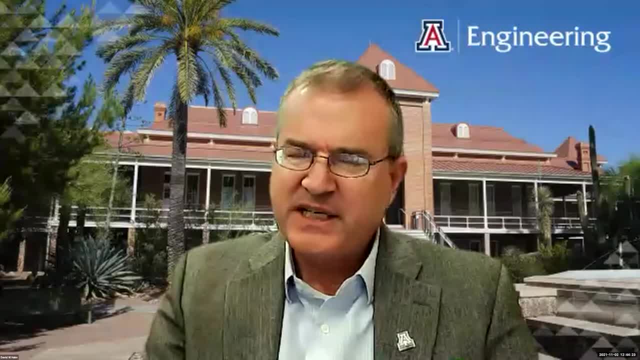 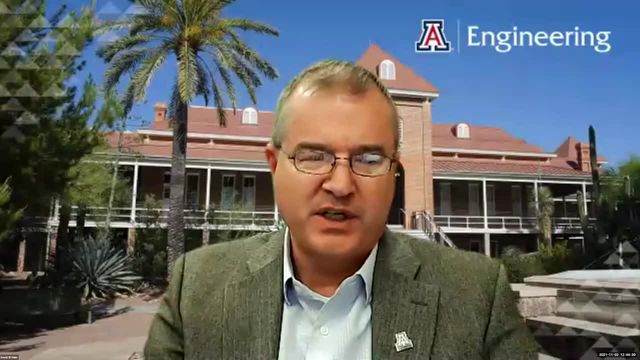 So that's great. Let me kind of come back to both of you, to our educational mission, just a little bit. So you both had interesting careers and some really exciting research. You know, Judith, you've got engineering training and biochemistry training. 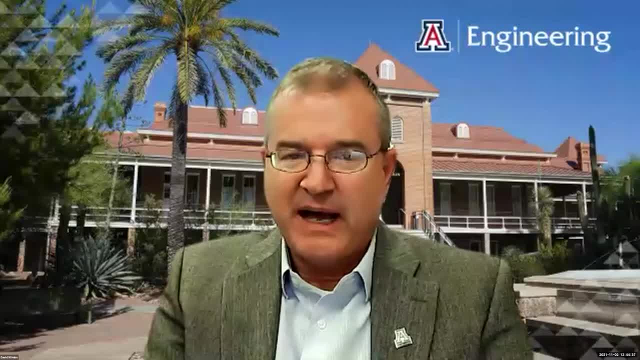 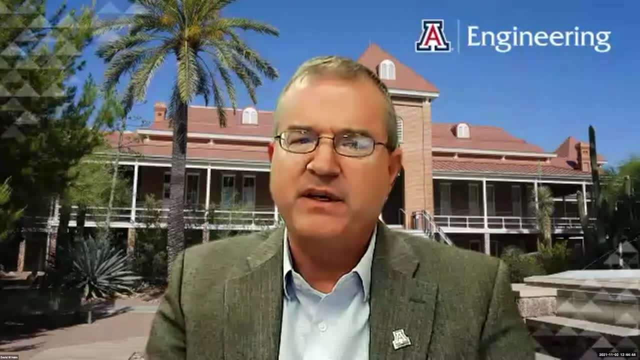 What are some takeaways from your professional life and career track that you would share with engineering students that are listening or will listen to this in the future, that might have an interest in health care, and kind of maybe give them some takeaways that could guide them to contribute in this area? 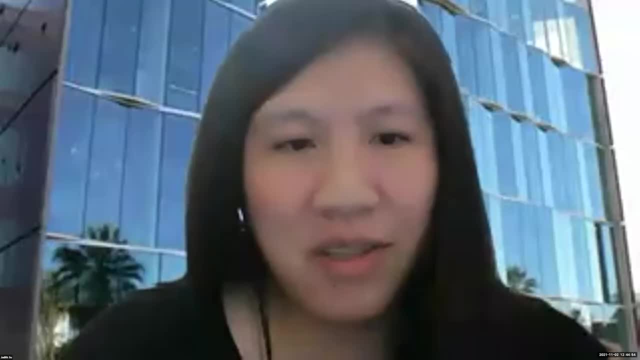 I'll go with you, Judith, and then to Jong-Yul. For me it's really been that the future is really unpredictable, So it's been really hard to predict what would happen in my life Six months from now, one year from now. 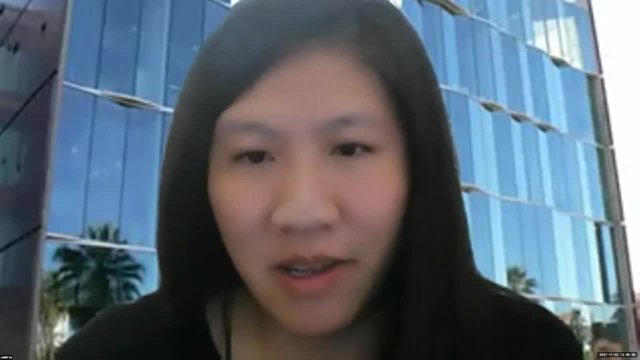 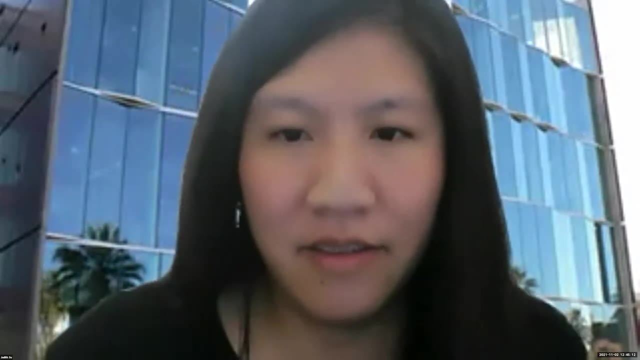 So I would just be really, really flexible and be ready to catch opportunities when they come up, And I would also really encourage tapping into the alumni of your college. So, for example, College of Optical Sciences has this huge industrial affiliates program which has a lot of alumni. 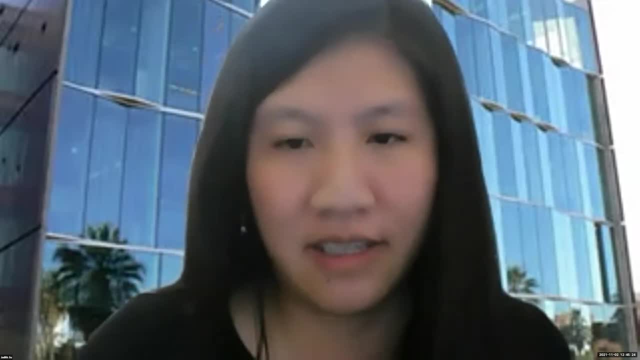 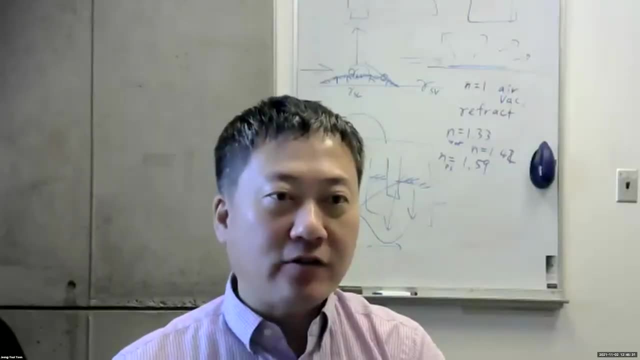 And they've been really helpful in terms of finding jobs, providing career advice, et cetera. Excellent. So, Joni, I would ask- I always ask my undergraduate students to participate in research activities and regardless what their career goals are. 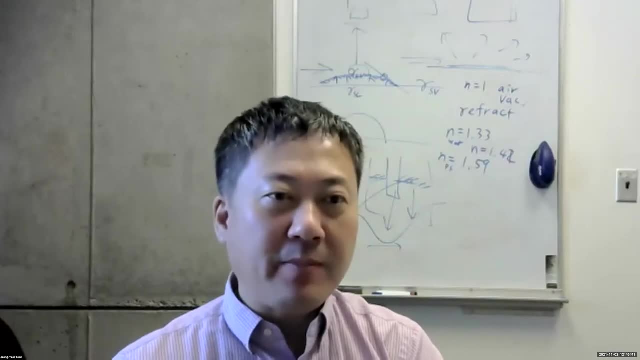 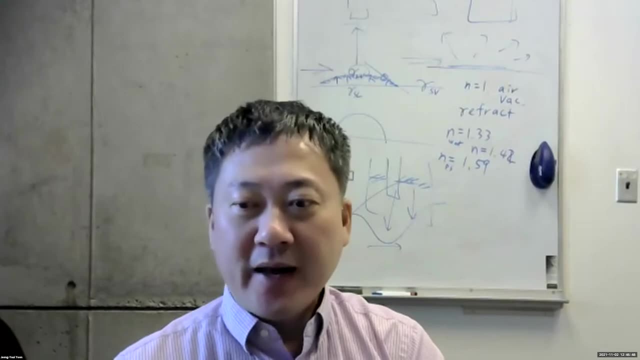 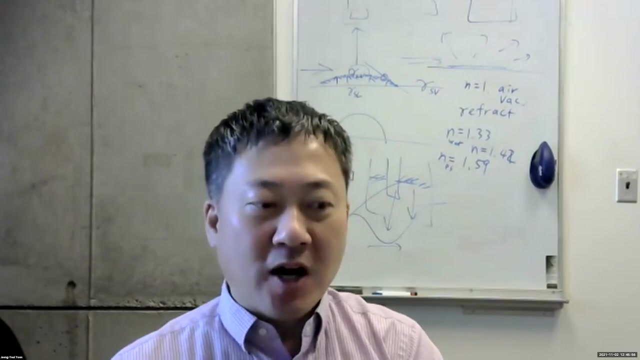 So many people think that the research training is primarily for the students interested in graduate program or medical school. Not necessarily. I have found many of my undergraduate students successfully finding the job they want in the relevant discipline with the high-paying job. So the research experience is quite important for undergraduates. 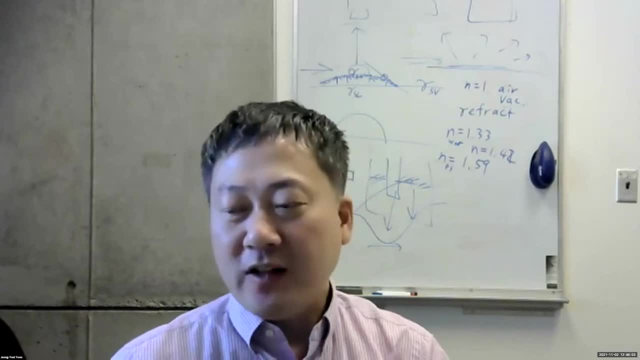 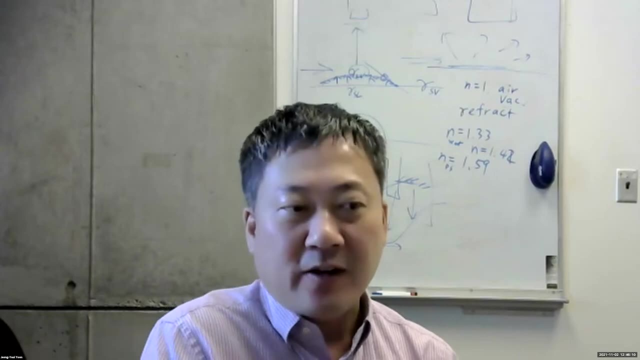 And I think it's really important for undergrad students to get better prepared. it's very different from taking classes and then taking- you know they get a good grade on your classes, but just to participate in their ongoing existing project as a team player. 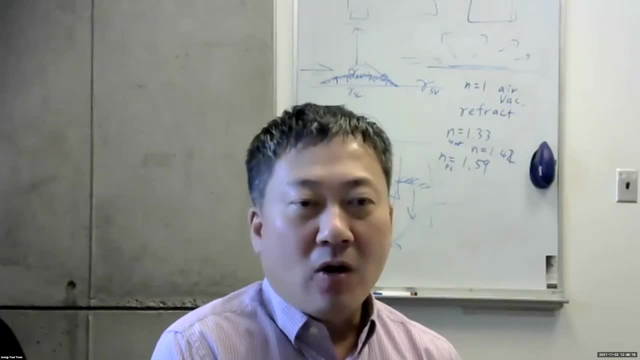 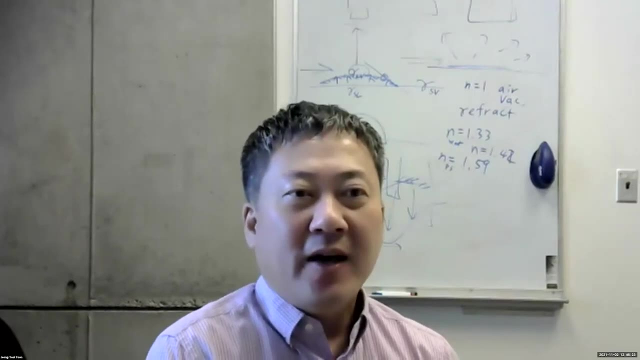 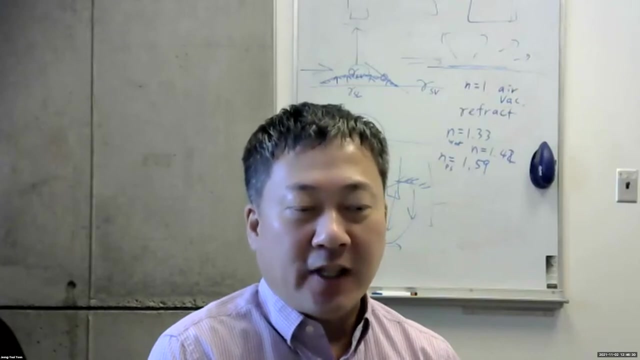 And I also strongly recommend all undergraduate students to participate in the internship, industrial internship over the summer, And there is also the research opportunity in the other institution as well. So they utilize all of their time. So they utilize all of their time, All those opportunities, then they can be better prepared for their future. 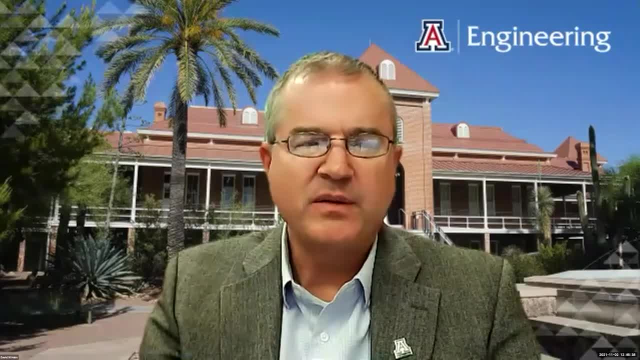 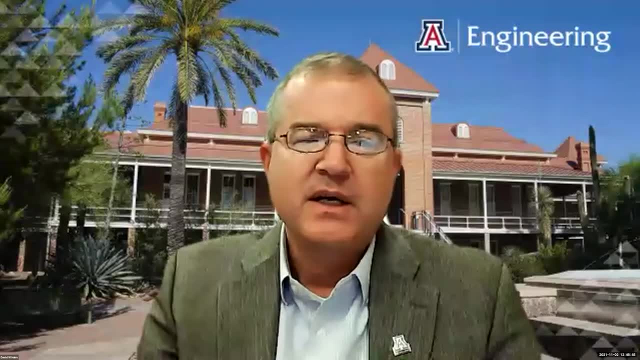 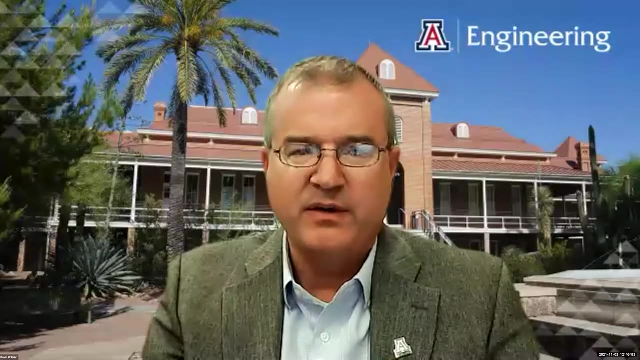 successful future career, Excellent. I'm going to go back to my kind of opening statement about the dollars associated with healthcare, the 17% of our GDP. Do you believe that your approaches can make a dent in the healthcare costs through some of the things that we've talked about? 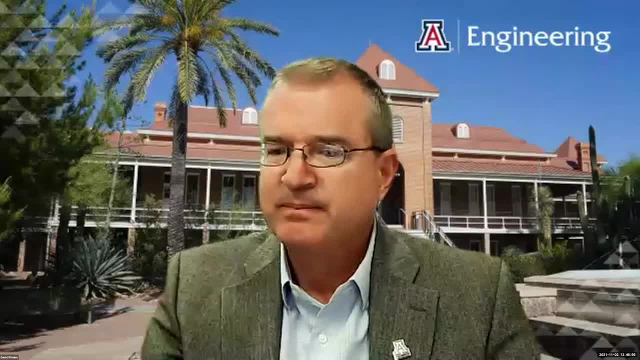 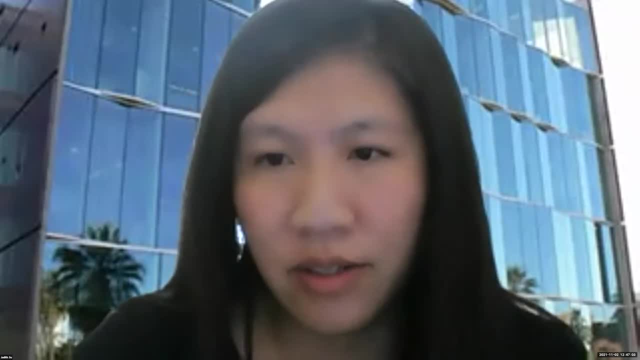 I'll go to you, Judith, and then to you, Dongjoo. I think, definitely, I think a lot of times. I think a lot of times things that we can do in healthcare can help reduce our health costs. So I think a lot of times what I can do can help reduce some of the health costs that we 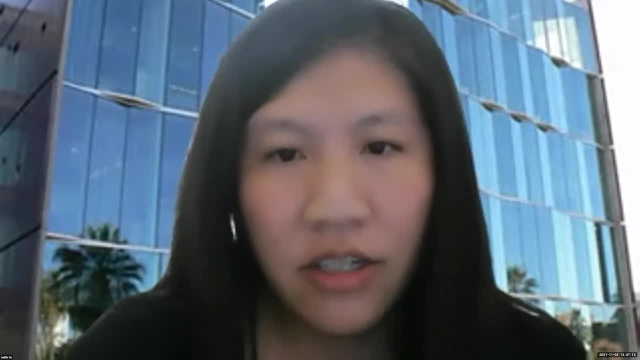 can have And so I think so that's a little bit more of a visual look at that. I think that's, you know, a way for us to be able to try and offer sort of anytime in the future to do it. Yeah. 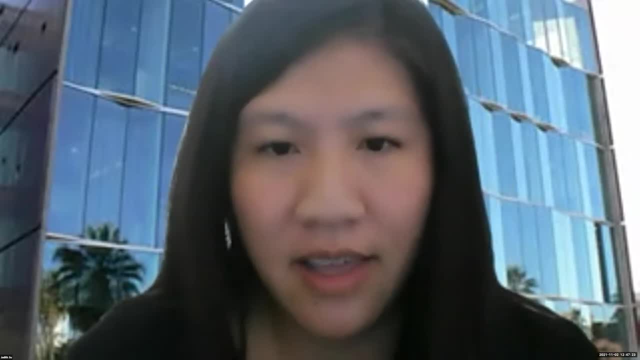 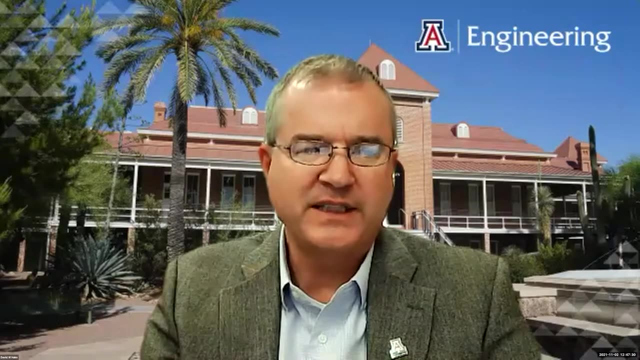 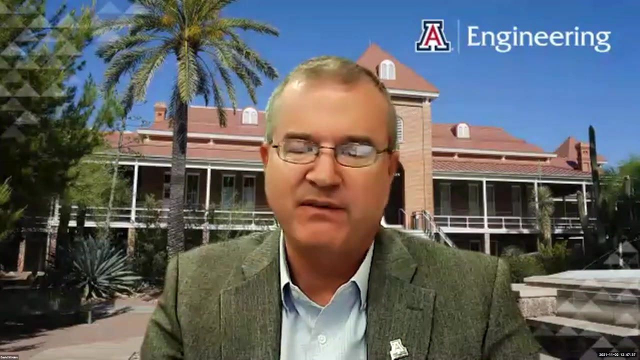 All right, Do you want to add to that? Yeah, I'll go ahead and do that. And the first thing is we have to keep in mind whether we're doing something that's positive or not. positive, Right, Yeah, Yeah, low cost testing, And I like what you said about early sort of detection or waiting. you don't have to wait until things get so bad, right, And that can really have a lot of cost savings. Excellent, Jung Yoo, what do you feel on this front? I would say on my own experience, because I have a lot of medical conditions And so the but I receive a letter from the insurance company all the time. you know they do this test, do this test, And then they're doing a lot of tests. you know they ahead of time, basically saved insurance companies money and otherwise they wouldn't do it. 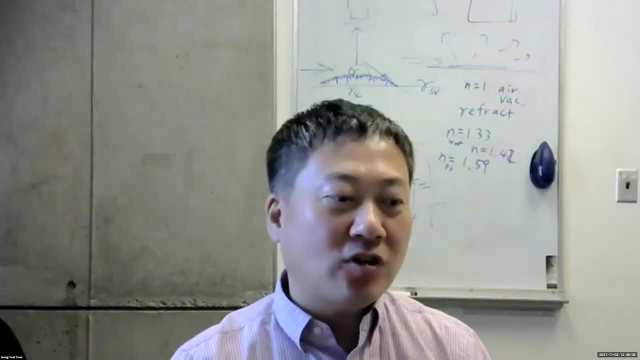 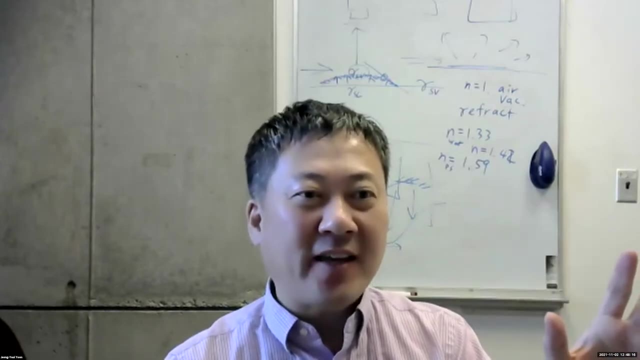 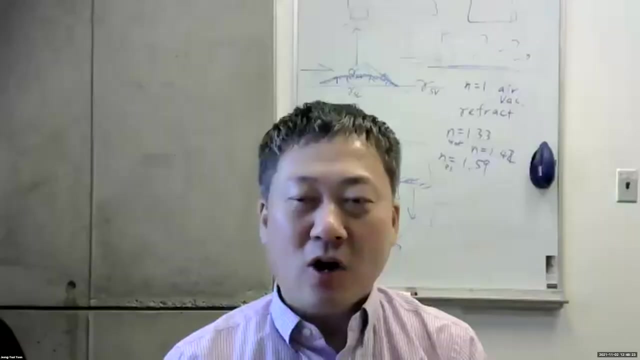 But the problem is this: when they asked me to do certain tests, and then there are tests that can be easily covered by the insurance, but there are other tests that is not covered by the annual checkup. Okay, you clearly see the difference. Yeah, then insurance companies trying to ask all of you to get tested. 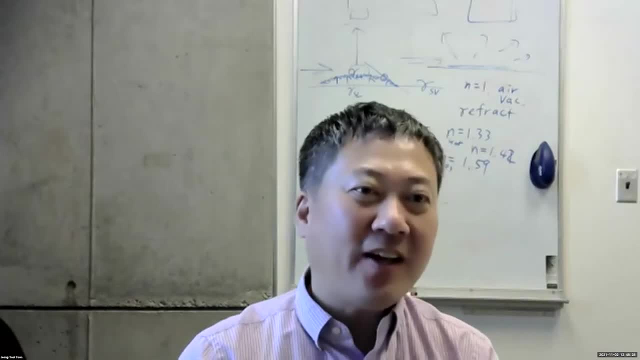 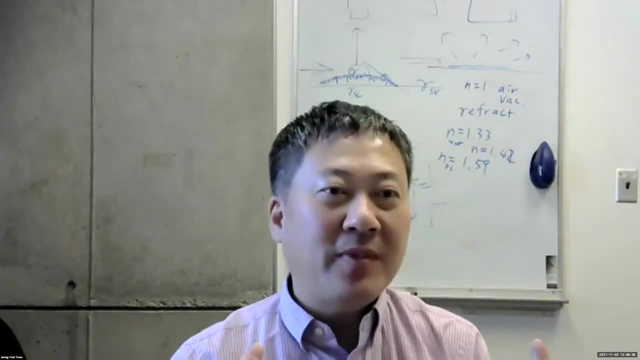 But you know the cheaper test only. So if we can lower the price of that you know the diagnostics and then make this kits test available to everyone, that's going to dramatically the lower you know the cost of the medical, the healthcare expenses. 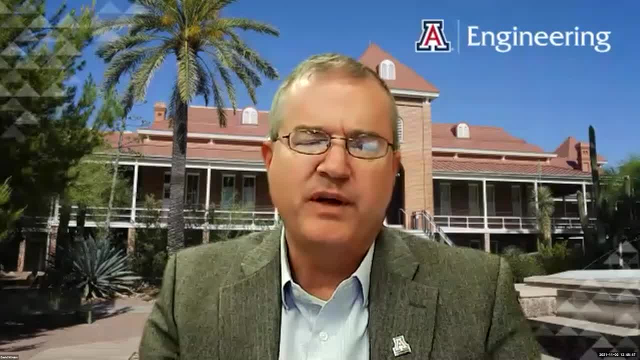 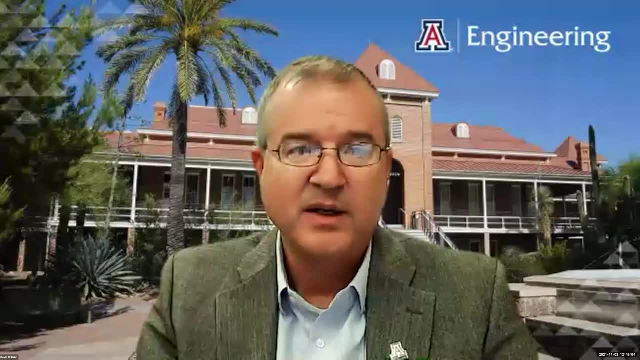 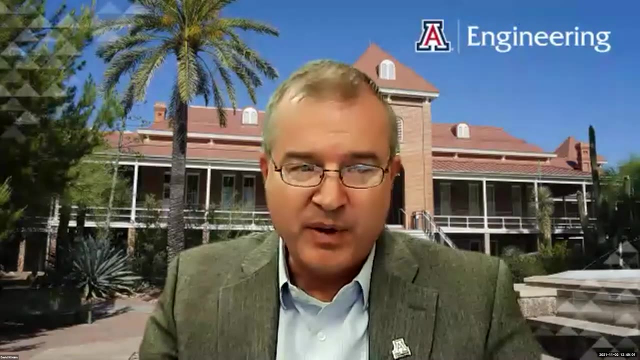 Outstanding Judith, I asked you after your presentation to clarify that you know was your device actually going inside the body? and you confirmed for the mouse trial it was not, But to both, both of you. do you have any future plans that you might incorporate some components of your sensors actually inside in vivo type sensing and 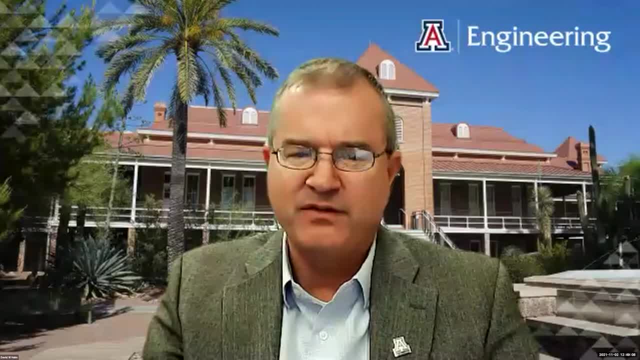 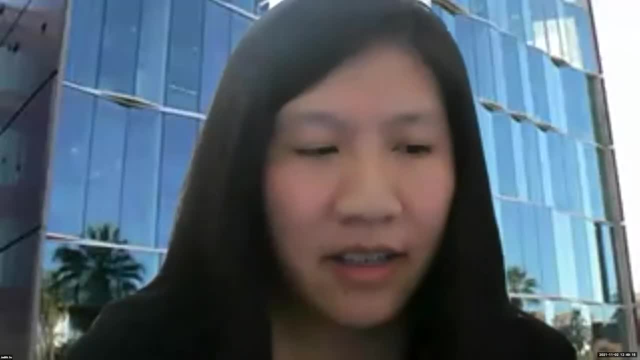 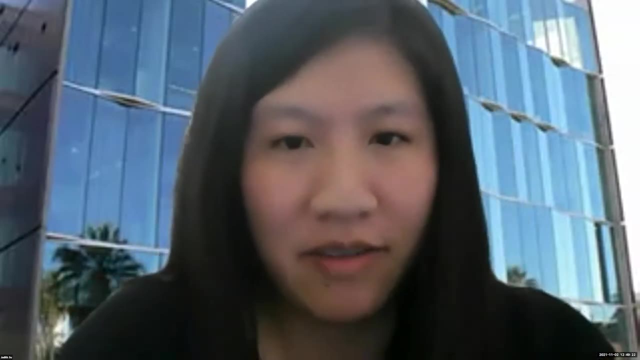 I'll ask you both to share any thoughts on that subject that somebody asked. I'll go with you, Judith, and then to you, Jongyul, if you have anything to add to this topic. Yeah, so I actually had a student that was working on this for a little bit before she got pulled away to do other projects where, yes, we were. we are interested in sort of developing these sensors to go inside the body. 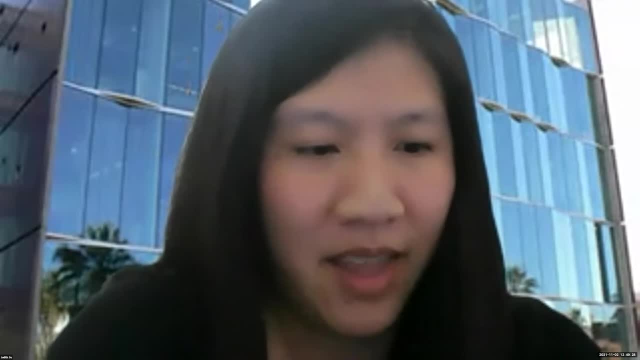 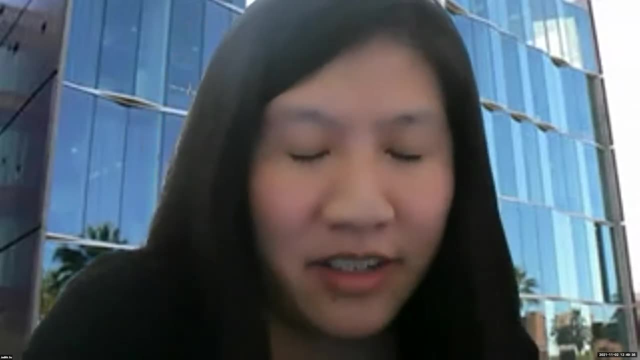 And, of course, that has to take a very, very different form, And you know we were interested in incorporating essentially little nano lasers inside the body to create sensors, And so that that is an area that we are actually very interested in. 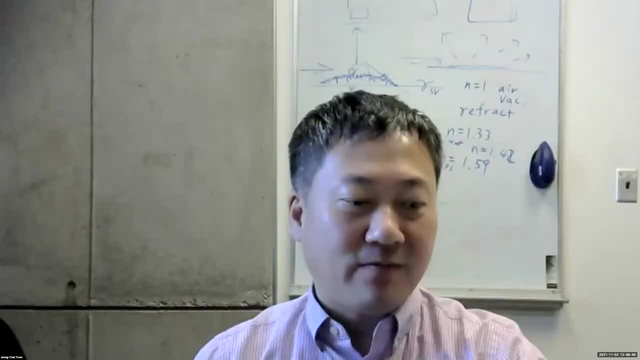 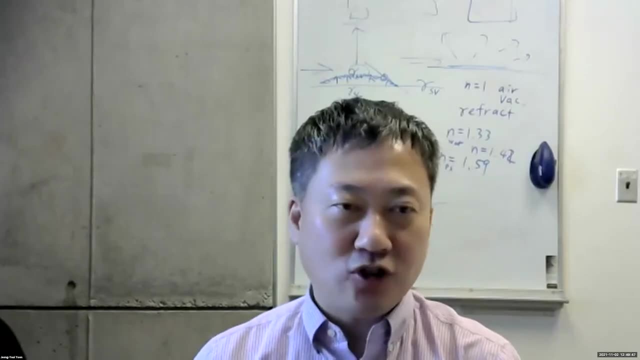 Oh, interesting, Jongyul. And then, frankly speaking, you know, the inside of the body is not really my expertise, as you can clearly see, but I am interested in attaching those sensors to the skin of your body so it can actually read your signal. So a good example would be the sweat sensor. 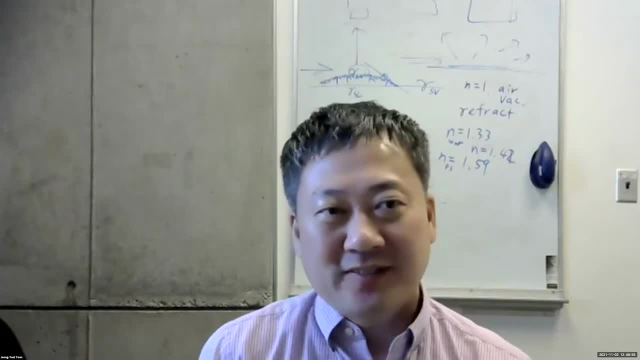 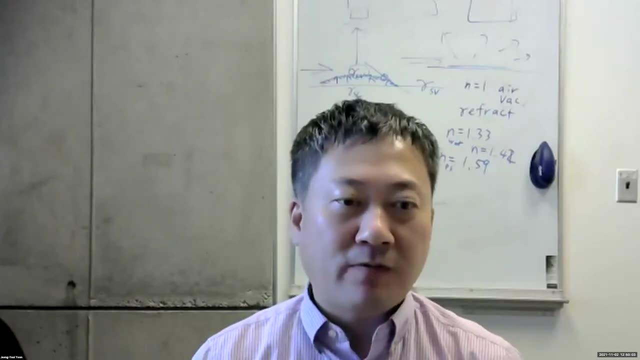 So it can actually read your signal. So a good example would be the sweat sensor, So the rather than analyzing your saliva or blood or your urine, but you can collect your signal from your sweat And then that could be considered as either the in body sensor. 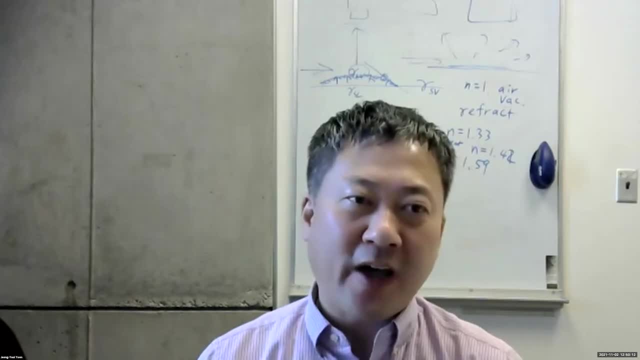 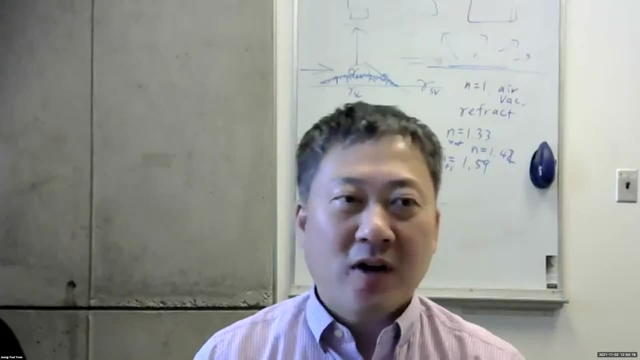 So that's the part I'm also interested, but we also have other players here at U of A who works on the sweat sensor is primarily geared towards glucose sensing, But I'm more interested in the more complex molecules. Excellent, And Jongyul, I'm going to stay with you for a second and pull a question out of the 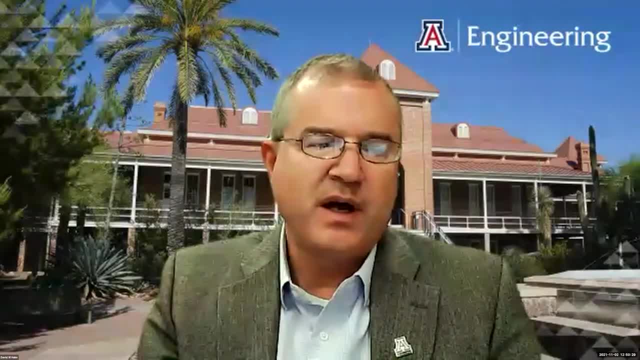 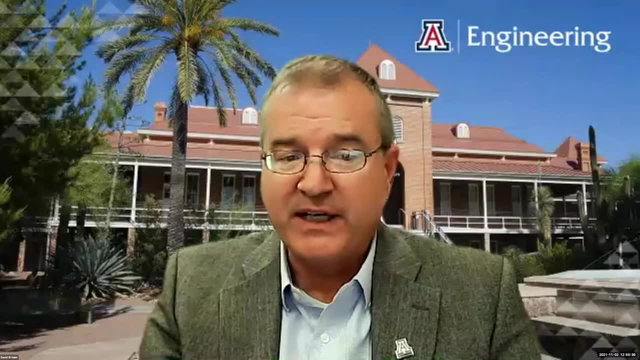 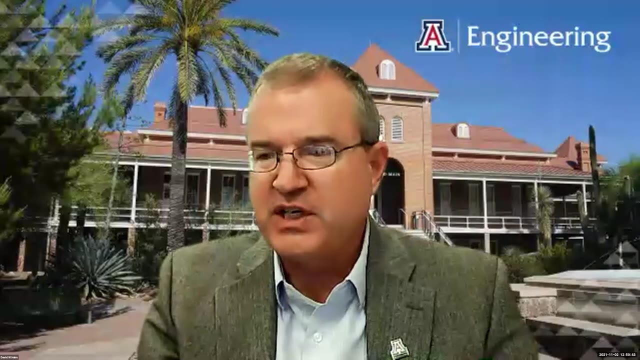 It was just submitted about. you know your devices and your machine learning to look at wastewater, for example, following UV disinfection. So I guess the question they ask is: can you differentiate between inactivated and active viruses to potentially assess the efficacy of disinfection or those types of applications? 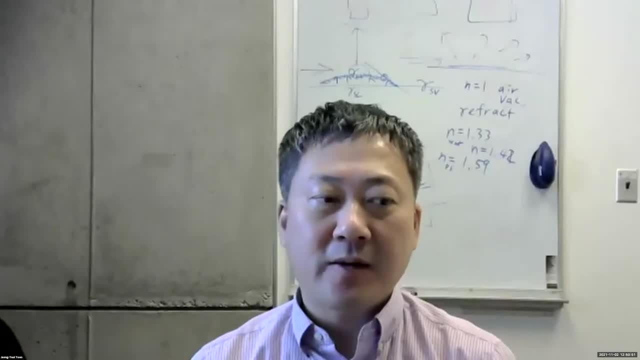 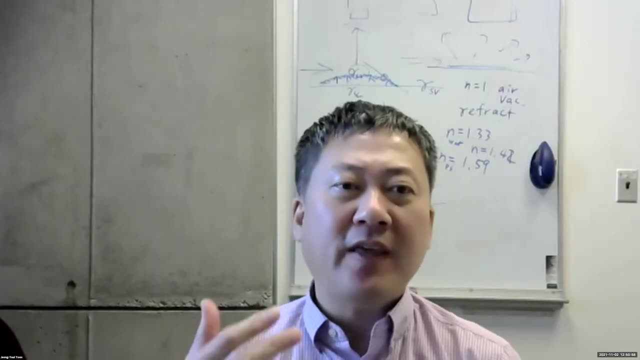 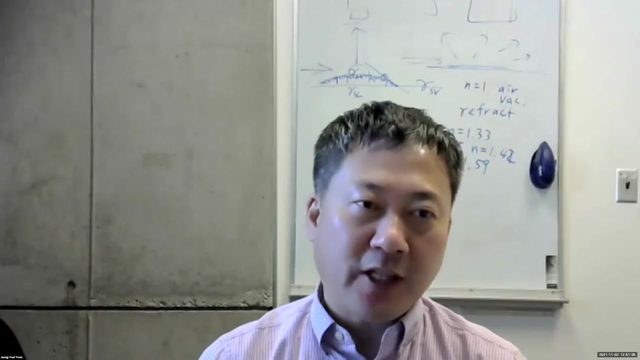 Unfortunately no at this time, because you know, it's all based on the interaction of my certain specific chemicals or peptides with the surface antigens, surface proteins of the bacteria. So we cannot really tell whether they are alive or not. So that's the limitation. 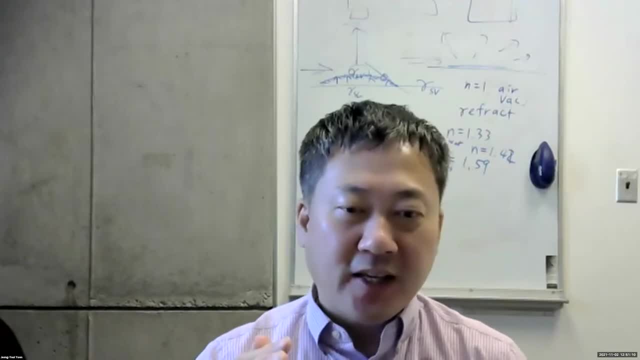 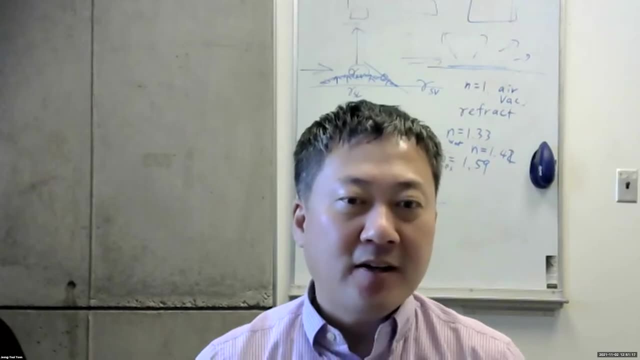 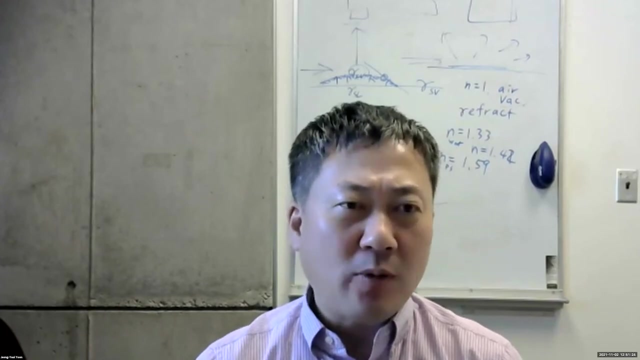 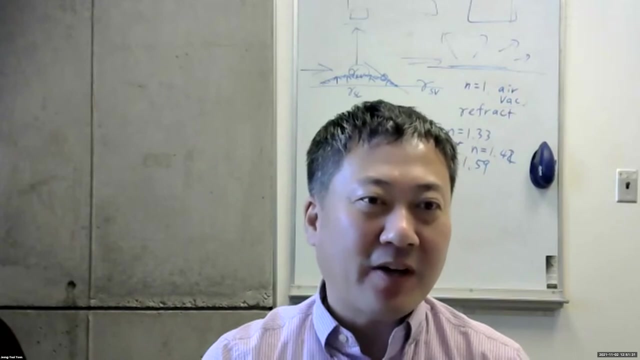 But we do have other methods based on the more sophisticated antibody assay or more sophisticated PCR assay, nucleic acid based assay. So this is more Like a preliminary screening tool, that you have something and and then we want you to further develop it. But you know the the having, and knowing what you are looking for is very important, because if you do not know what's in there, you need to test it like hundreds of different subjects. 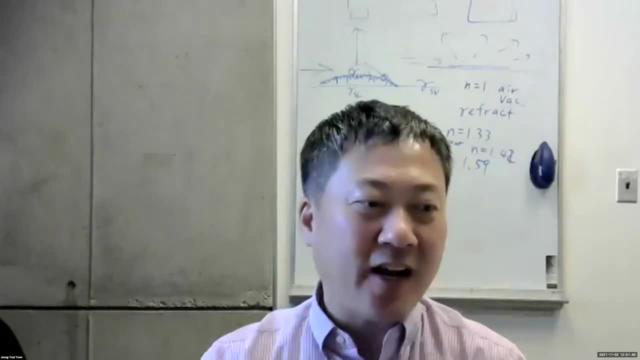 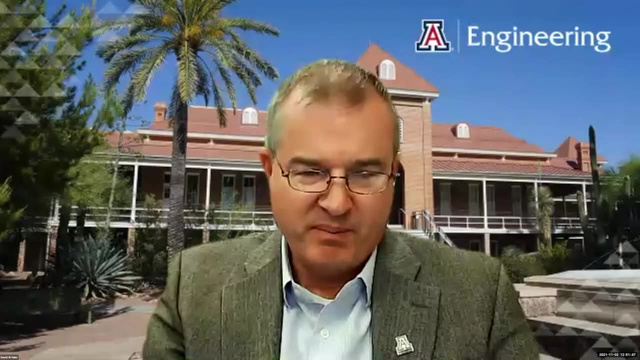 And you don't want to do that, But this machine learning technology will tell you most likely you have this or that. I want you to further test that on these two Gotcha, And I'll just stick with you for a moment and pull one. 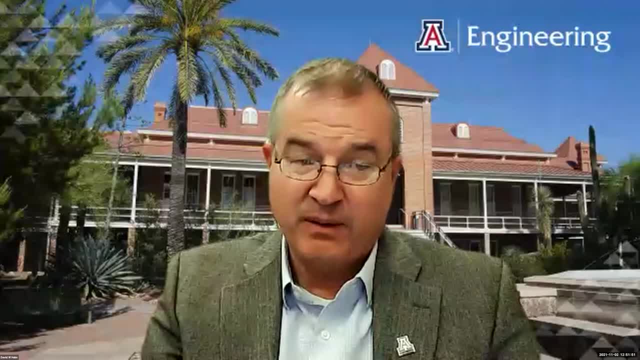 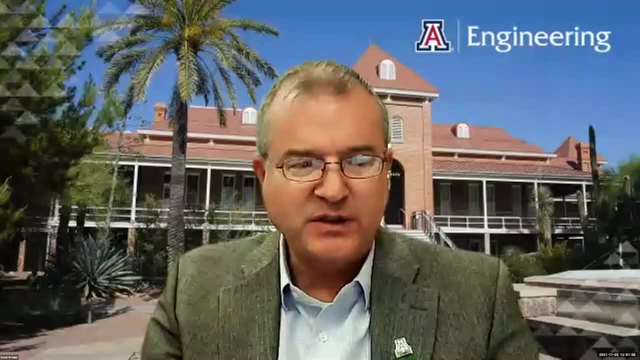 I have one more question in real time. Someone asked that they've heard that some firms are already meeting with the Food and Drug Administration on using smartphones and apps. Have you had any exposure to those companies and working in that space and any thoughts to add to that question? 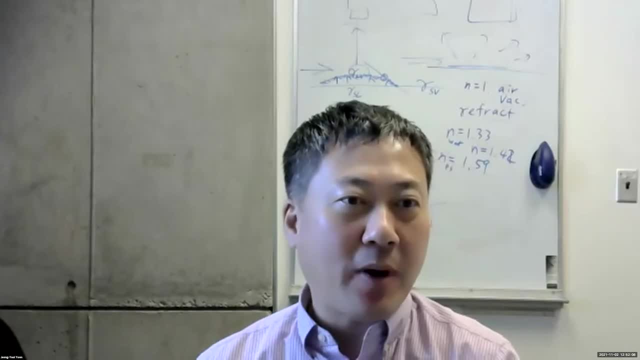 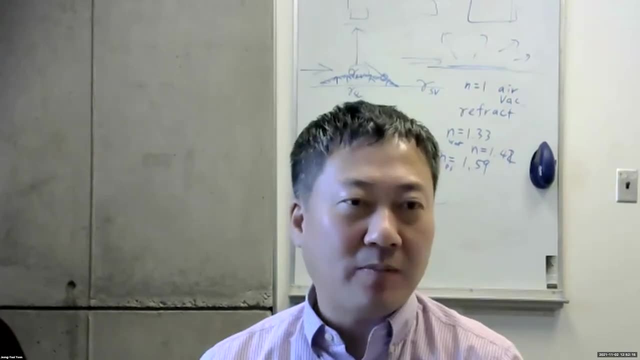 So actually that the, the smartphone reader device that I published in 2013, has been licensed out to an external company, and then they have gone through FDA clinical trials in the past couple of years. I think their product has come out on the market. 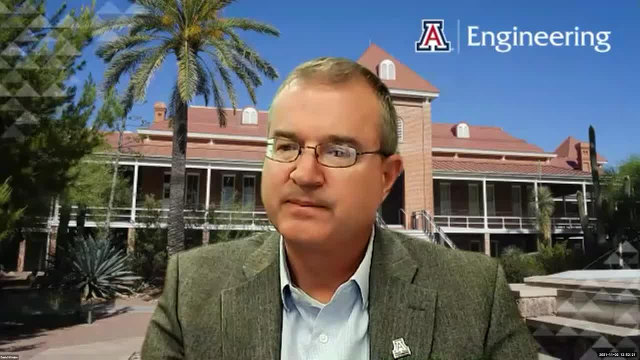 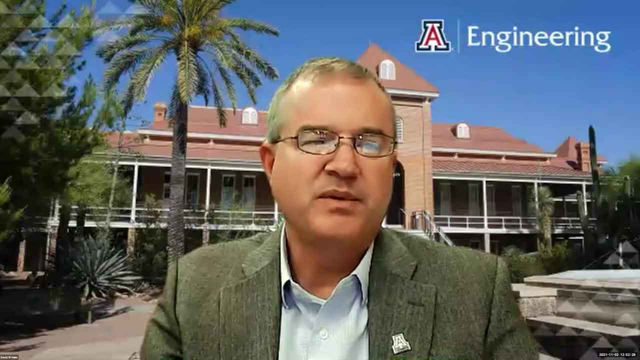 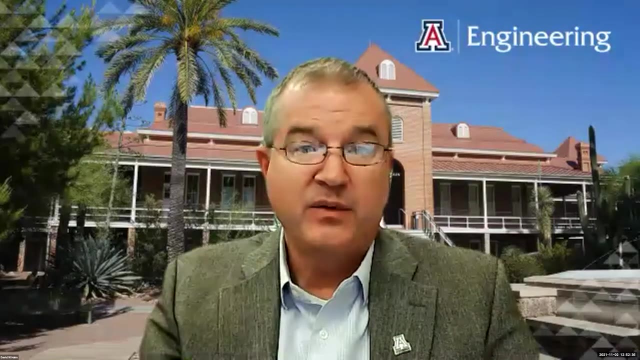 You know, the last year or something- Wow, I have some experience with that- and that they are not the only one. of course, That's outstanding, You know. again, I'm going to take this back to education for a minute, because our graduate research program is a very important part of this college and the recruitment of top students is paramount to the success of our graduate programs. 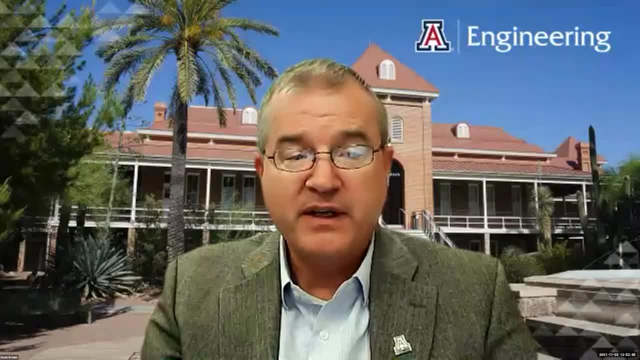 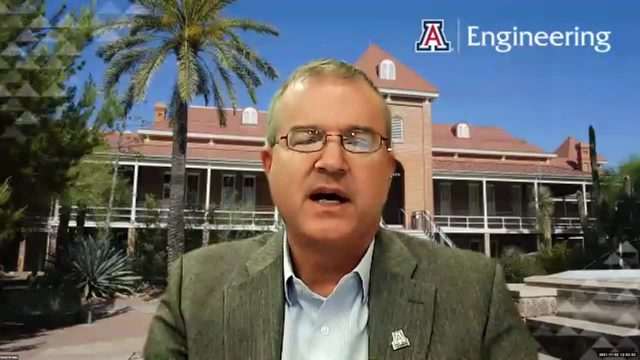 Can you both comment on the specifically sort of the attractiveness of your work to help industry? How do you recruit students? Is this a magnet? Do students really want to work on these things? So I'm going to start with you, Judith, and then I'll go to Jong-Yul. 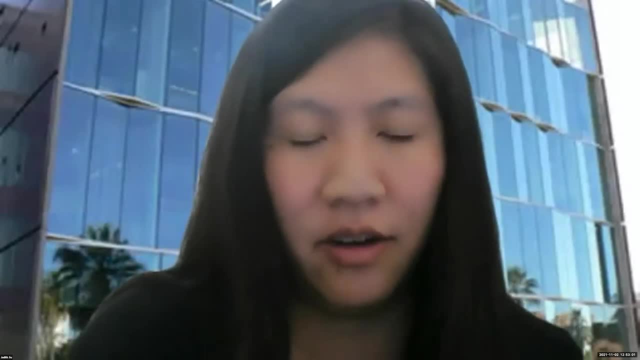 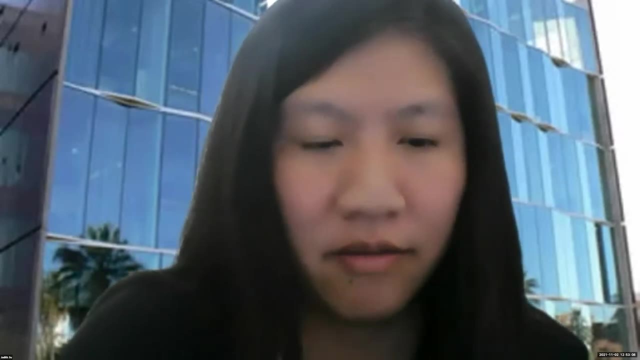 Yeah, I've certainly found that many students are particularly interested in health care, you know, making an impact on people's lives, And so for them, you know, the application of technology to health care is a really attractive field of study, And they always want to know, like you know, what classes they need to take to be better at this and how can they get involved in stuff like that. 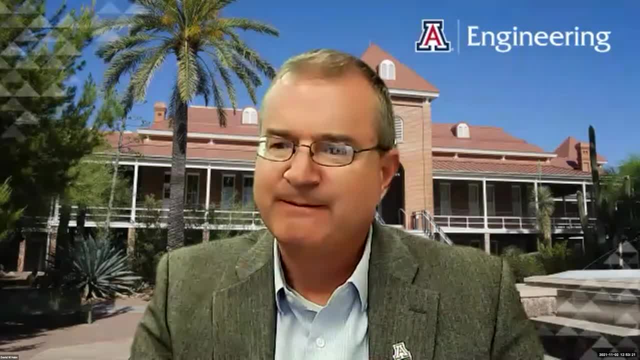 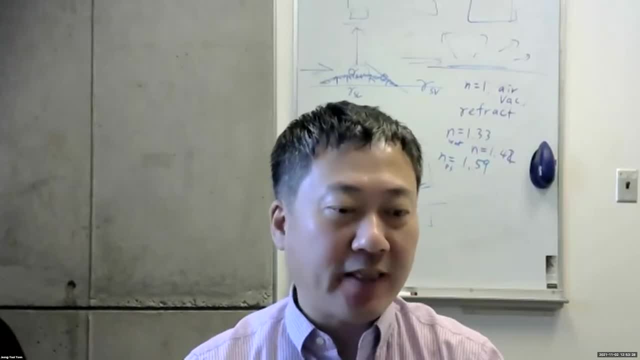 Outstanding Jong-Yul. what's your experience, Ben? Well, if you do, you know the impactful walk and then, if you publish, continue to publish, and then you figure out the proper media attention. students are the ones who know the best actually. 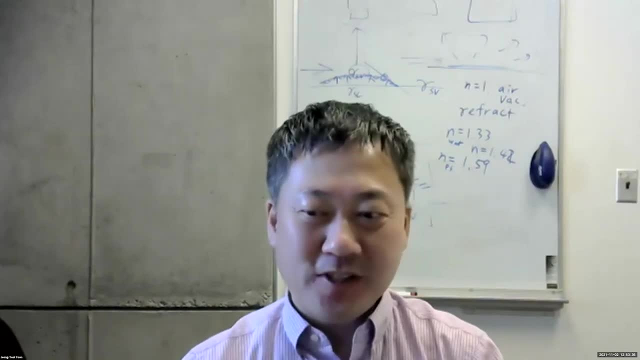 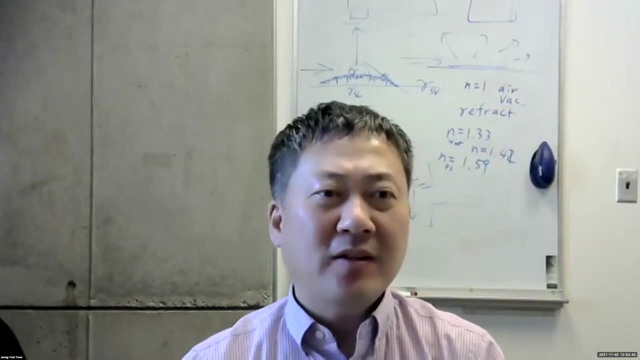 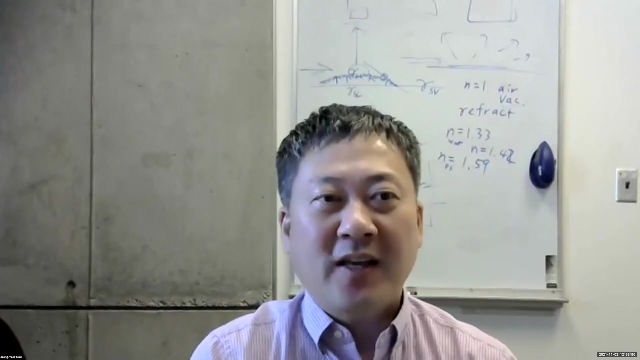 They are quite smart and you'll be quite surprised, And so if you do a great job, then you usually have no problem in recruiting high quality students. The downside is, maybe the little bit of limitation would be recruiting students Internationally or recruiting students from the other side, other part of the nation, like, for example, from Massachusetts or from Florida. 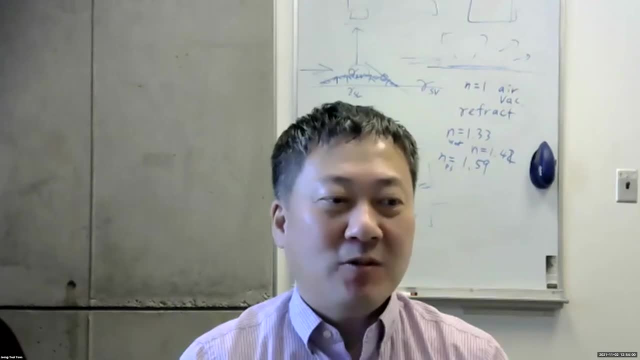 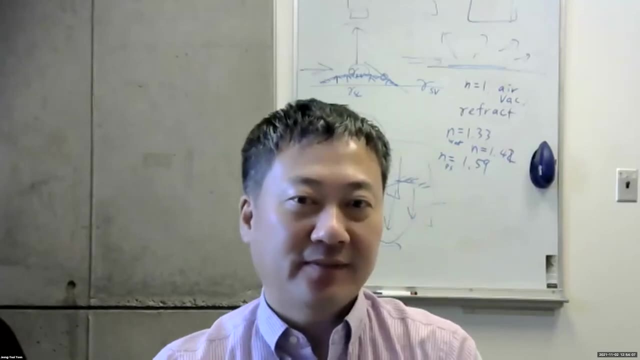 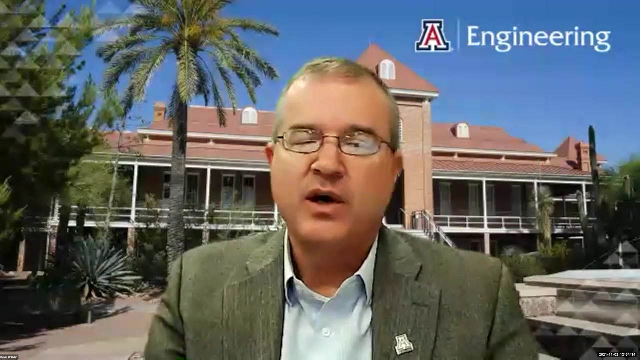 That's. they're so far away. So the day we need to do some the concerted effort to expose our walk to those people out there. So you know, when, when I came here as dean two years ago, one thing that drew me was the co-location of our health sciences, our medical school. 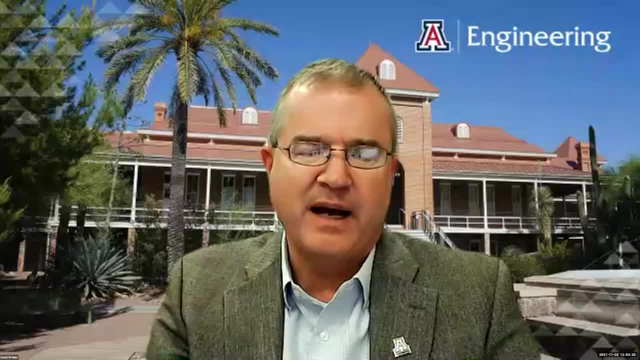 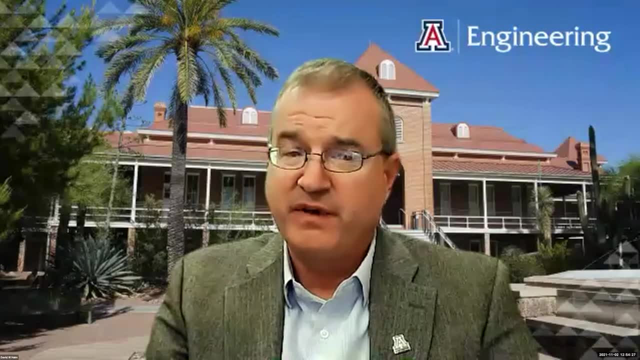 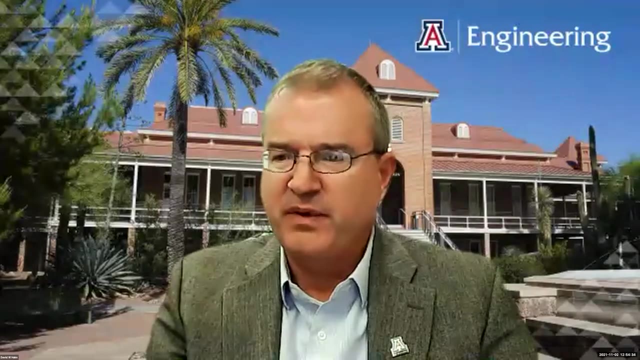 pharmacy nursing and medical school. So you know I'm a big believer in pharmacy nursing right here on the main campus. I'm a big believer in the intersection of engineering and medicine. can you both speak to that year in your experiences, how beneficial has it been to have health sciences and medical school right here and maybe get into some of the details of your specific collaborations with, with our colleagues over in health sciences? 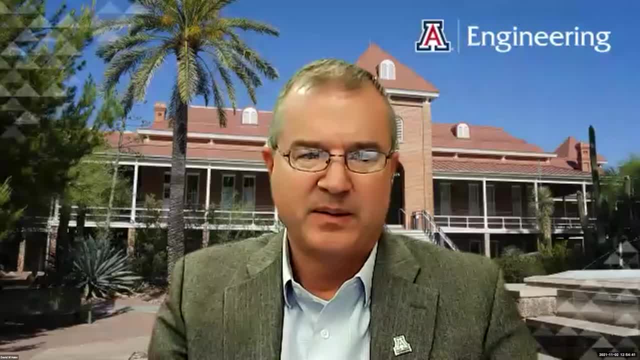 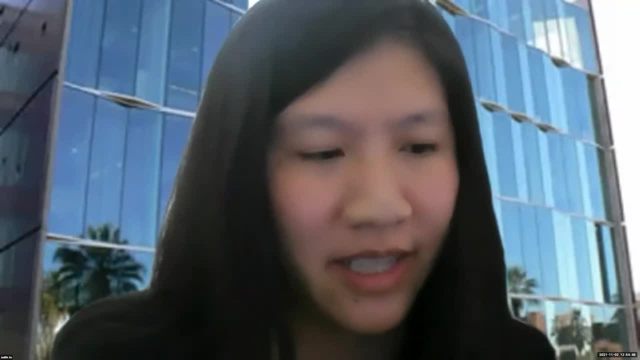 I'll go Judith and Jung-Yul again. It's been really beneficial. So I had submitted a very large proposal- It was like $6 million- to the MSU- And I had been working with NIH recently And one of the criteria was that, you know, we had to be able to detect, you know, 20 different disease types. 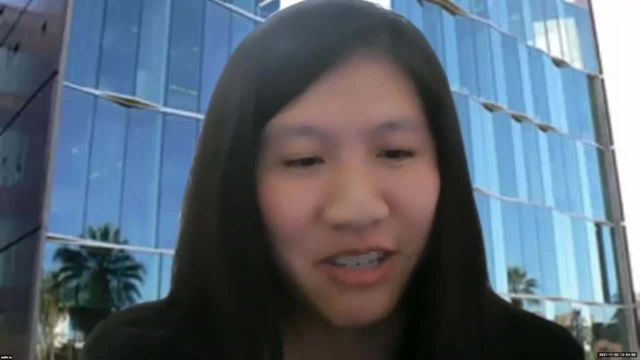 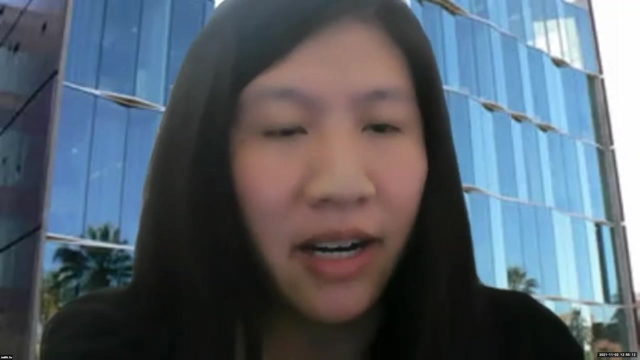 And I was thinking it was like how, how are you going to be able to get that? so you basically- and it wasn't just like 20 different kinds of cancer. they wanted like cancer, diabetes, like a really broad- And I was able to contact people at health sciences and, you know, we were able to get people from cardiology, psychiatry, like sort of every, every medical branch and- and I don't think I really would have been able to do that easily at another place- 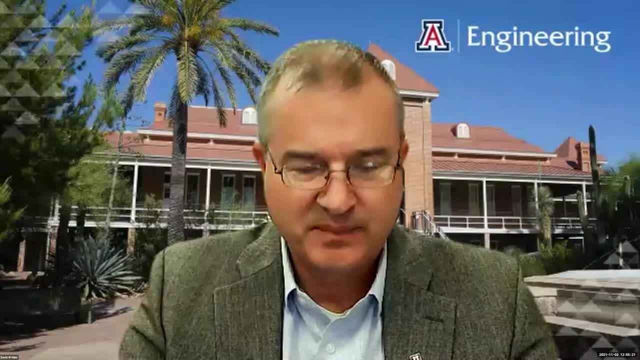 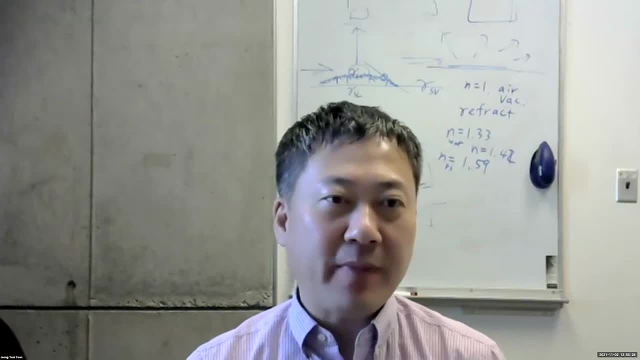 Excellent. How about you, Jung-Yul? The same goes with me, for about, for example, my COVID-19 project, I'm collaborating with the, the two professors in medical school and one in the College of Science, And I am using the student sample collected by, you know, the, the Banner Health. 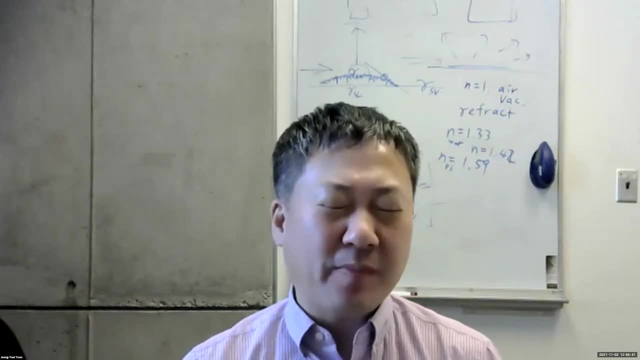 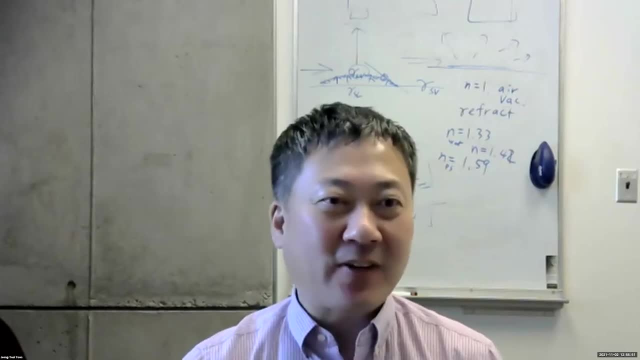 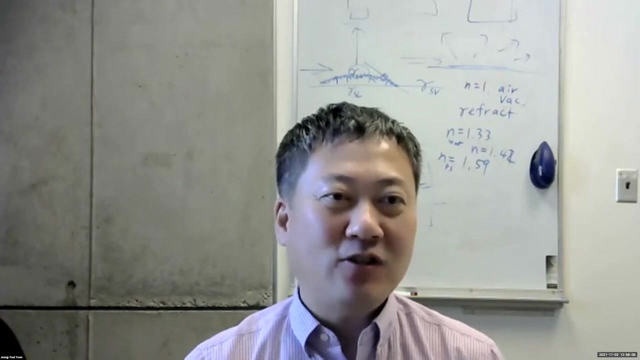 And then we can deliver our sample from their laboratory to my laboratory in less than half an hour- actually it's about five or 10 minutes- And and then we can just even walk our sample from their lab to my lab And it, which is very convenient. but if my medical, if our medical school was positioned in Phoenix, we need to drive like a two hours back and forth. 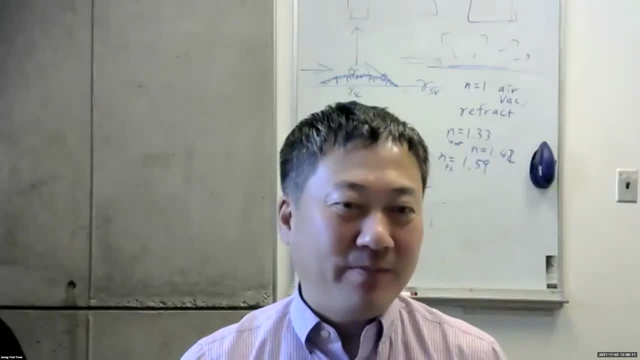 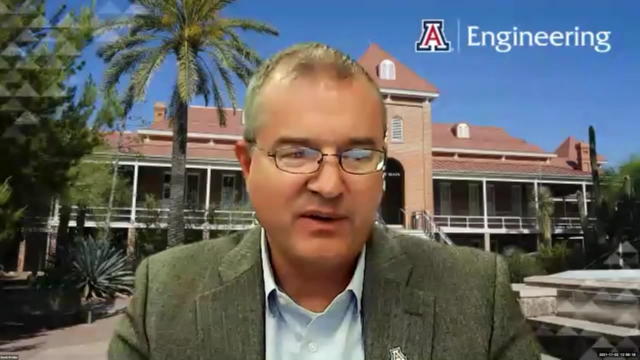 And that's going to be a big inconvenience for all of us. So that's definitely helpful to me. Excellent, That's, that's good. That's a great answer, And that's what I was hoping to hear from you both. Um, so you know we're coming to the end of the hour. 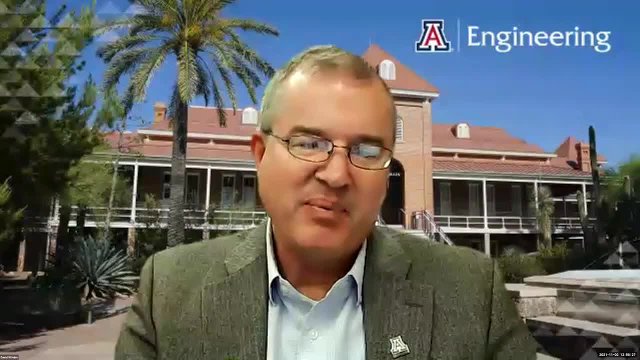 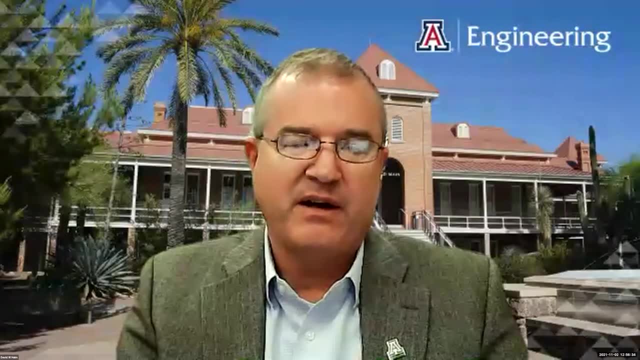 It's been a great conversation. I'm going to give you, you know, each now pull out your crystal ball and look, say, 20 years into the future. What problems do you think will will have solved in this area of sort of biosensing? 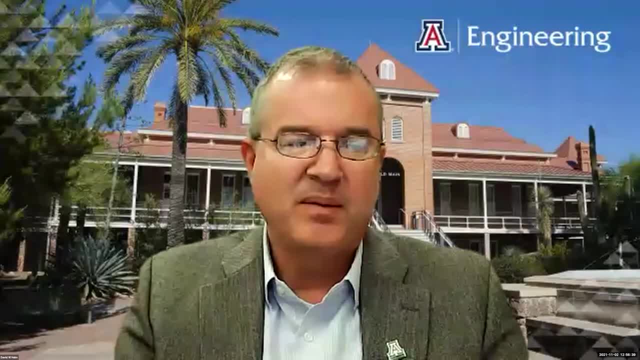 And maybe what might the next challenges be. I'll go to you, Judith, and you, Jung-Yul, So I think that you know, I think, where this is headed is really. I think that you know, I think where this is headed is really. 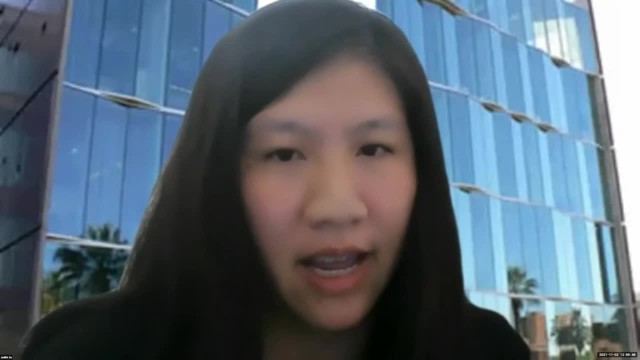 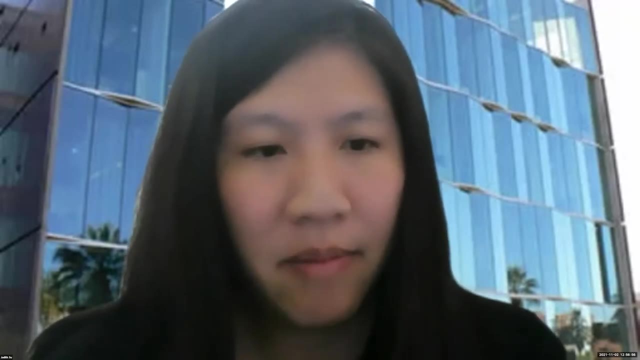 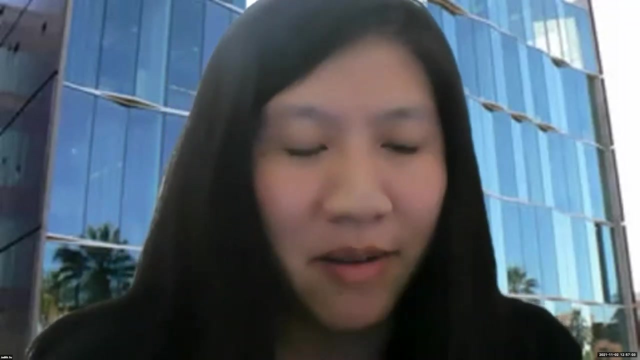 Personalized, you know, point of care Sensors. So I think you have this increasingly aging population increasingly wanting to be more educated about their health outcomes, So I think you're going to see lots of sensors integrated everywhere. So, you know, you might, you know, wake up in the morning, you know, step on your floor. your floor might have sensors to tell you about your gate and how that affects your health. 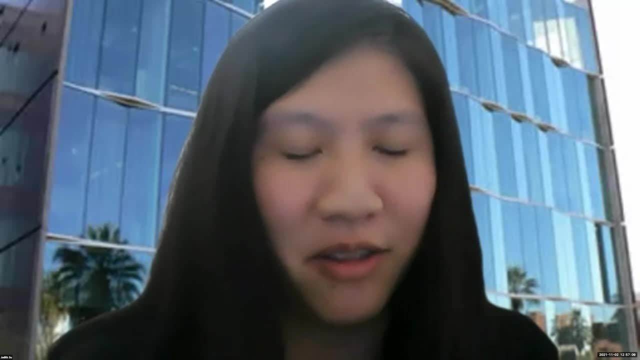 You know, you might have sensors that tell you whether you took your medication or not. you know, and you'll and everything will be, you know, personalized. You'll and everything will be, you know, personalized specifically to your biomarker levels, your baseline. 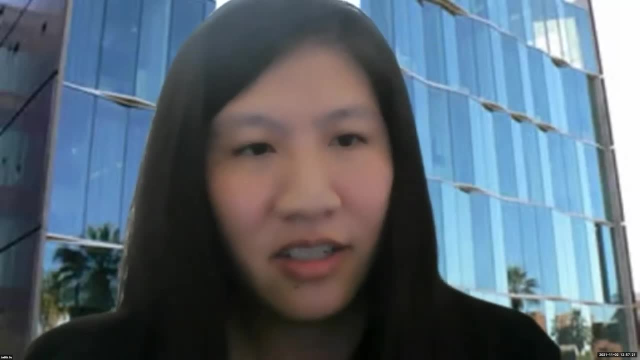 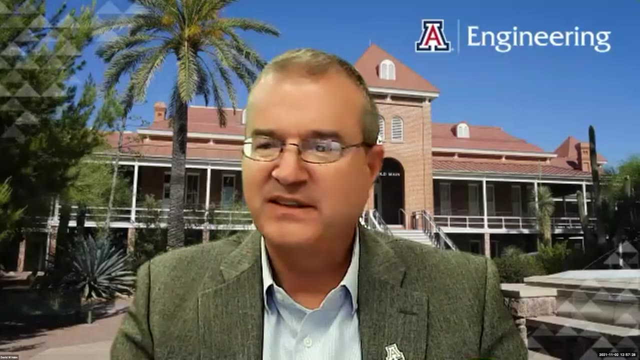 And maybe automatically sent to like physicians. So I think you're, I think it's really going to be personalized, personalized healthcare and point of care healthcare. Wow, Fascinating Jung-Yul Yep. So the the same thing goes with me. 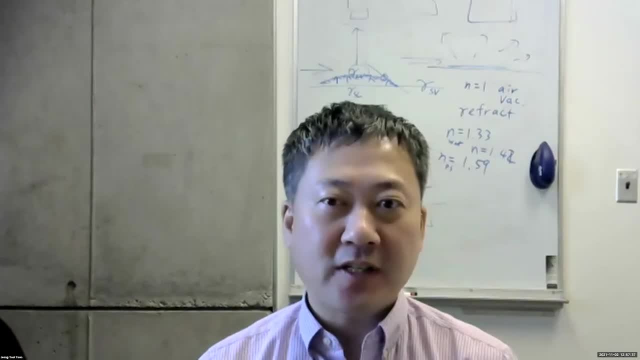 So in the future, you know the this could be a concern for primary doctors. but you know, I think we can use primary doctors over Zoom And then we can actually test them. Yeah, our own blood test, our own saliva, using the off-the-shelf sensor devices or the strips. 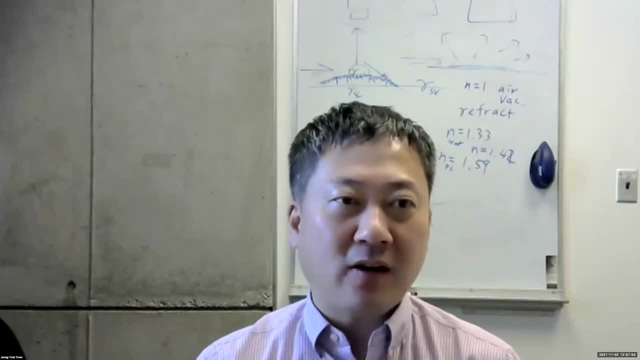 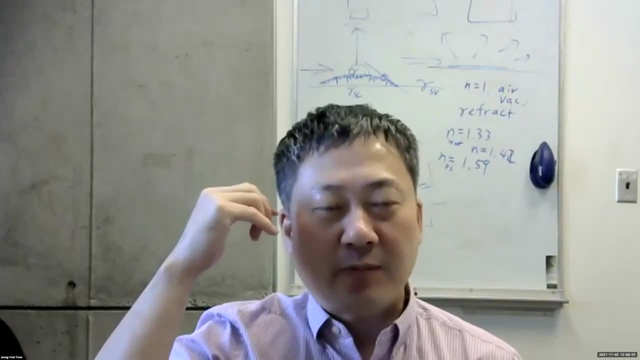 And the results can be sent to your doctor automatically in real time and the doctors can see them. So right now you need to call for an appointment with the primary doctor. you see a doctor a couple of weeks later, then you go to the lab and then you need to wait for. 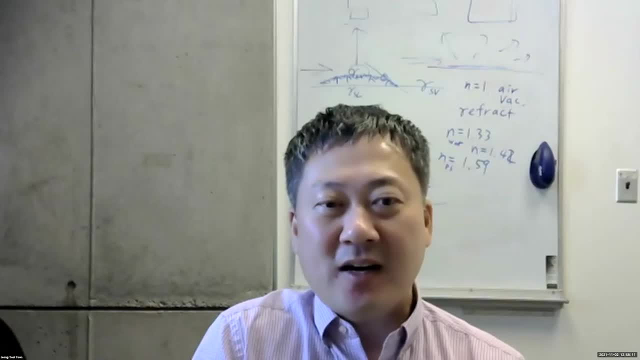 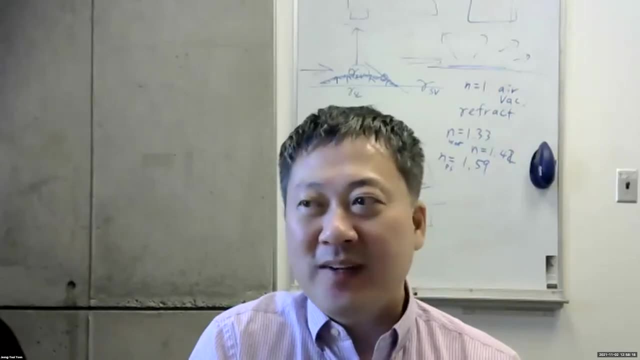 another week and a follow-up meeting. Everything can be done in a matter of just one day, And then, eventually, those primary doctors may be replaced with the AI- artificial intelligence. Wow, Yeah, that's the future that people are talking about. 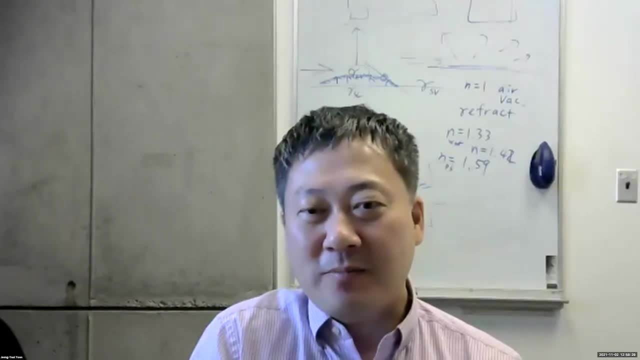 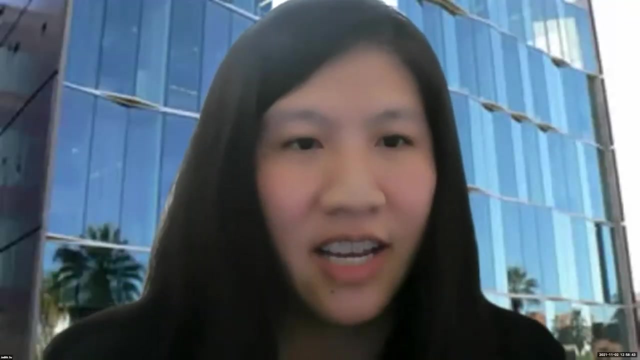 So there will be some resistance from the medical community and insurance companies, but since this is the way to save their time and save their money, I think it's going to go towards that direction, whether we like it or not. I think you're going to see this democratization of science. 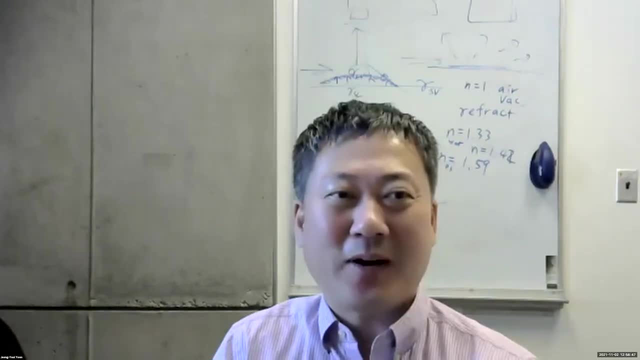 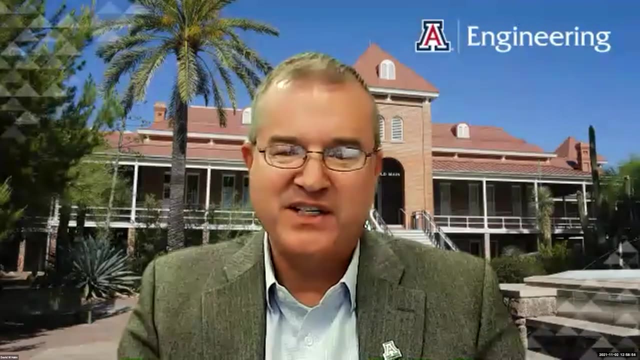 You're going to see more citizen scientists get involved? Yeah, probably That's a great vision. I want to thank both of you for a really informative, engaging discussion. I want to thank our alumni friends, colleagues in the audience that attended. 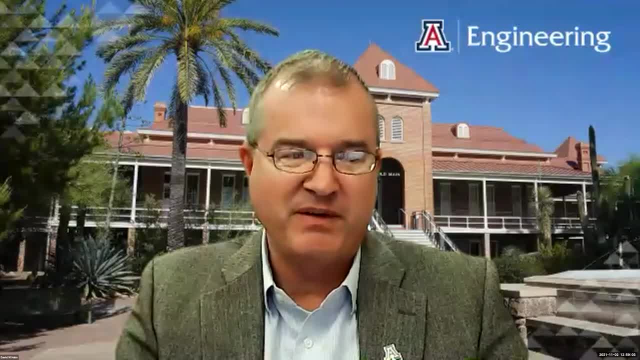 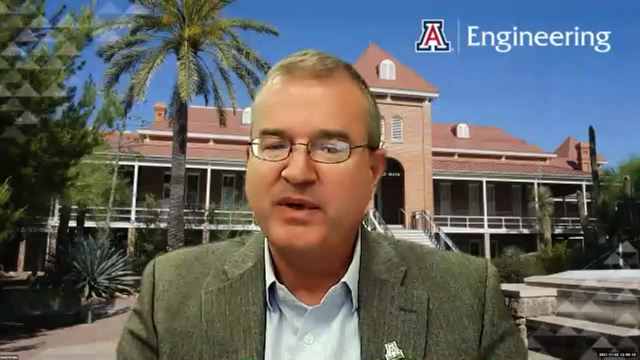 some great questions. This has been a really informative and it's been a very enjoyable afternoon, So I want to thank everyone for your attendance. I hope to see many of you Friday at the homecoming breakfast for the college or at Saturday's tailgate out on the lawn.